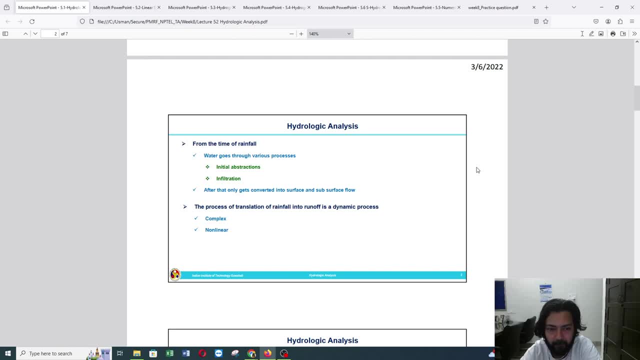 whatever water is left that is converted into subsurface flow and surface flow right After infiltration. whatever water is left that goes to subsurface flow and above the surface, whatever water is flowing, it is called a surface flow right. So what we are going to see in today's week is, more precisely, we are going to see this process of translation of rainfall into runoff. 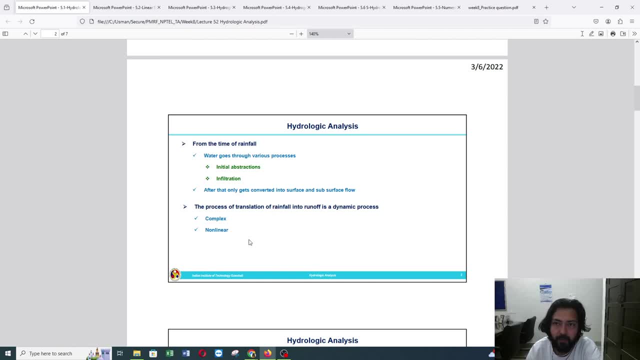 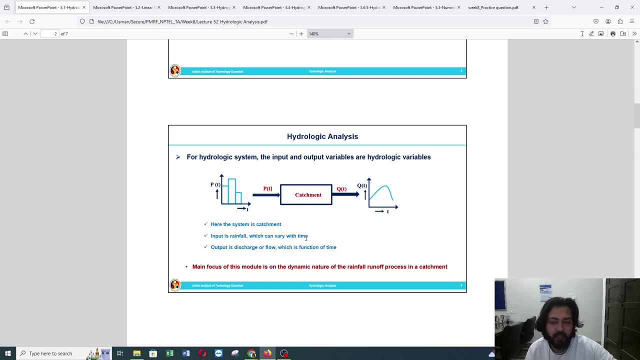 which is a dynamic process And why we are saying it is a dynamic process? Because rainfall and runoff, both are having function of time. It changes with respect to time, Right? So we are calling it as a dynamic process. So the important thing here to understand the rainfall runoff process is to understand the hydrological system concept. 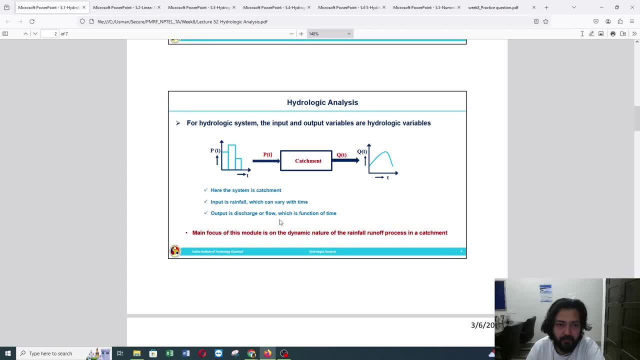 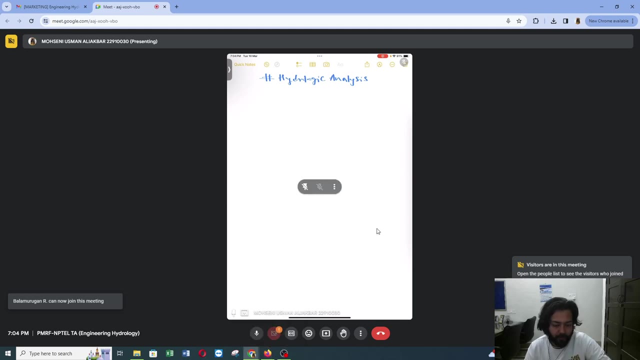 So, if you look at, if you want to talk about hydrologic system first, we should understand what is a system. So, if you want to understand a system, a system consists of three parts, right, The first part that a system consists is of is called as the input, the input to the system. 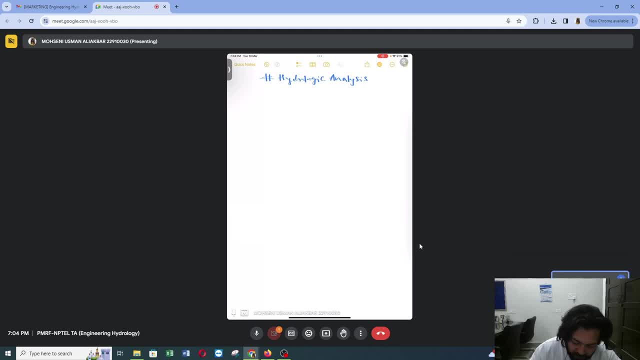 So, if you are talking about system, the first thing that we should understand is: So, if you are talking about system, the first thing we need to understand is: so, if we are talking about system, the first thing we need to understand is the system. 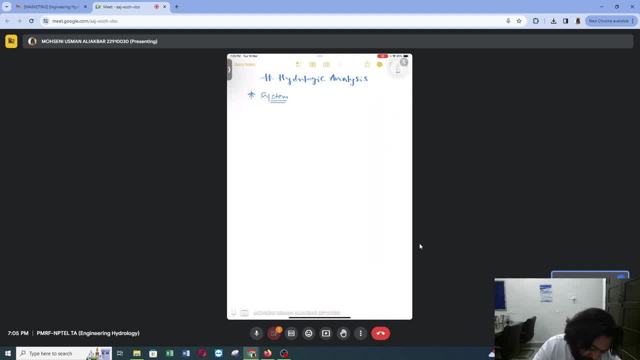 consists of three parts, and those three parts are: first is input to the system. second is we call it as a operator, on which thing the system is operating. so second part is called as operator. and the third is output from the system. so any system will comprise of this. 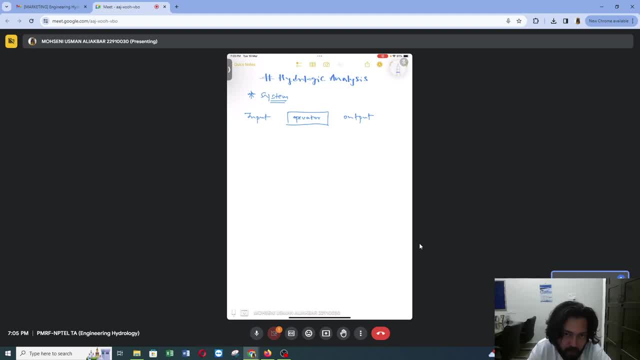 three part: input, operator and output. so, but here we are talking about hydrological system or hydrologic system. so hydrological system, so hydrological system, will also comprise of the three part, that is, input, operator and output. but here the important thing to understand is that the input and output should be a hydrological variable. so if in any system the input and 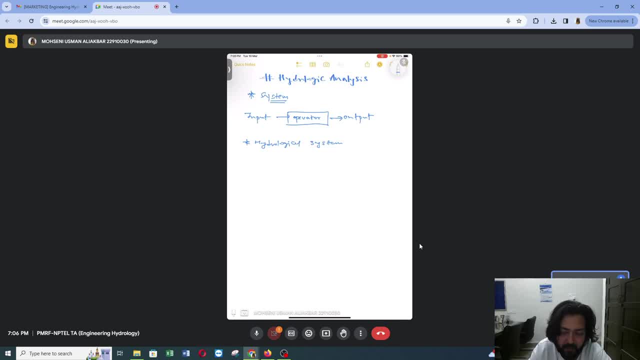 output. both are a hydrological variable. we call that system as a hydrological system. so in in, for example, we can say that the let, the input, will be rainfall, which is a hydrological variable. so this rainfall is an input to the system. here the operator would be the catchment. 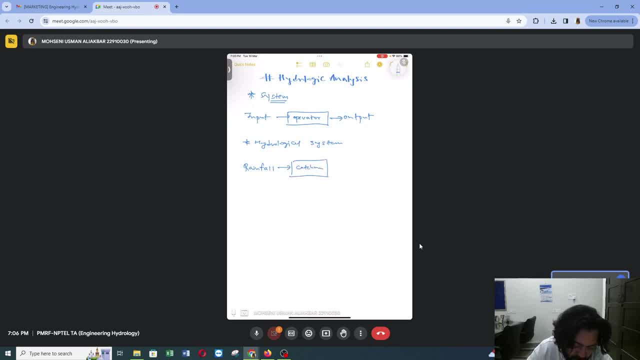 or the basin on which the rainfall is occurring right, and all the catchment will have a outlet point right. so from that outlet point what we will get is runoff. So this entire system is called it as hydrological system because the input is a hydrological. 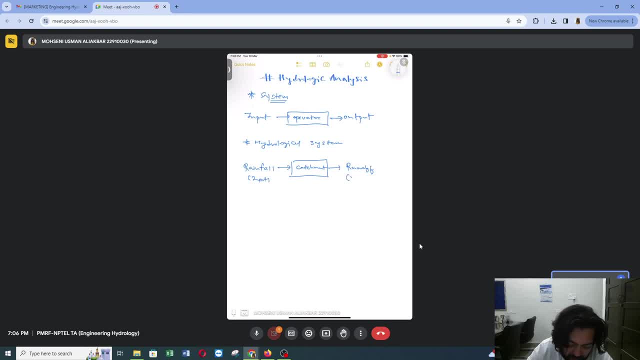 variable that is rainfall, and output is also a hydrological variable, which is runoff. so this is like the basic definition of hydrological system. now, to understand hydrological system, we need to develop the model right, and there are many models that are available right. the model can be physical model, or it can be empirical model, or it can be non-physical model, or it. 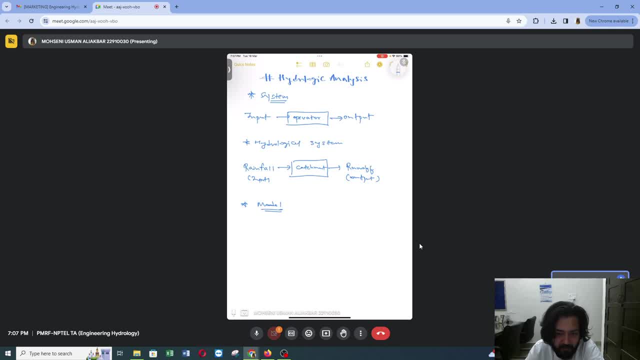 can be conceptual model. so there are various categories of model, right. so this we have covered in the very first week of the lecture of the subject, like what are different types of models that are available. so what we are going to study here is we are going to study. 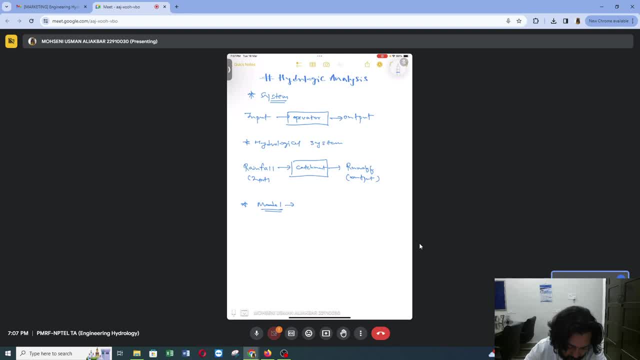 like: what are the different types of model? so we can categorize that as physical model. right, We can categorize it as empirical model or it can be conceptual model. so these are different categories of model. we know every model like what physical model has it like physical models? 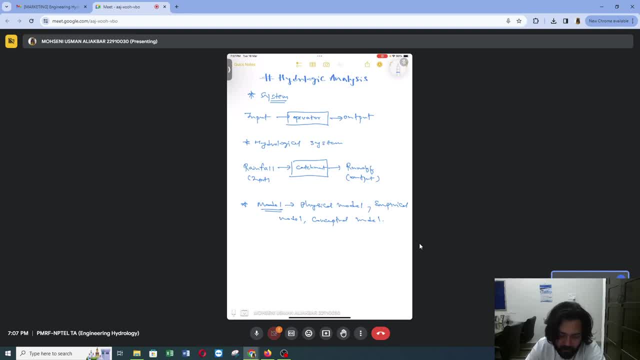 are those models which are basically run on the governing equation, right. empirical models are those model which we have which will, where we will derive a relation between the input and output variable, normalize analogue model. we know we also see the psychological modelling. dimension is 辱 at the center of all the different types of model, right? so each of theer, whatever the 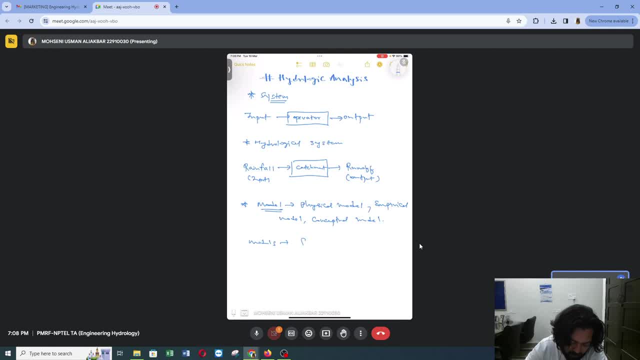 motive we were dealing about. so let us study about, like: what are the different types of hydrological or want? also, if you want to categorize the models, are those that are based on free function first. it can be categorized based on them- space- so any model can be a function. 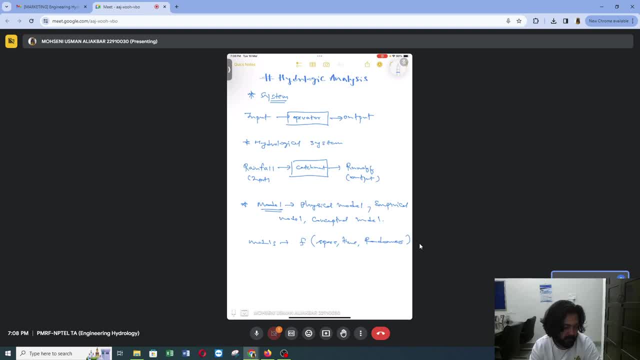 of space, or it can be a function of Randomness, right? So will limit? is this model based on three functions? Let me sort this out first. this is the window from your 0 to boil. that is. that then part based on three functions, that is, space, time and randomness. so let us take the first parameter. 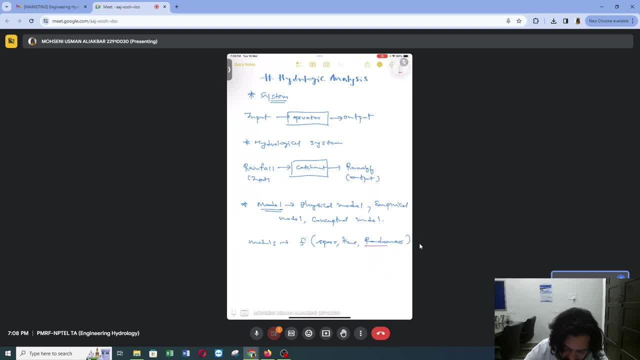 let us consider randomness. so if we are considering any model which is having a function of randomness, then we can categorize those models. as if they are function of randomness, then we can categorize those models as either deterministic models, either deterministic models or either stochastic model. so, based on the function of randomness, we can categorize the. 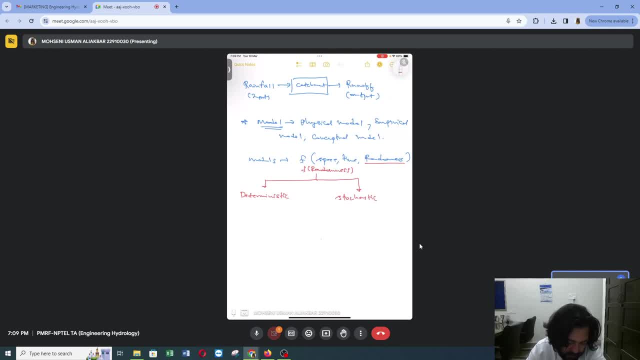 models as deterministic or stochastic. now let us see what is deterministic and stochastic. so in deterministic model we can say that it is a model which uses the law of physics, that is, the governing equations, that is, conservation of mass, conservation of momentum and conservation of energy, But at the same time it ignores the uncertainty that are present. So it will. 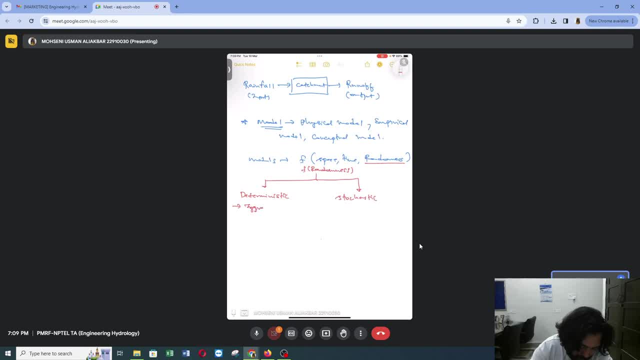 ignore the uncertainties. By this we mean that let us say we have a model which is y is equals to mx plus c, So for each input it will give a predefined output. So it is ignoring the uncertainties. But when we talk about stochastic model, there will be some. 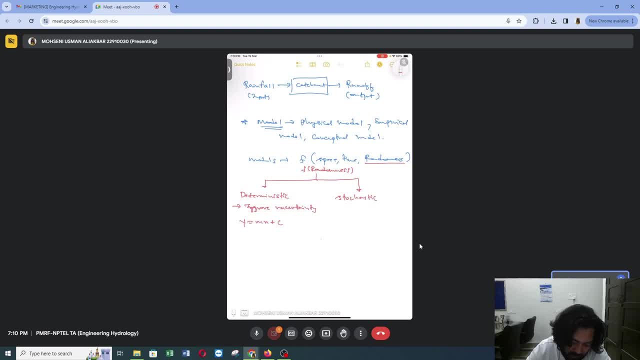 uncertainties with the output. So here they are considering the uncertainty. So we can say that the equation would be mx plus c plus some function of randomness. So here we will get the. for each output we will get each. Each input will get output. But here there will be some randomness associated with the. 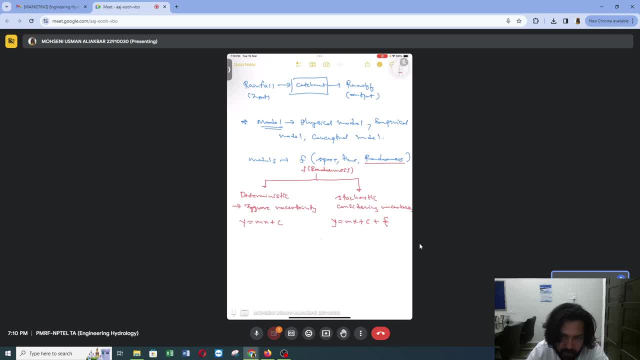 result. So this kind of models are called stochastic, This kind of models are called deterministic. They both are function of randomness. Now let us say we want to consider function with respect to same Some model, which are having function of space. So those models 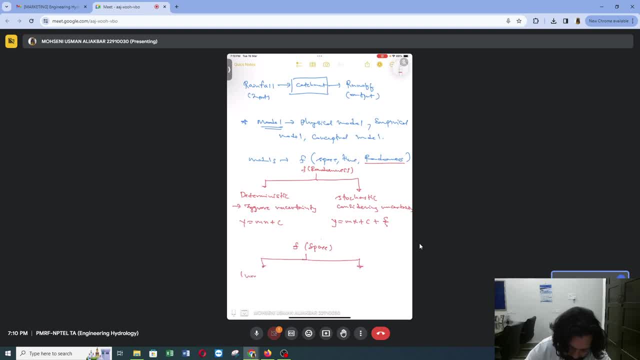 can be divided as lumped model or distributed model. From the function of space, the models can be categorized as lumped model or distributed model. So now let us say, like, what does lumped model do and what does distributed model do? So lumped means they are ignoring the spatial variation. So they are ignoring the spatial. 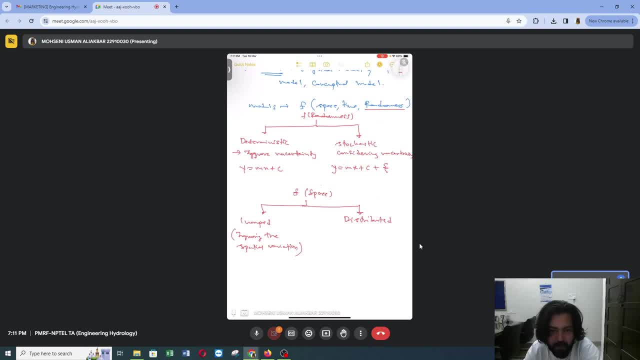 variation. So what does it mean by ignoring the spatial variation? Let us say we have a catchment and we have rainfall data for catchment. So we have rainfall data for catchment, So we know that the rainfall is having spatial as well as temporal variation associated. 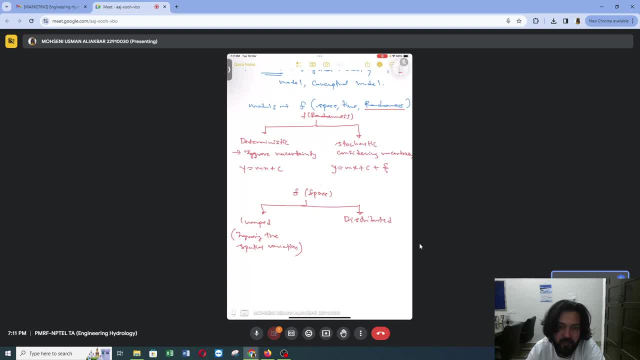 to it. But what does lumped model do? It will ignore the spatial variation. So what does it do that For the entire catchment area, it is saying that the rainfall is constant throughout the catchment, which cannot be true, So it is ignoring the spatial variation. 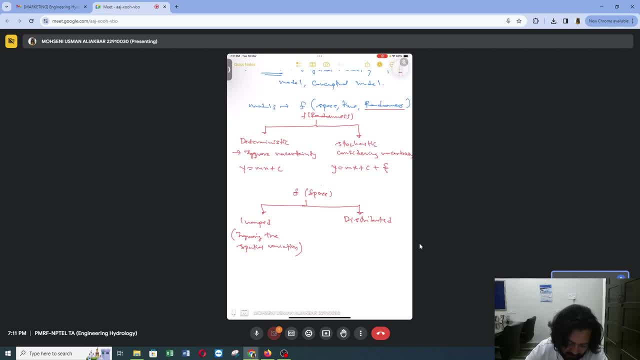 So lumped model is ignoring that spatial variation in the data set, Whereas distributed model it considers the spatial variation. So lumped model is ignoring that spatial variation. So based on randomness, we can divide a model. Classified model is deterministic. 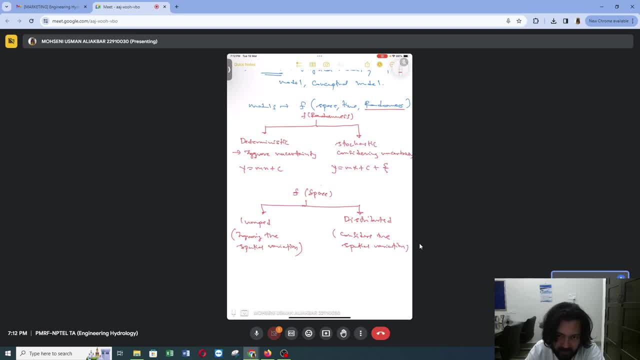 or stochastic. Based on function of space, we can categorize them as lumped and distributed. Now, the last is based on the function of time. So, based on the function of time, we can categorize the model as steady model or unsteady model. 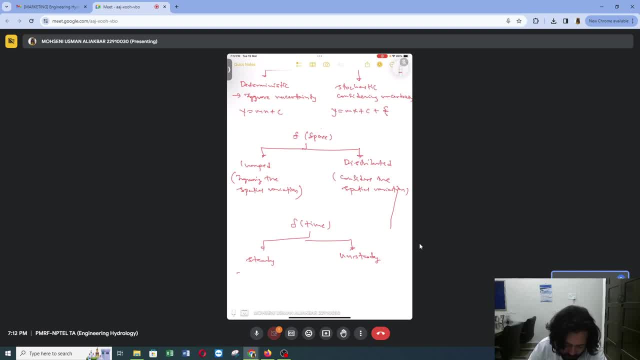 So by steady model we know that it ignores the variation with respect to time. It means the parameter will not change with respect to time. So that is what we mean by steady And by unsteady means it considers variation or it varies with respect to time. So we 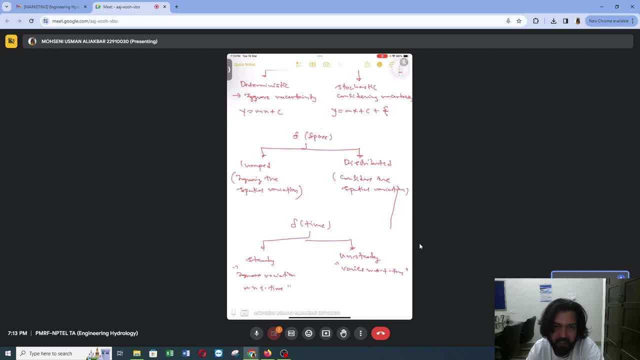 know that it ignores the variation with respect to time. So, based on these three functions, we can categorize the model as deterministic or stochastic. based on randomness associated. Now, based on the function of space, we can categorize the model as lumped or distributed. 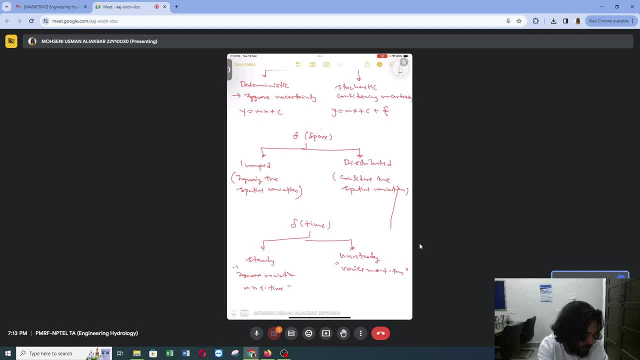 And, based on the function of time, we can categorize them as steady or unsteady model. Now that we have classified and we understood what are the different types of model, now the important thing here to realize is that to understand the function of time, we can. 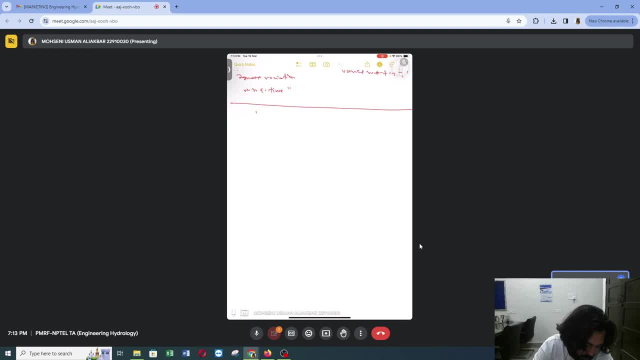 categorize the model as steady or unsteady model. Now, the important thing here to realize, that is, we should talk about more about the transfer function, or we call it as operator. now, this rainforest of process is based on linear system, right, so by linear system means. 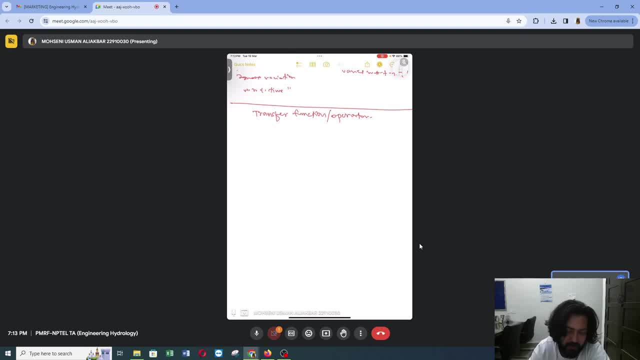 we should consider the linearity in the transfer or function operator. so let us say we are considering this first function as constant, so we are keeping the transfer function as constant transfer function. so what does this mean by constant transfer function? so by constant transfer function we mean that there is some relation between input and output of the data. 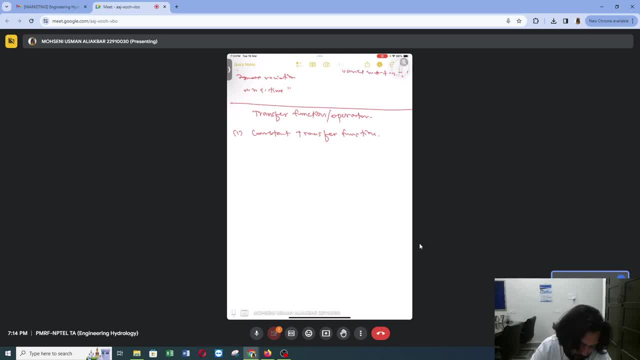 so we can say that C times of input, which is the function of t, is equals to Q of t, right? so from here we can get the constant transfer function as qt by i of t. So if you want to look at the graph also, we can say that this is the inflow, this is the outflow and there is a. 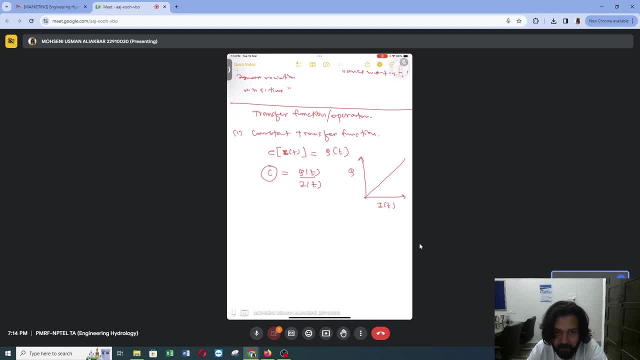 linear relationship which is given by c. But this is not the case. always, right, There could be some relation. we call it as differential transfer function. We call it as differential transfer function. So by differential transfer function, what do we mean by that? We know. 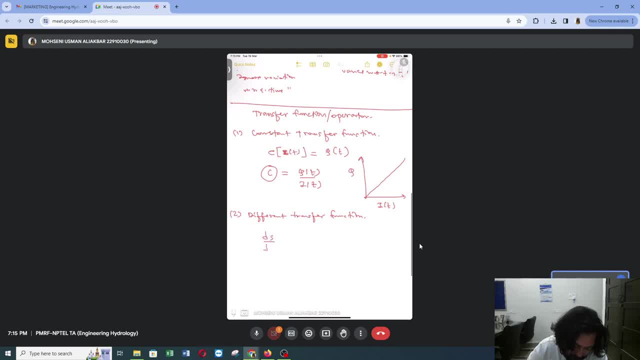 that the continuity equation is nothing but ds by dt is equals to qt minus it, right? So this is the continuity equation that we know. But also we know that the storage that is is a function of outflow. So storage is a function of outflow. So if we differentiate this with respect to time, 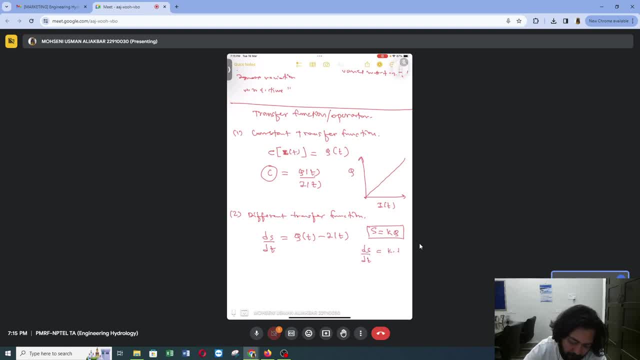 we will get an equation of ds by dt is equals to k dq by dt. Let us say this equation is 1.. And also we can also write this as inflow minus outflow. So now what we are going to do: We are going to substitute this equation 1 in equation 2.. So what we will get is kdq. 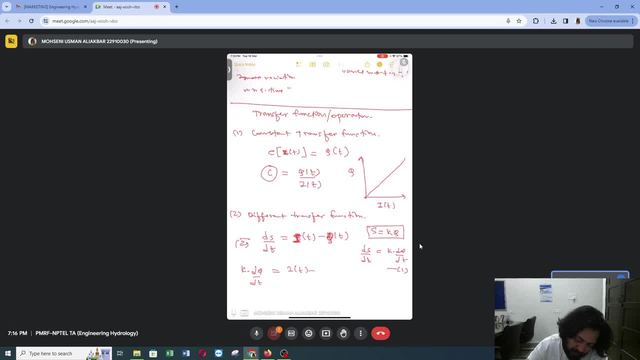 by dt. So what we are going to get is: kdq by dt is equals to i of t minus q of t. right Now we will keep the discharge term, that is, the outlet term, on the same side. So dq by dt. 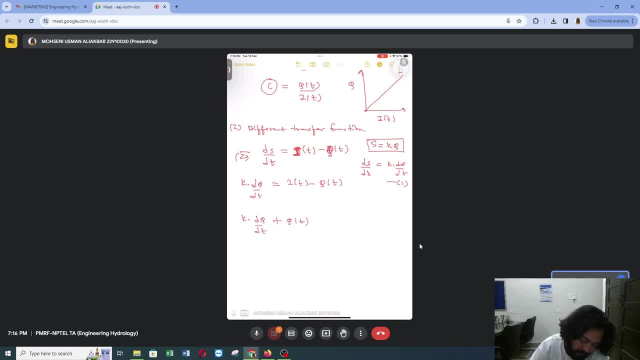 plus q of t is equals to it. right Now, what we can do is we can write capital: D is equals to d of dt, So so this term will become q of dq plus q plus q of t equals to i t. So, if you want, 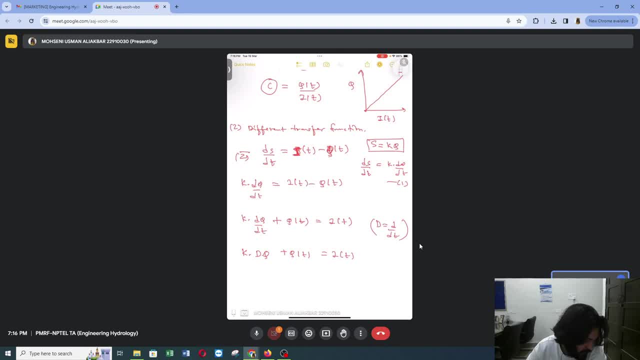 to again modify this equation. what we can do. We can take kd plus 1 into qt. equals to i, t And from here we can get kd. so I am writing dp. I can say: if you want to modify and substitute this by dt, I will write by dt. so we will only need a partial of dq per. 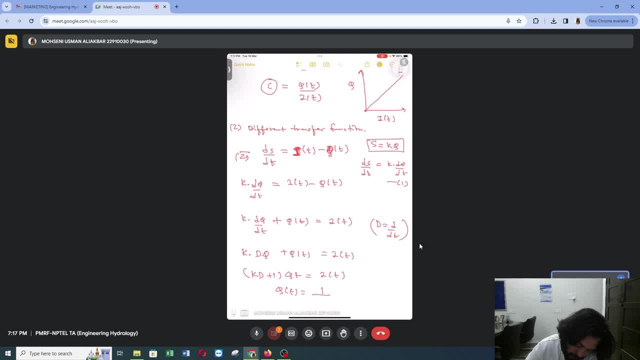 dq. Now, if I substitute this equation enter to zero, then what I will get is again: the q t is equals to 1 upon k d plus 1 of i t. right, So from here we can say that this term, which is nothing, but it is a differential transfer function, which is a differential 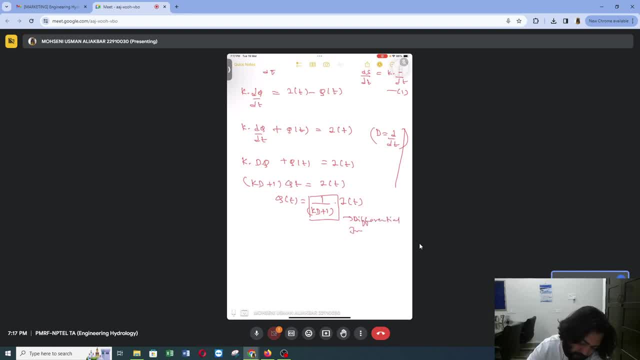 transfer function right. So the relationship between outflow and inflow can be due to a constant transfer function or it could be due to a differential transfer function. So from this we can say that the output and input is, or the rainfall runoff model is a linear. 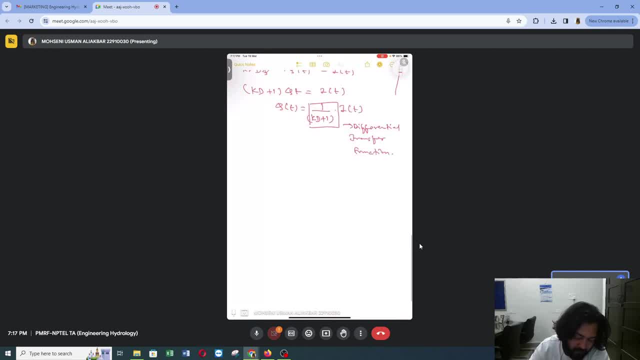 system. Now, what does? how does a linear system work? So the next thing that we should understand is that: how does a linear system work? So the next thing that we should understand is: how does a linear system would work? So let us see here: like what is, what are the? 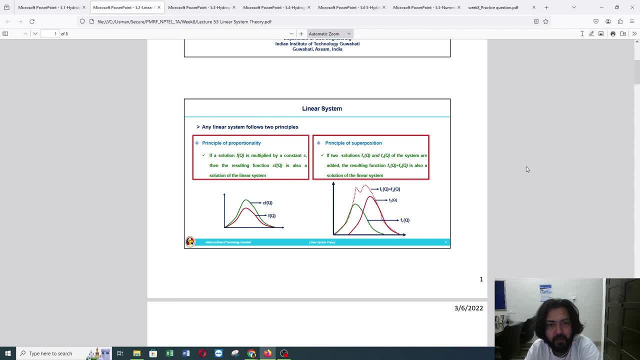 two principle on which the linear system is working. So the linear system is based basically on two principle. So the first principle is principle of proportionality and the second principle is principle of superposition. Now let us understand: like what is? what is the? 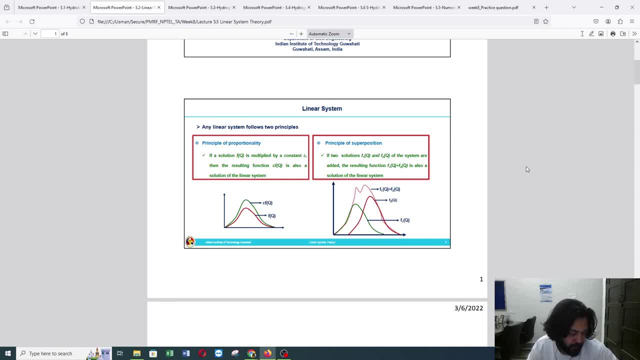 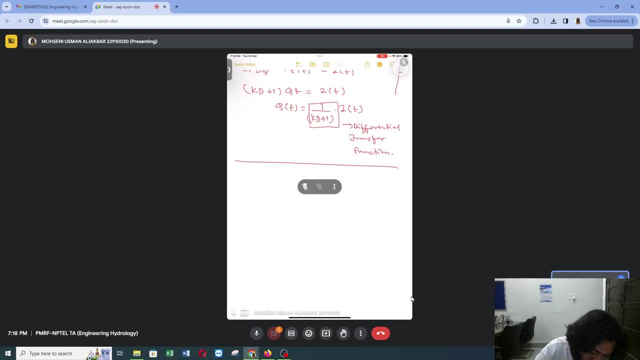 principle of proportionality and what is the principle of superposition. So first we are going to understand principle of proportionality. So the principle of proportionality state that if a solution of f of q is multiplied by a constant right, So it is saying that if a solution of f of q is multiplied 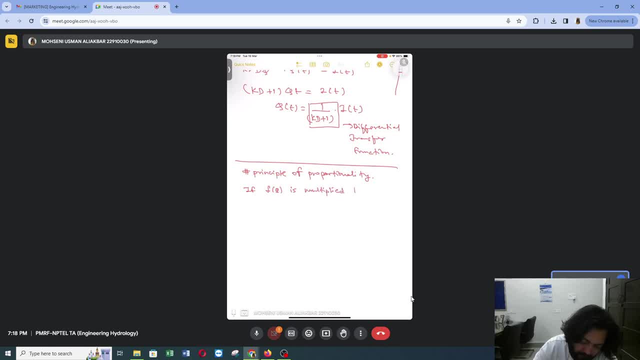 by a constant c, then resulting function, that is c times of f of q, is also a solution. So they are saying that if we have a solution let us call it as f of q, And if we are multiplying this solution with a constant c, so the next result that would be coming that is c, f of q. 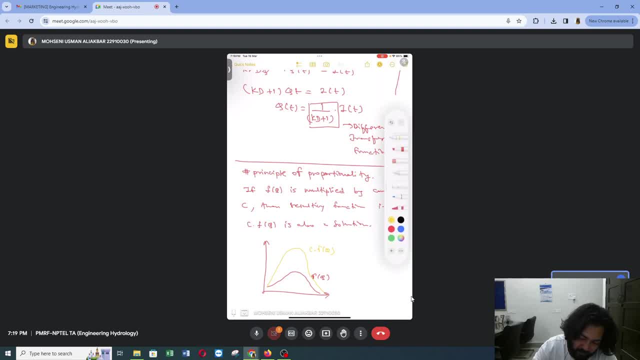 is also a solution of this. So this is what we mean by linear, of principle of proportionality. So in principle of proportionality, we are going to multiply a constant with the already defined solution and the result. So the next is principle of superposition. So this we have also studied before. But 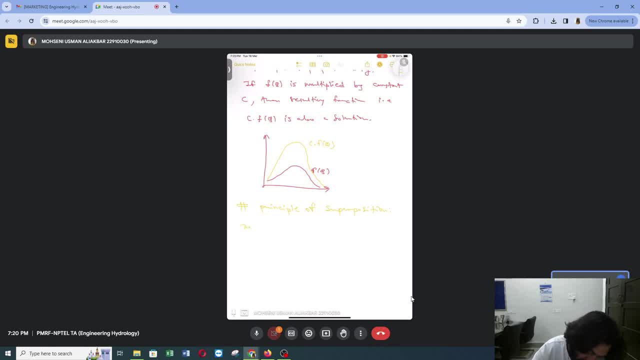 what does the principle of superposition means? Let us say: if we have two solutions, Let us say f of q, Then f1 of q and f2 of q, Then the resulting solution which is obtained by taking summation of these two solutions. 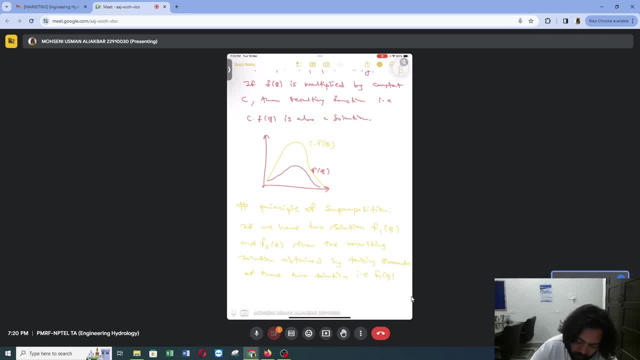 that is f1q plus f2 of q is also a solution. So in principle of proportionality, we multiply the solution which we already have. we are multiplying a proportionality constant to that. in principle of superposition, Whatever solution- 2 solution we have- we are taking. 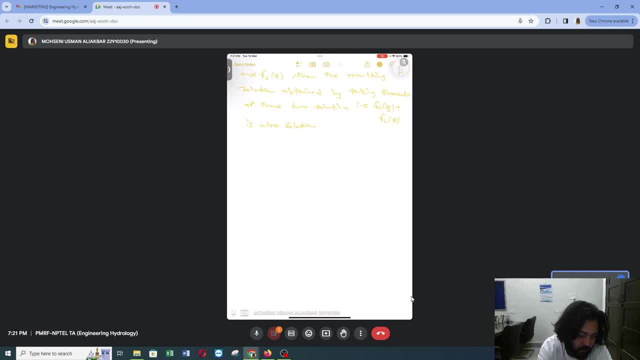 the summation of it and the resulting function, which is a summation of the predefined 2 function, is also a solution. So if we have 2 solutions, let us say we have a solution f1 of q, we have a solution f2 of q. So if we take a summation of these 2 solutions, so the answer 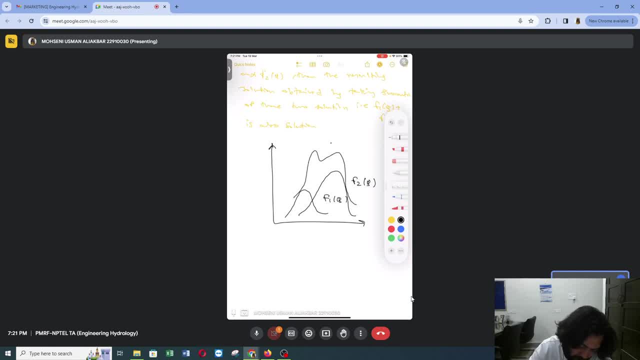 would be something like this. So this solution, which is summation of f1 of q plus f2 of q, is also a solution. So this is nothing but principle of superposition. So linear system is based on these 2 principles. 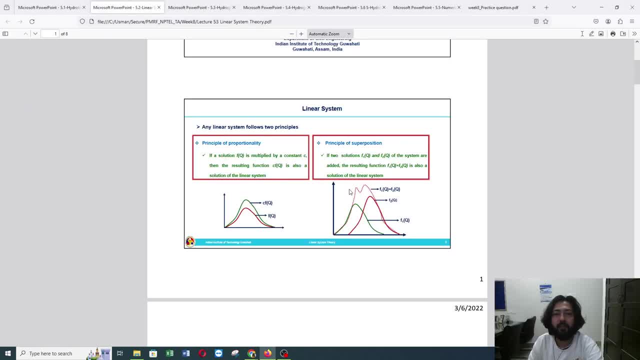 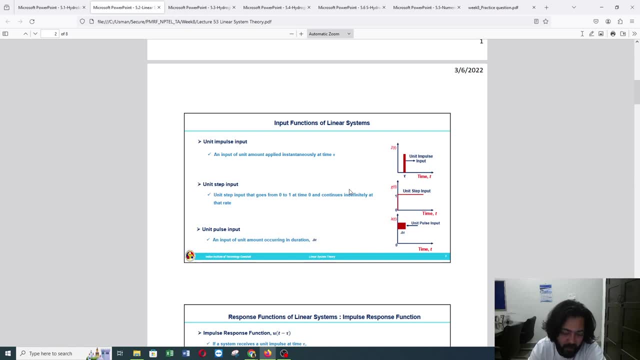 that is, linear principle of proportionality and principle of superposition. Now let us understand what are the input of linear system. So the input function of a linear system are there are 3 type of input function. So the first input function is: 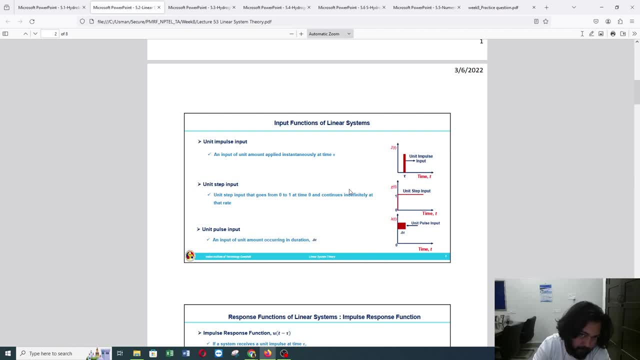 input functions of linear system. So there are 3 input function of a linear system. The first is called as input impulse input, unit impulse input. So unit impulse input means that there is a unit impulse input which is applied instantaneously at any time t. So 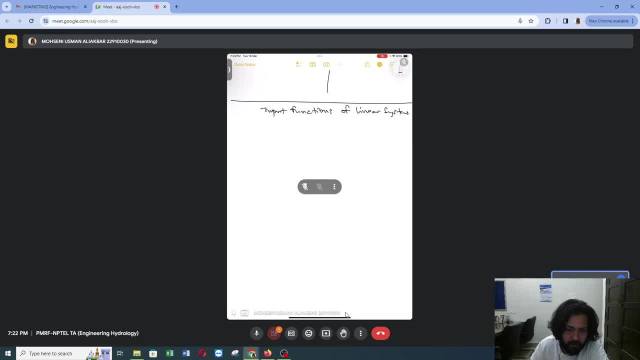 it is applied at any instantaneous time. So let us say the first type of input we have is called as unit impulse. So unit impulse means an input of unit amount applied instantaneously at any given time. t So the first input function. 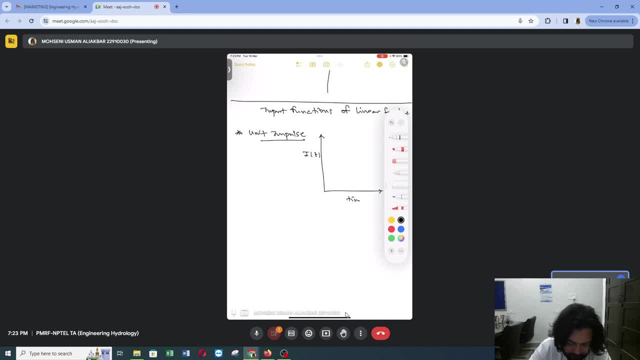 So this is input with respect to time. This is time given by tau. So an input impulse mean at any instantaneously, at any instantaneous time we apply a unit impulse, So there is a unit impulse right. This is a unit impulse which is applied instantaneously at any given. 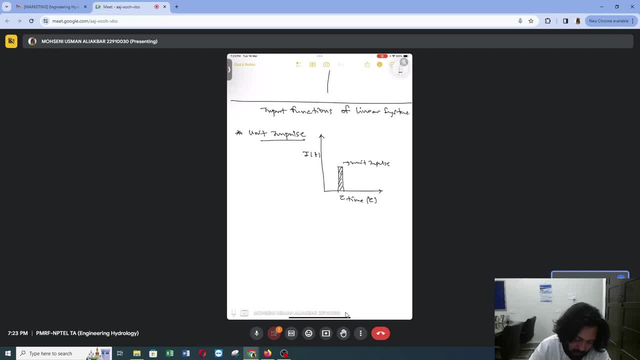 time tau. So this is unit impulse. Then there is something called as unit step. So if you want to understand unit step, this is time tau, this is input of t. So the unit step is that input that goes from 0 to 1, at time equals to 0 and then it remains constant. 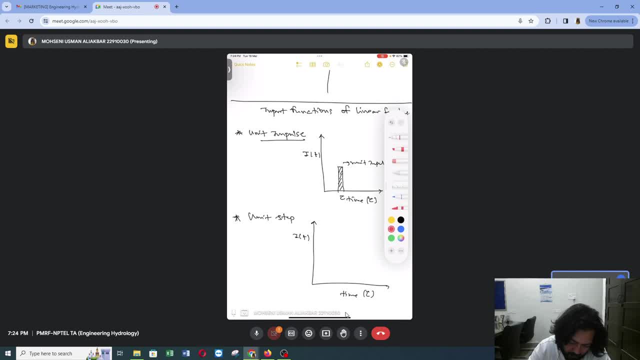 So it is saying that. So it goes from 0, when time is 0,, it goes from 0 to 1.. Let us say it is 1. So it will go from 0 to 1, and then it will remain constant indefinitely. So it will remain constant. 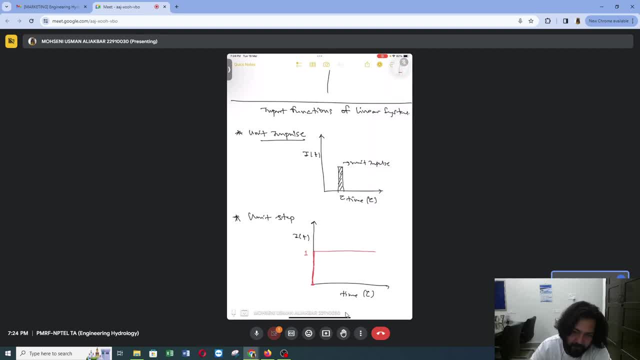 So this is nothing. but this kind of input function is called as unit step, So it goes from 0 to 1 when time is 0, and then it remains constant over indefinite time. And the last is we call it as unit pulse. So unit pulse is same as unit impulse, but unit impulse is applied at any 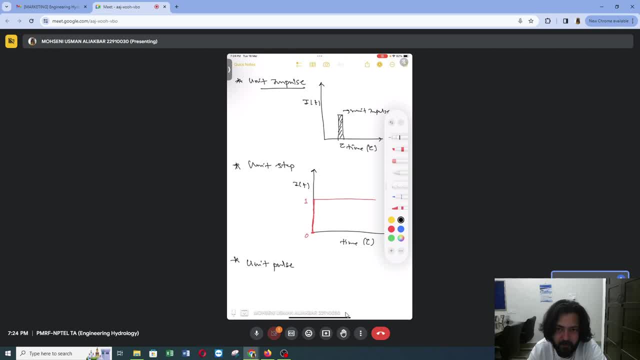 instantaneous time, whereas unit pulse is defined for a is applied for a predefined time. Let us say that time is delta t. So if you applied a unit pulse over a period of time, we call it as unit pulse. If we applied it at instantaneously, at any given time, we call it as impulse. So difference between impulse and pulse is that impulse is applied instantaneously, whereas pulse is applied for a given period of time. So let us say: this is time tau. So here we can say that we have applied a pulse for a period of time of delta t. 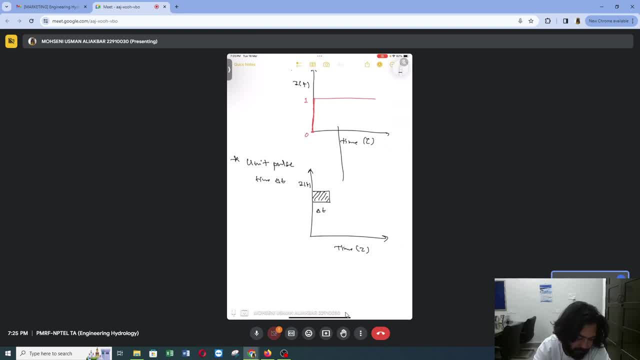 So we call this input as unit pulse. Now there is something called as response function of linear system. So this is the input function. So previously we have studied that a system will consist of three parts, That is, input, transfer, function and output. 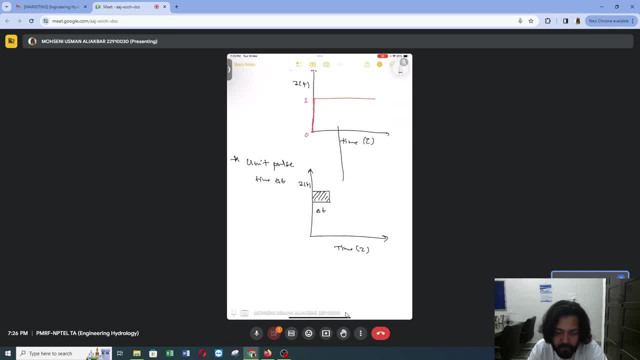 So here we are talking about a linear system. So the linear system will also have three parts. The first part is input. So first we have talked about input function. So the input function of a given linear system is of three types. 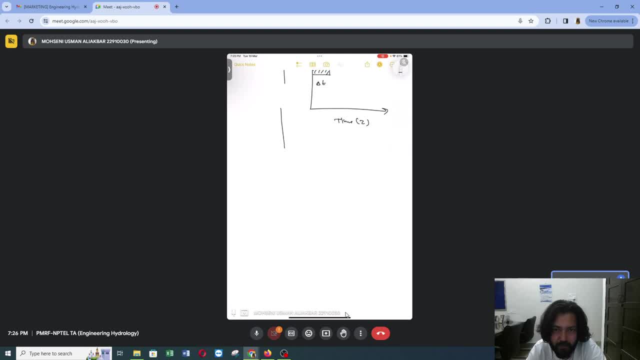 The first is impulse, unit impulse, Second is unit step and third is unit pulse. So these are the input function of a linear system. Now what we are going to talk about is the transfer function, So we call it as response function. 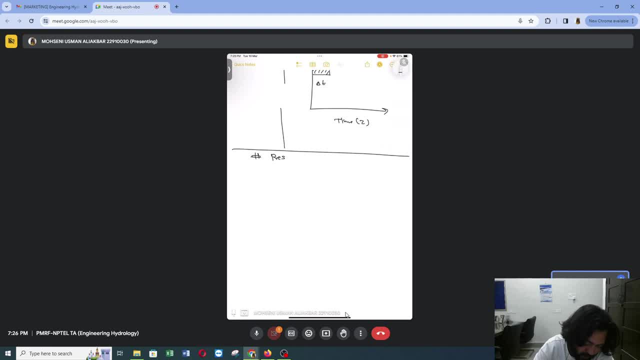 So here we are going to talk about response function. So how do we call it? So here we are going to talk about response function of linear system. So, similarly, based on the type of input, the response function will be of different type. 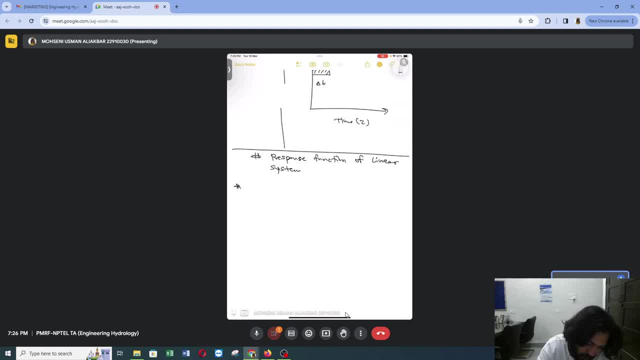 So first we talk about impulse response function. So first we are going to talk about impulse response function. So here we are going to talk about impulse response function, response function. So imposed response function is nothing but u times of t minus tau. Now 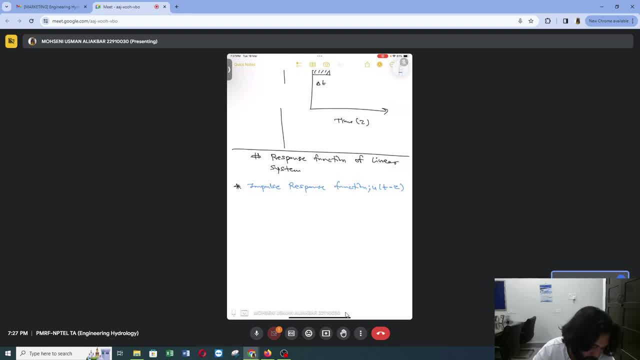 let us say what is u times of t minus tau. So if a system receives a unit pulse of t is a unit pulse at time tau, then the response of the system will be a later time t. This means that whenever we have a unit pulse as a input function in any system, the response 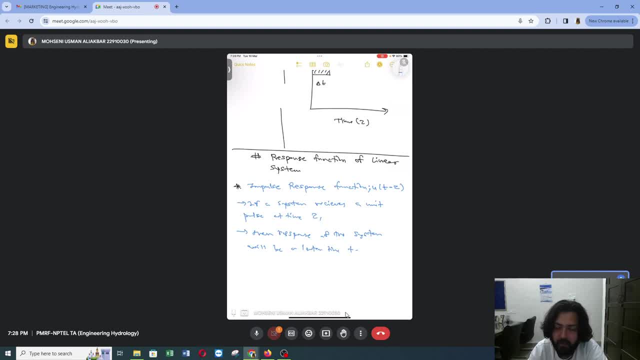 system at a given time, then the response of the system will be after a time t. it means there is some time lag between the response, so that time lag is given by that. time lag is defined by or given by t minus tau, right. so if you want to understand this, you can. 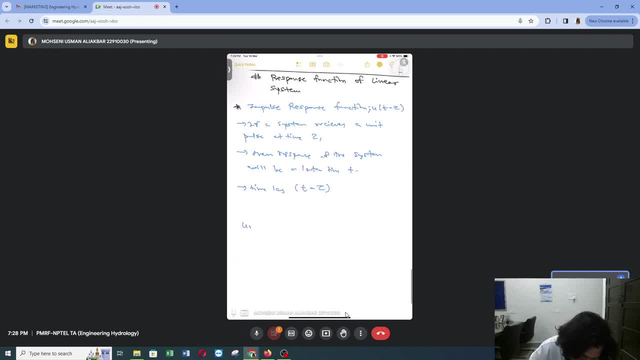 understand this by a representation also. we have a input which is unit impulse, right? so unit impulse is the input, right, then the operator is the system and the output is nothing but u times of t minus tau, right? we can also look at this graphically also. so initially we have a input. 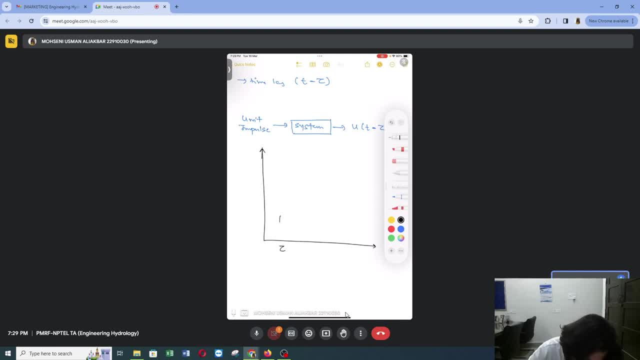 unit input at any at a given time, tau. so we have a unit impulse, right. so here u is equal to one at any given time, tau, right. so for this input there would be some output, and that output is given by response function, right, and that response function is right, and that function is nothing but u times of t minus t minus tau, right. and 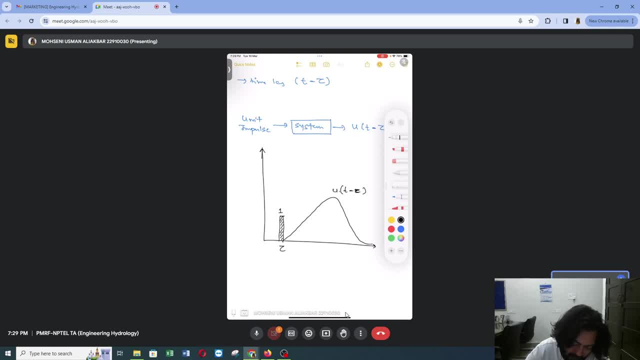 t minus tau. So there is some time lag. So we can say that this is, it is, the output is starting after time tau. So here we can say that this is now, if we apply a principle of proportionality and principle of superposition to the same system, we can, we can apply principle. 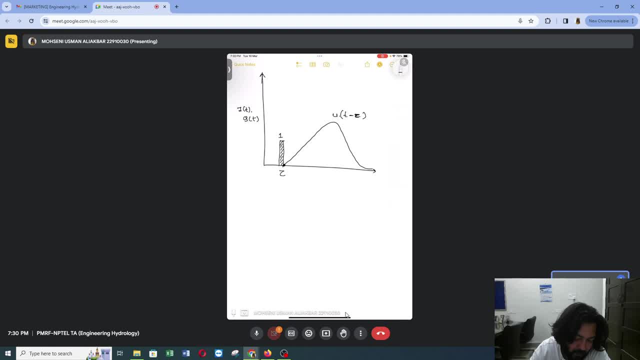 of proportionality. So first what we are going to do: we are going to apply principle of proportionality. So by principle of proportionality means we have to multiply the input impulse with some constant value. Let us say that constant value is 3.. So what we are going 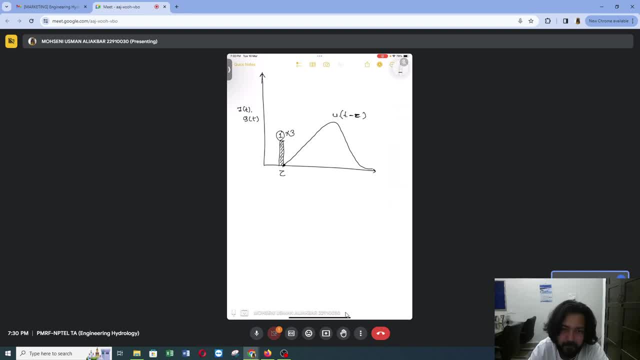 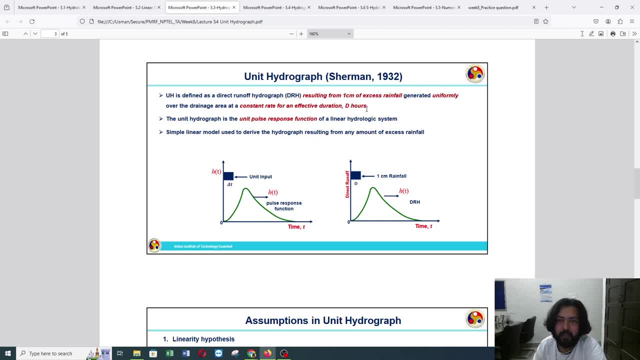 Right, So for this 3, we are going to apply principle of superposition to it. right? So for this 3, we are going to apply principle of superposition to it. Very nice, well done, Alright, Ok. so so just the first 2 things. now come to Power Principles of individuals. 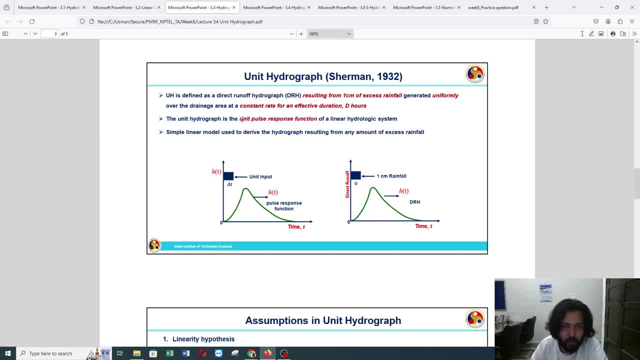 and individuals First. they are separate variables, so we should constantly pay attention to block work. Okay, so we know what is unit pulse response function now. so this figure we have studied previously also so unit impulse. unit pulse means there is a unit input over a period of time, right? 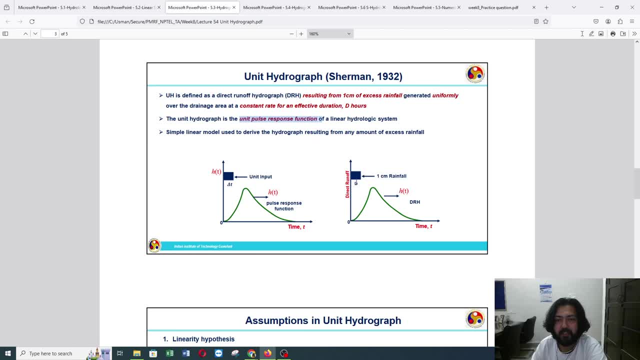 so this, for a unit hydrograph, is nothing but one centimeter of excess rainfall. so we can compare this two figures and we can understand that for a unit pulse response function of a linear hydrahoic system, the unit input is a unit pulse for a period of time right. 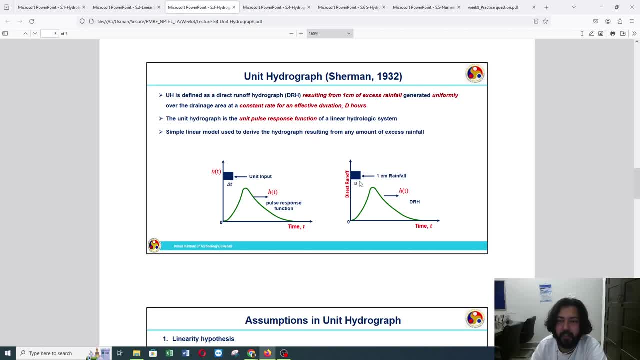 so the same thing for unit hydrograph is one centimeter of rainfall over a time period of d right and the output is a pulse response function. but here the output is d? rh right. so input is an excess rainfall for a unit hydrograph and output is a direct run of hydrograph. 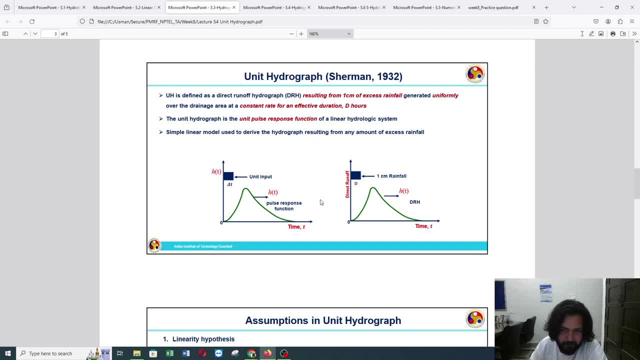 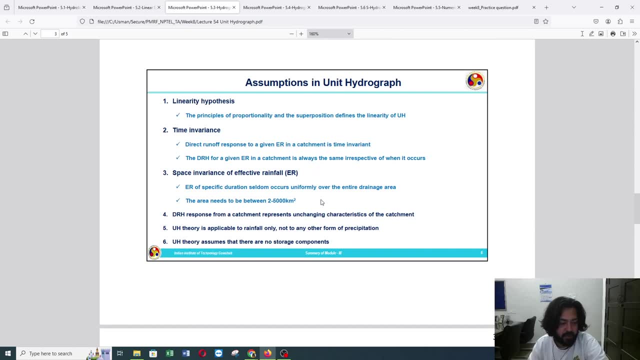 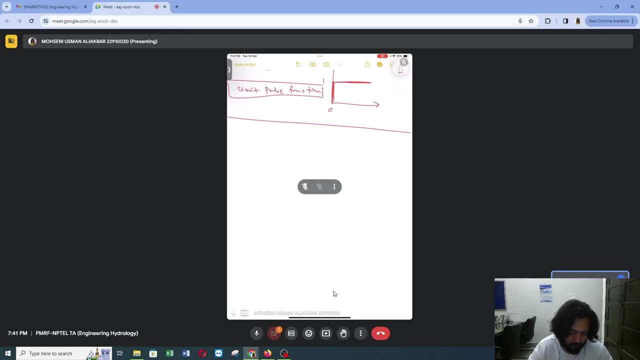 which is nothing but one centimeter pulse response function. Now there are some assumptions that are associated with unit hydrograph. So let us see, like what are the assumptions that are associated with unit hydrograph? The assumptions of unit hydrograph. So the first assumption is that the system 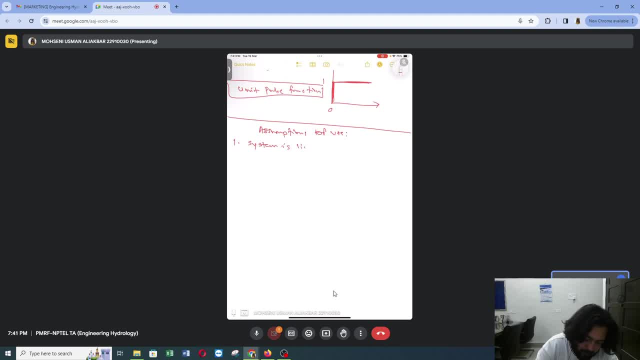 is linear. The second assumption associated is the system is time invariant. So by time invariant means it does not change with respect to time. The second is: effective rainfall is uniform over catchment. This is the third assumption. The fourth assumption is that 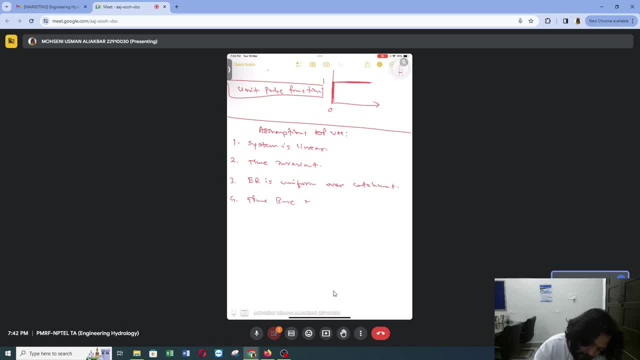 the time base remains constant. So peak might change, but the time base will remain constant. And the last assumption is that the area of the catchment should be between 2000-5000 km square. So these are the assumptions that are associated with unit hydrograph, The system. 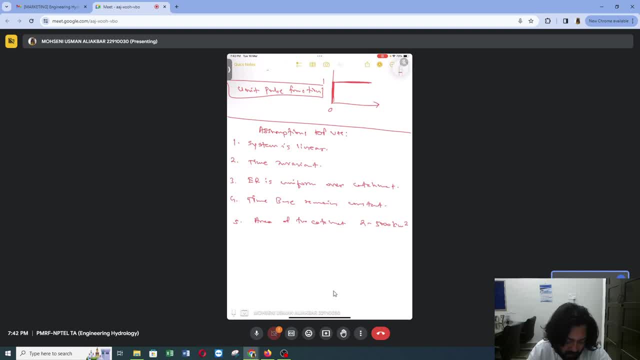 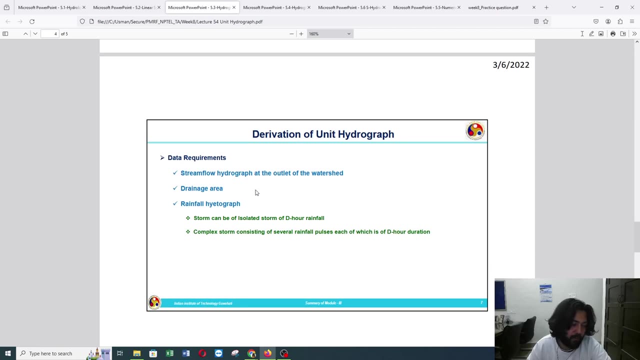 system is linear, it is time invariant, the effective rainfall is uniform over catchment, the time base remains constant and the area of catchment should be between 2 to 5000 kilometer square. Now let us see like how to derive a unit hydrograph. So the three important: 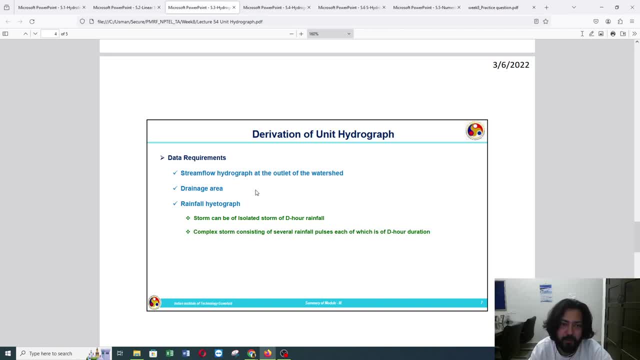 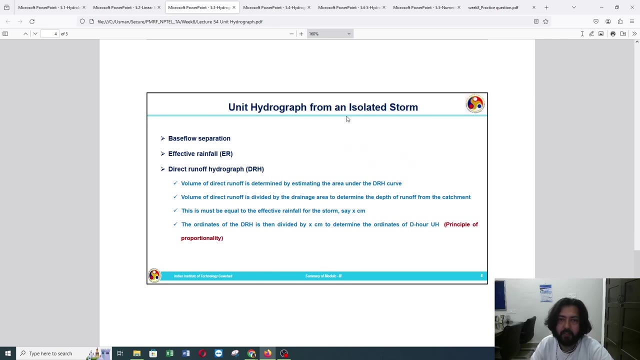 thing that you need in order to derive a unit hydrograph is: the first is the steam flow hydrograph at the outlet, the drainage area of the catchment and the rainfall hydrograph. that is the input. Now, this is nothing but a unit hydrograph that is derived from a isolated 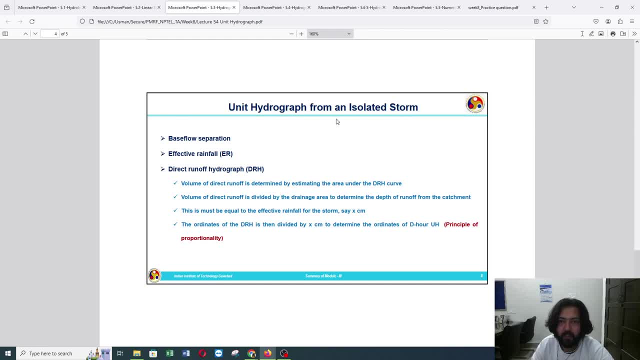 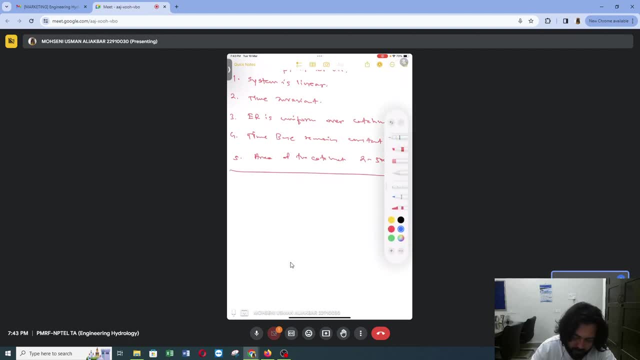 storm right. So what are the steps in order to derive a unit hydrograph from a isolated storm? We can note down the procedure for this also. It would be easier if we look at the procedure right. So we can note down the procedure for this also. 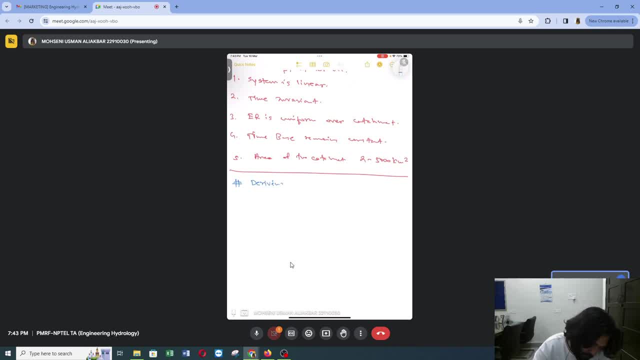 So we can note down the procedure for this also. It would be easier if we look at the procedure for this also. It would be easier if we look at the procedure for this also. So what we are doing is we are deriving a unit hydrograph from isolated or single storm. 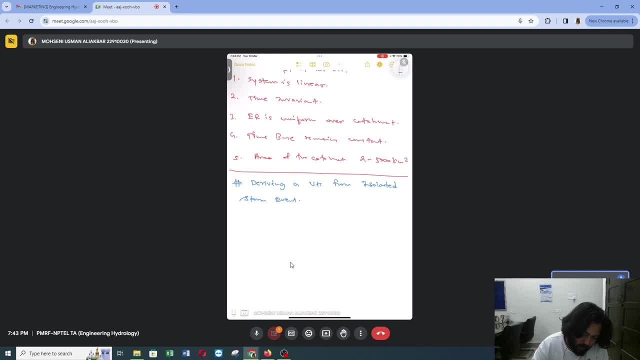 event. So what are the steps? So the first step involved is we should select a isolated storm of some duration, Like Scytler says, we should know the duration of that storm. So the first step is selecting the unit hydrograph at the outlet, at the outlet at the bottom. 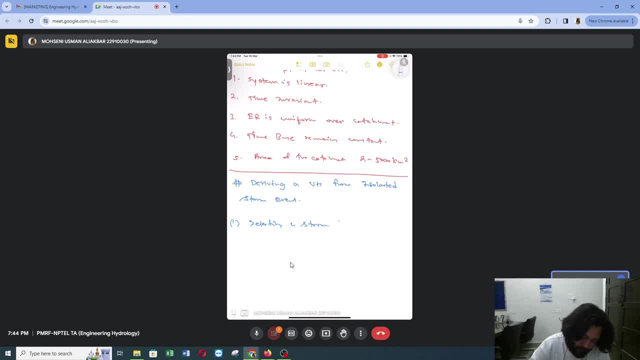 a storm, having desired duration d right. so if we have a storm and we know the duration of that storm, then we can proceed with deriving a unit hydrograph for that storm. the second part is to draw to plot q versus time, plot that is, discharge versus time, curve for that. 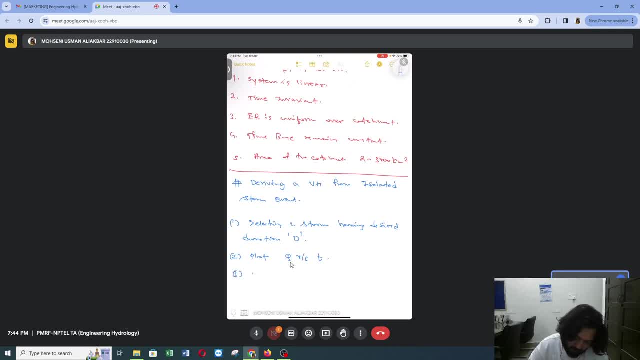 storm. the third is base separation. so what we are doing here is we are separating the base flow contribution to that runoff. so why we are doing this here? this is because in order to derive unit hydrograph, we need to know the direct runoff hydrograph. so we are. 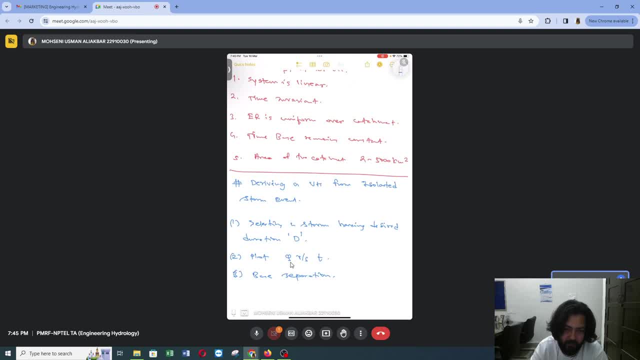 doing direct runoff value, right. so for that we need to separate the base flow. so there are different techniques in order to do that. we have discussed that in the prior class in the prior week. for base separation or base flow separation, there are technique called as straight line method and there is variable slope method- right, fixed base method. so there 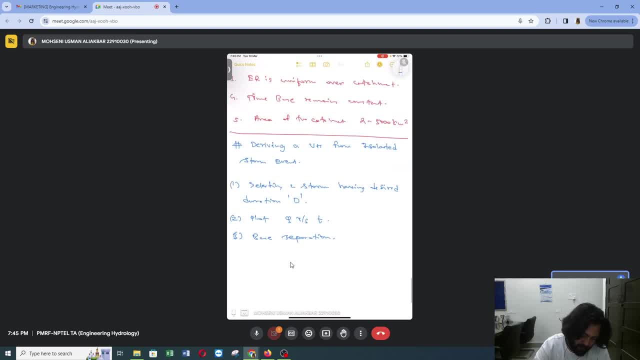 are three different techniques in order to separate the base flow from a unit hydrograph. the next step is to find the volume of drh. now that we have separated the base flow contribution into that catchment, we can calculate the volume of direct runoff hydrograph right. so how we can do that in order to calculate the volume. 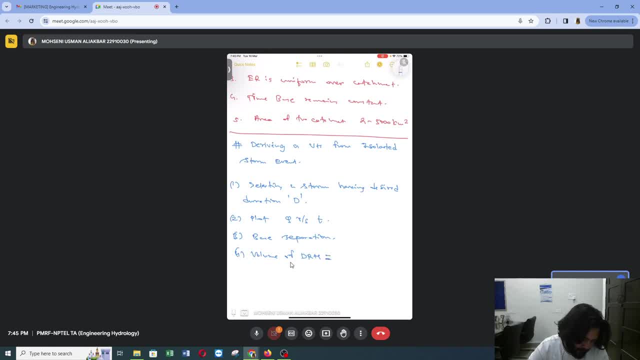 of drh, we can simply calculate the area under the curve. so if we calculate the area under the curve, we will get the volume of drh. next we can calculate is the depth of effective rainfall, and how we can do that is by dividing the volume of drh with the area of catchment. 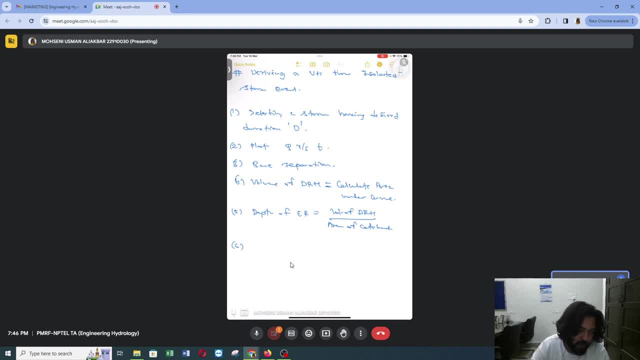 see, not that we know the depth of effective rainfall. what we can do is we can calculate the ordinate of drh, so we can calculate the ordinate of unit hydrograph. and how we can calculate it is the process of the infants of hearing. it will do so to how we can Will. 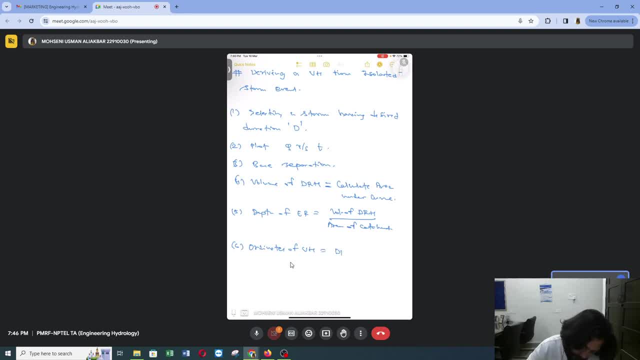 that titles bag tct a can do that by dividing drh, ordinate with depth of effective rainfall, and so these are the 6 steps that are involved in order to derive a unit hydrograph from a isolated storm event. right, isolated storm event means it is a single storm event. now let us say there: 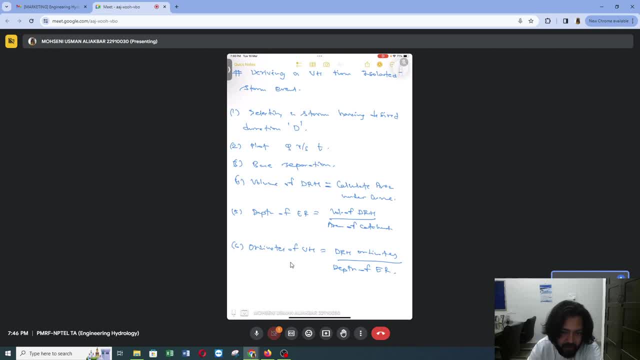 are multiple storm events, so how we can derive the ordinate of unit hydrograph. so now we are considering a case of a complex storm of duration multiple of d. so there is a standard equation which we can use in order to derive discharge for this kind of problem, which is 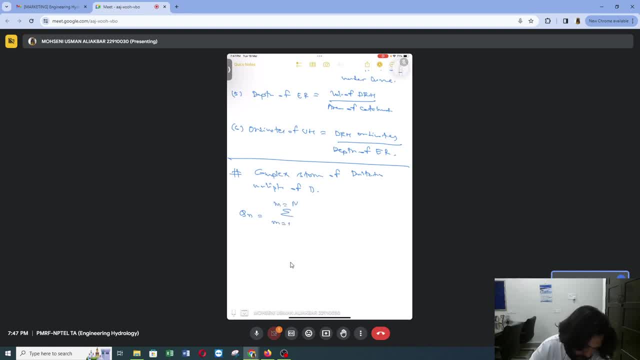 where P is. where P is, X is the rainfall depth being felt with or being observed, or qn is drh ordnates and u is unit hydrograph ordnates that is to be found. so this is the standard equation which is used in order to derive drh of, or unit hydrograph or ordnates. 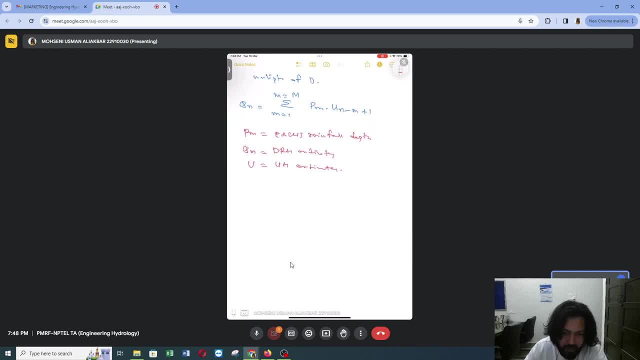 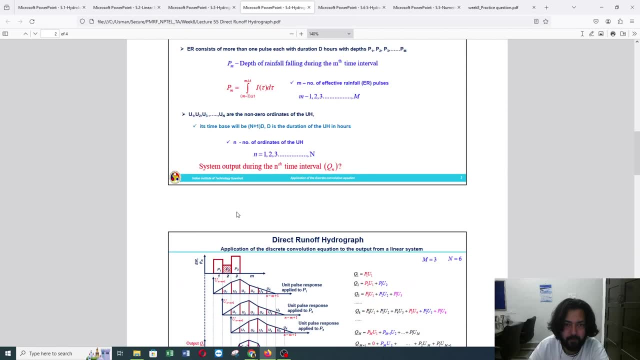 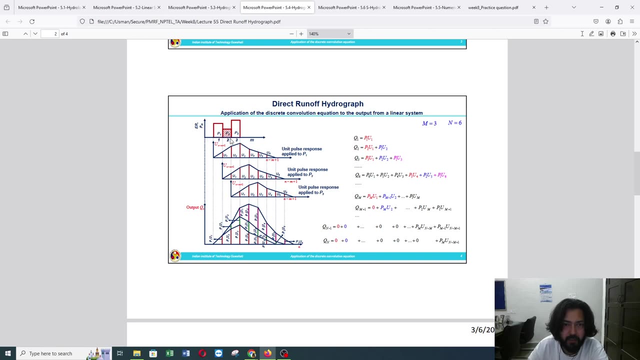 of unit hydrograph. now we can see, like how, how we can apply this to a problem. so if you look at the figure here, this is the input, right? so input is nothing but a pulse, a pulse for div. so there are three input: p1, p2 and p3. so what we are going to do, we 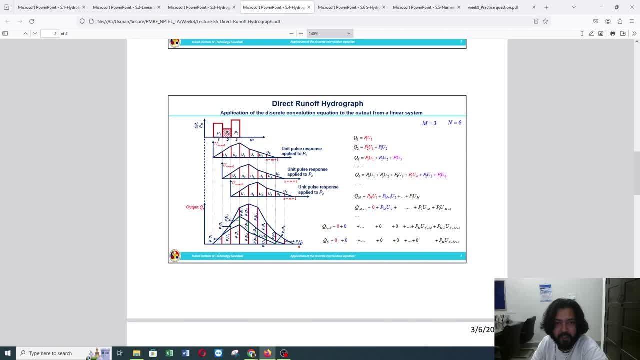 are going to calculate the pulse response for each of these inputs. so we are going to calculate the pulse response for each of these inputs. that is, we are going to calculate the input pulse and response which is applied to p1, then which is applied to p2, and then which is applied to p3, and then we are going to 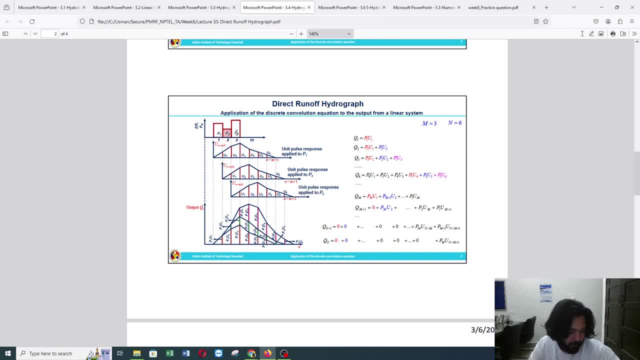 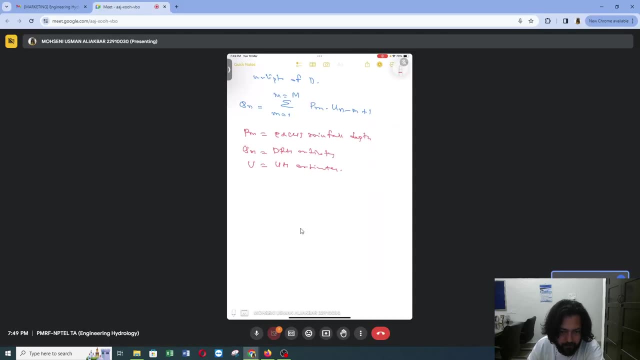 take the summation in order to get the final output right. so let us see how this equation can be used in order for different different pulse. so let us say we have three input pulse. so this is the effect to rainfall, right? so we have three input pulse. 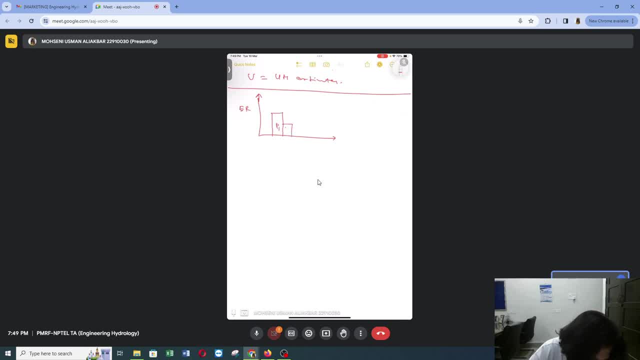 that is p1, we have p2 and we have p3, right. so these are three input pulse. so for each input pulse will have, for each input pulse will have the input response right, the response function. So for P1, so for P1 the response function will start from P1, right and it will 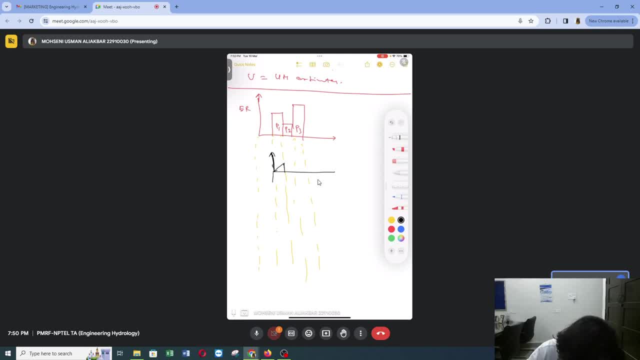 goes something like this: right, this will be U1,, then it will be U2,, then it will be U3, U4, U5 and U6, right? So this is the response function of applied to P1,. this is the response function which. 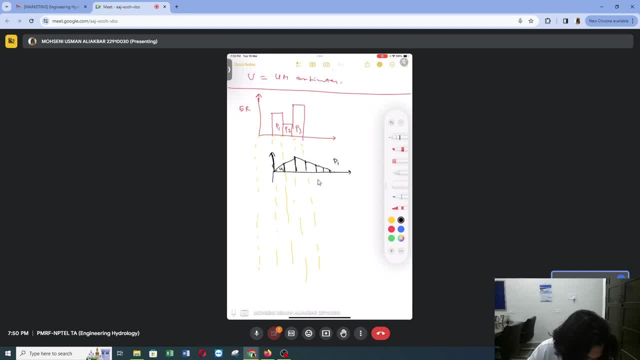 is applied to P1.. Now let us say, let us calculate the response function which would be applied to P2. So there will be some time lag, so that time lag will be of this one. so the response function will start from U2, that is, from P2.. So the response function, 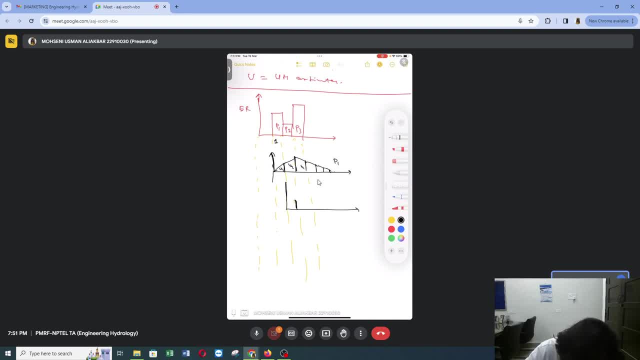 will be. this will be U1, U2, U3, U4, U5.. So this will be U1, now this will be U2, U3, U4, U5 and then it will be U6, right. 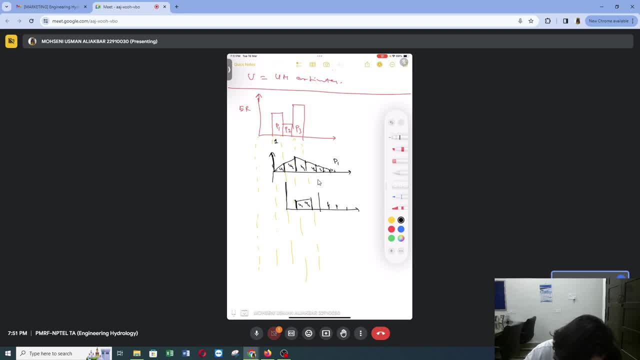 So this is U6 and this is applied to P2, so similarly, it would be applied to U3, also, right, when it is applying to u3, this will be u1, u2, u3, u4, u5 and u6, right? so this is the response. 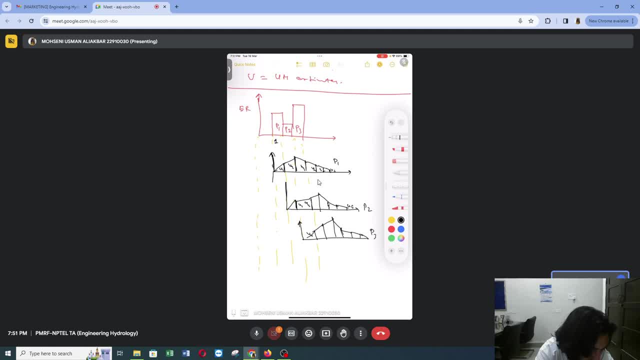 function that is applied to pulse input, pulse 3. now what we are going to do? we are going to add the response function right to get the output. so this is the output: q. so the response function would be here: that is starting at p1. this is called u1 times of p1 because here it is u1 and here it is p1, so this is u1 times. 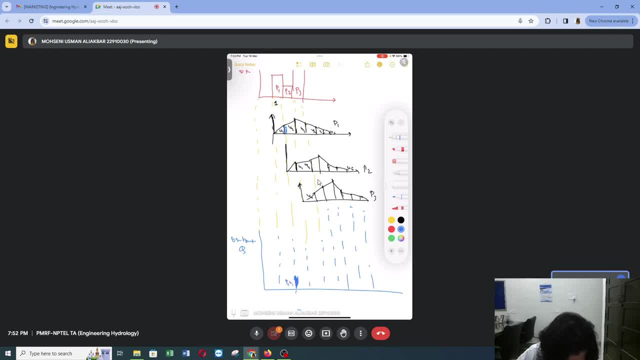 of p1, that is p1- u1, right? so this is for first function. then it will be p1- u2, then it will be p1- u3, p1- u4, p1- u5 and then it will be p1- u6. so this is the output because of first impulse. 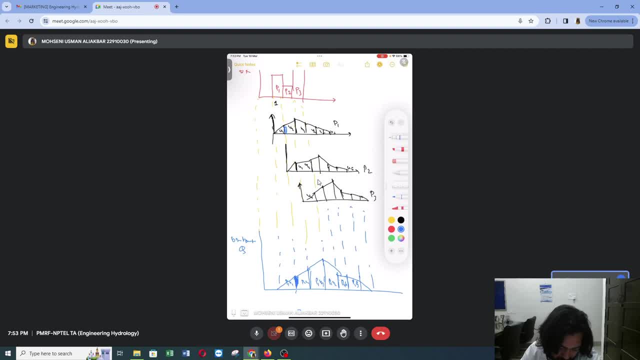 and first output response function. right, so p1, u1. the next would be because of p2, u2, right, so it will start from here. then similarly for third, so third one, it will start from here, right? so if we want to find the output for individual response function, that is we want. 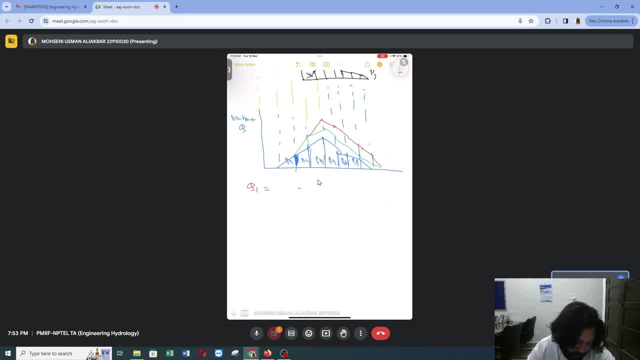 to find q1, so q1 is nothing but product of p1 and u. if you want to find q2, so q1 will be because of p2, u2, p2, p1, u2 will be because of p2 is a function of a. so in terms of q2, the output. 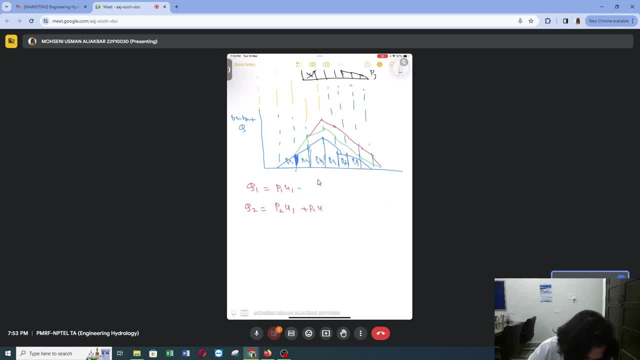 will be well recall of couple of other components. now we have another formula in which we would p2 u1 plus p1 u2 and similarly q3 will be because of p3 u1 plus p2 u2 plus p1 u3. So 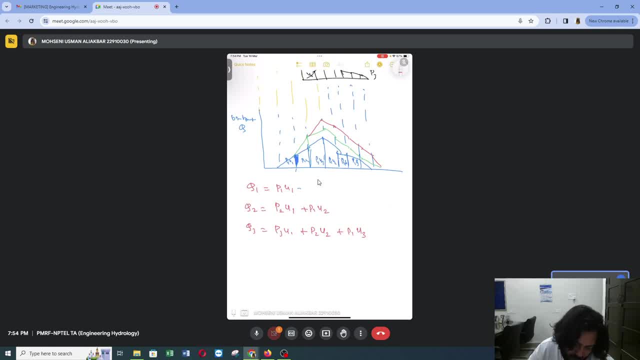 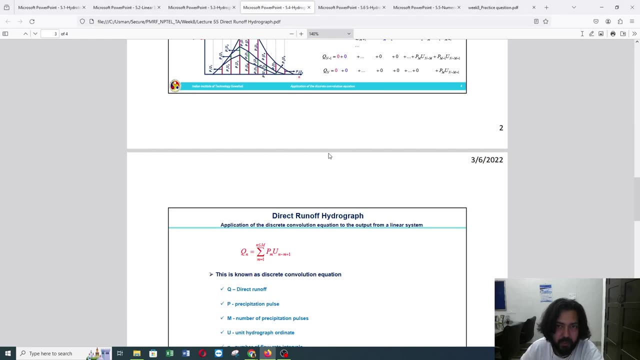 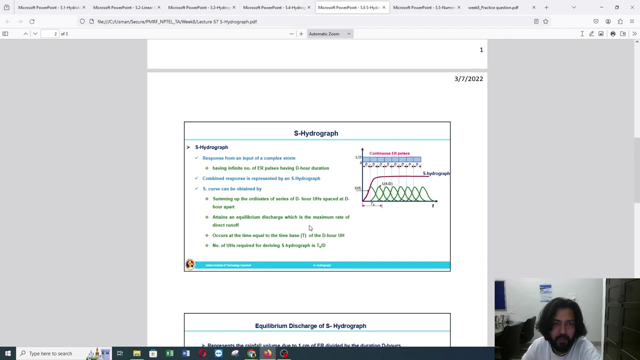 if you want to find, want to generalize this equation, that generalized equation is nothing but this equation. So in this way we can, in this way we can derive drh from a unit hydrograph. Now let us see what is s hydrograph. We have studied like what is unit hydrograph? 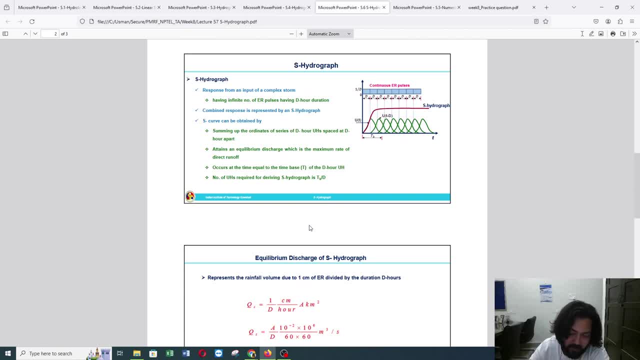 So in unit hydrograph the important thing to understand is that it is resulting from 1 centimeter excess rainfall, which is occurring unilaterally. So in unit hydrograph the important thing to understand is that it is resulting uniformly over the catchment, having a uniform r like for a effective r. that is dr so s hydrograph. 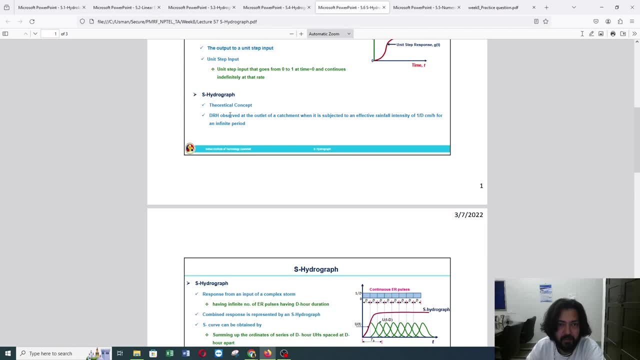 is nothing but s? hydrograph is defined as a drh observed at the outlet of catchment, where it is subjected to a effective rainfall intensity of 1 by d cm per hour. so the important thing here to understand is that it is subjected to an effective rainfall intensity, whereas 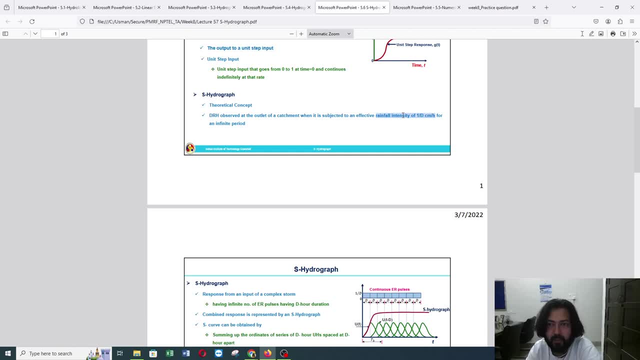 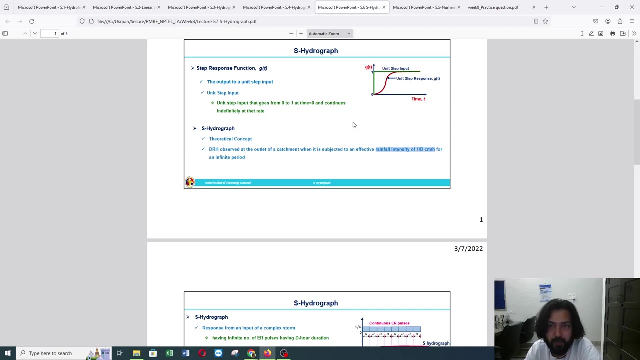 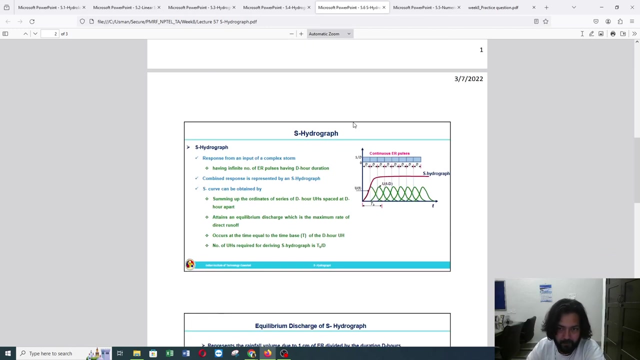 unit hydrograph was subjected to an effective of unit excess rainfall. right. here it is a because of unit rainfall intensity of 1 by d cm per hour. also, the important thing to understand here is: the unit hydrograph was based on the unit pulse response function right, whereas s hydrograph is based on unit step response function. now let us see like: 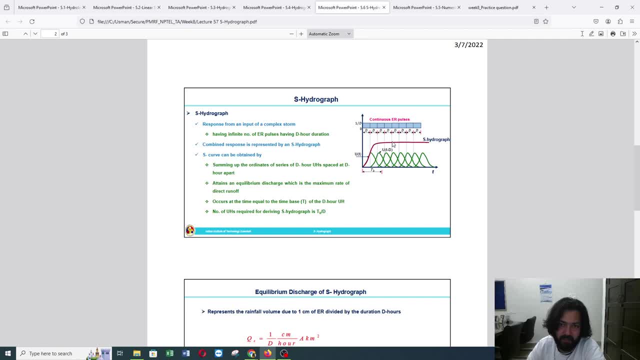 how does how to obtain s careers hydrograph your s curve? so it is based on a complex storm like it is having a complex term for of multiple, multiple storm event right. so it is having an infinite, infinite number of effective rainfall pulses having dr duration, each here in the figure. we can say that, whereas in 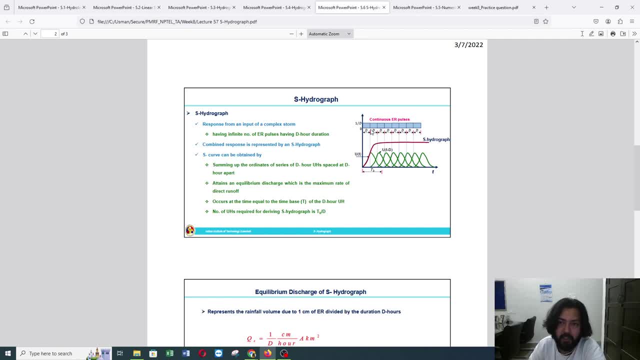 unit hydrograph there was only one input when we are talking about single storm duration event, whereas for s hydrograph there are multiple number of effective rainfall pulses, is having dr duration and the combined response is represented by. the combined response of this input is given by s hydrograph right. so how can, how we can obtain this? so can be obtained by. 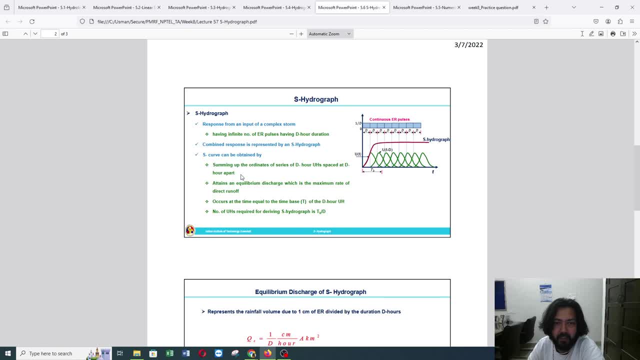 summing the ordinate of series of dr unit hydrograph spaced at dr apart. so what we are going to do for this input pulse will calculate the output first, so that output is nothing but u times of t. so for second, it would be u times of t minus d. there would be some time lag and 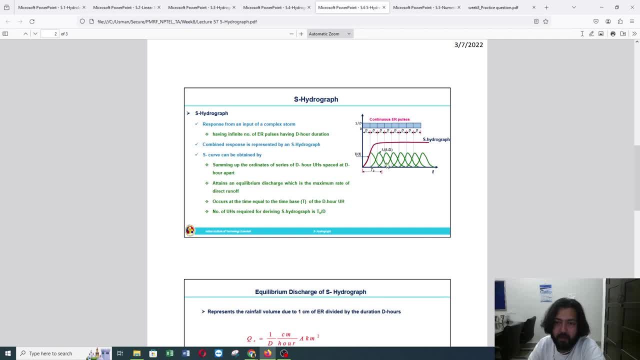 then it will occur like this: so for second, it would be u times of t minus d. there will be some time lag. and then it will occur like this: so for second, it would be u times of t minus d and remain same, but there would be some time lag associated with it. then the important thing, 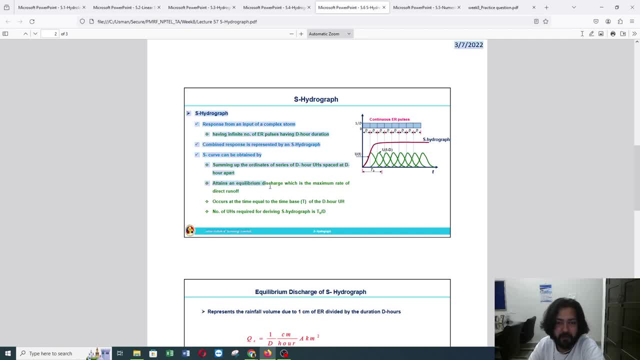 here is in S hydrograph. it will. there will be some equilibrium discharge, which is the maximum rate of direct runoff. what is this equilibrium discharge? we will study here in the next part. and also, in order to calculate a S hydrograph, we required number of unit hydrograph, and those number of unit hydrograph can be obtained by this term time base, by: 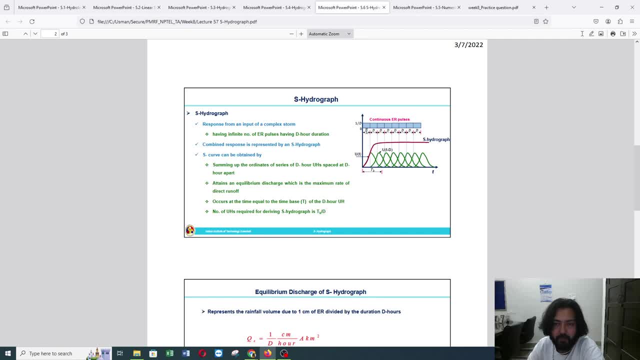 D. so if we know the time duration- like the D are from storm- for the each storm duration for each storm event, and we know the time base right, so then, dividing the time base to the duration, we can calculate the number of unit hydrograph that are required. so let's 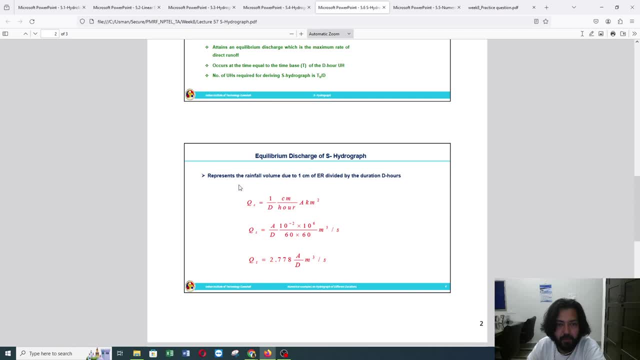 talk about equilibrium discharge here. so in order to represent the rainfall volume due to 1 centimeter of excess rainfall divided by the duration of R, we can calculate equilibrium discharge of S hydrograph. so that is nothing but 1 by D of area. so this 1 by D is nothing but centimeter per R and area is in kilometer. 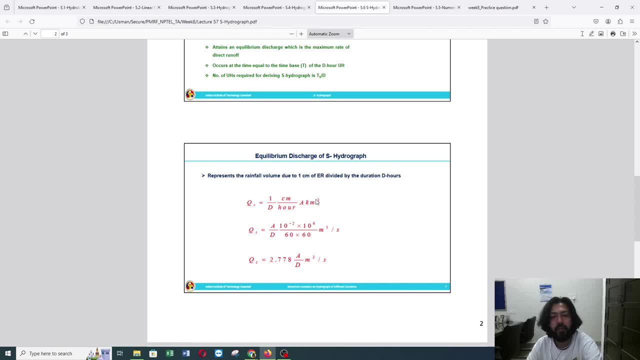 square. so we want to convert this into the unit of discharge, which is meter cube per second. so we can convert this centimeter into meter. that is 10 to the power of minus 2. this area, which is in kilometer square, we can convert this into meter square by 10 to the power. 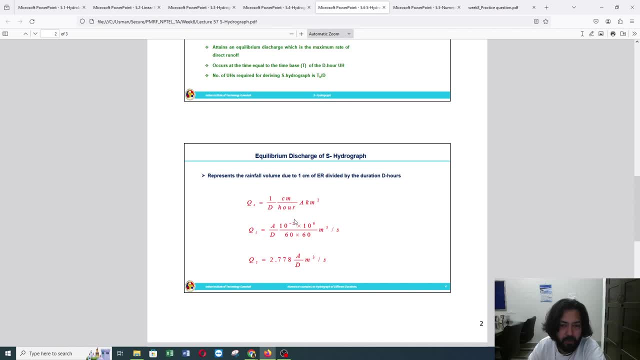 6, so the numerator is in meter square, meter cube now, and R we can convert into cent second. that is 60 by 60. so we can convert this. we will get the equation of discharge, which is meter cube per second, and the formula of equilibrium discharge will come up to be: qs is nothing but 2.77 of 8 multiply. 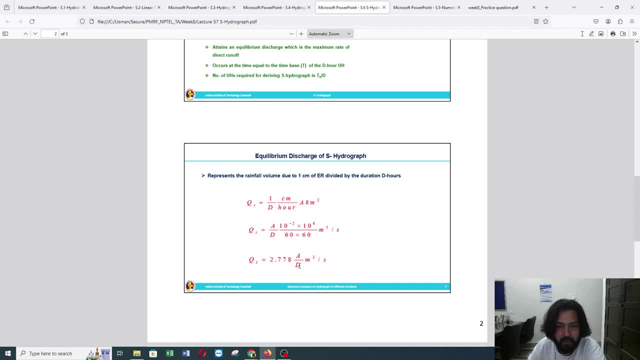 by area and divided by time, right duration of storm. so we should keep in mind here is, if you want to use this equation directly, the area should be meter square and time should be in second. then we can apply this equation directly, or else we have to go with the standard. equation that is area divided by duration of storm. so we can apply this equation directly, or else we have to go with the standard equation. that is area divided by duration of storm. so we can apply this equation directly, or else we have to go with the standard equation that. 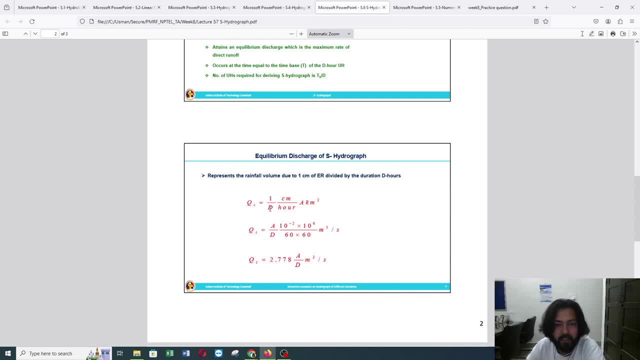 is area divided by duration of storm, so we can apply this equation directly. or else we can apply this equation directly, or else we have to go with the standard equation. that is area divided by duration of storm. so we can apply this equation directly. or else we can apply this equation directly, or else we have to go with the standard equation that. 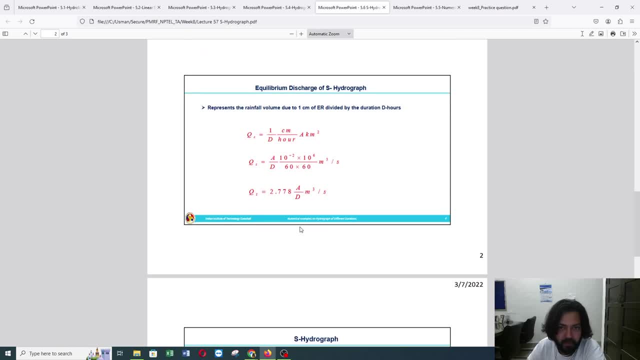 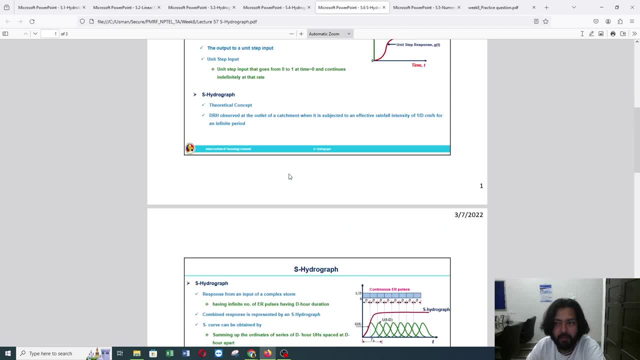 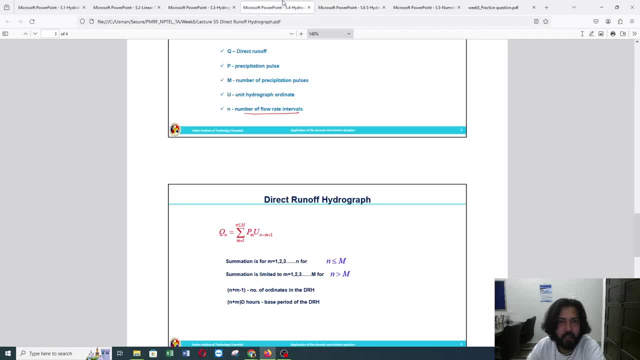 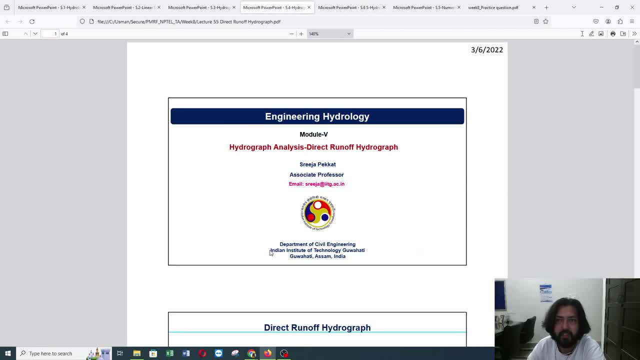 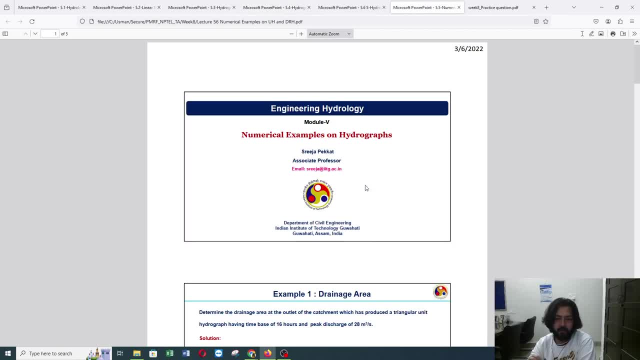 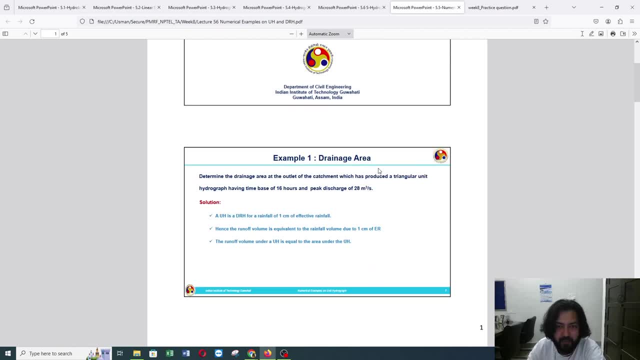 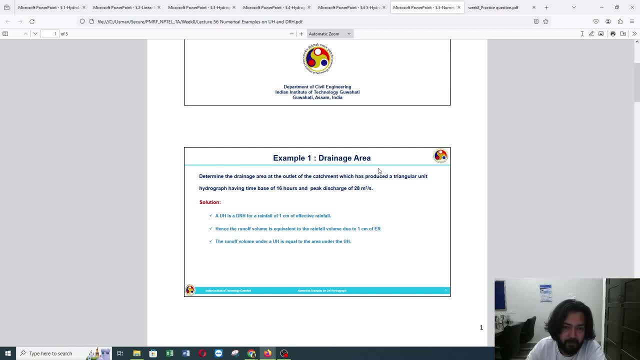 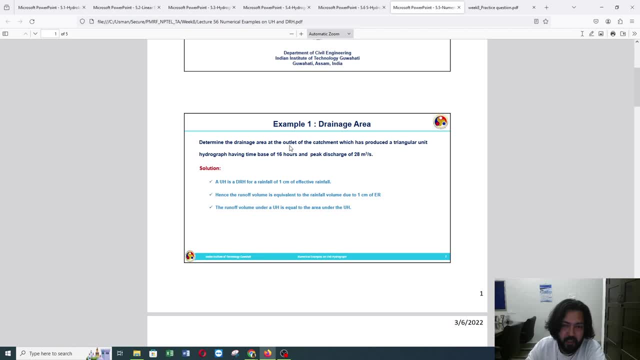 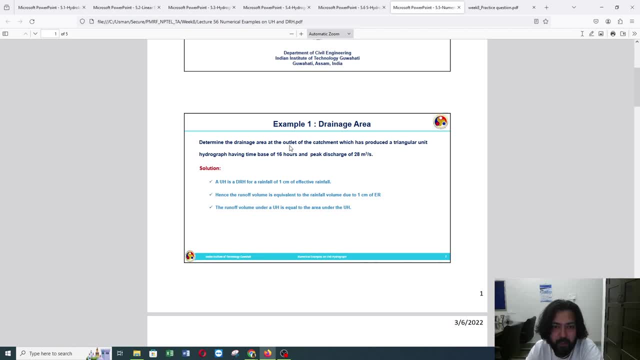 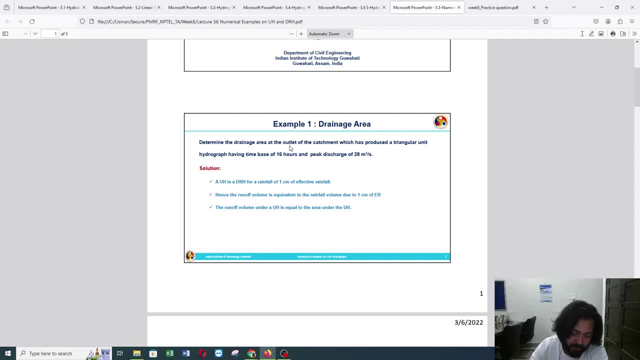 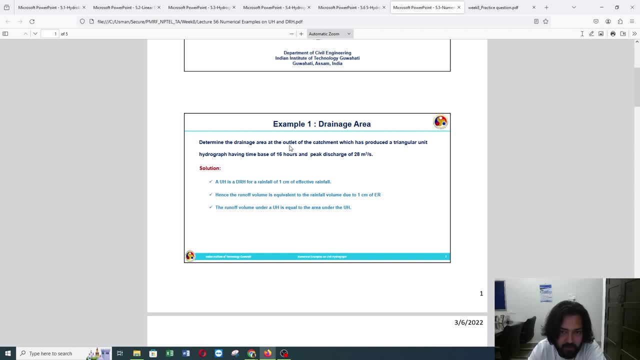 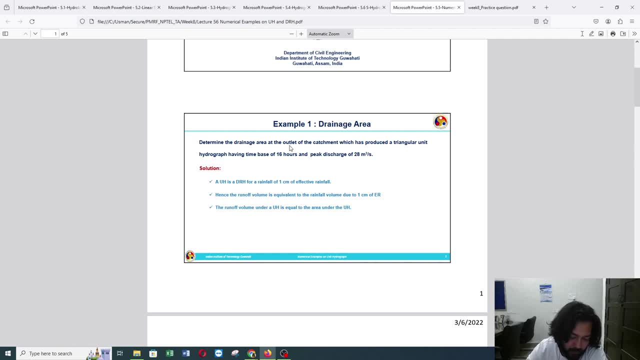 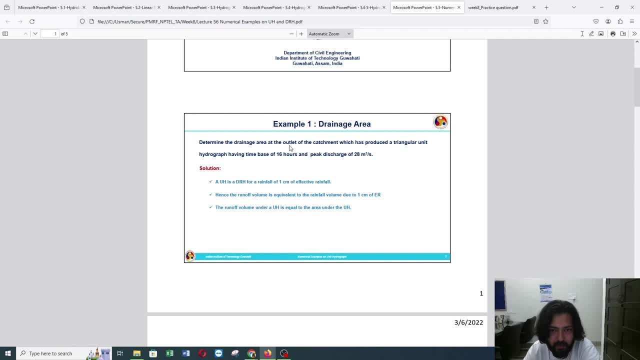 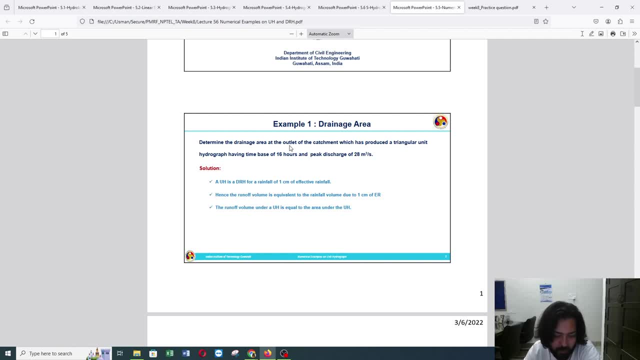 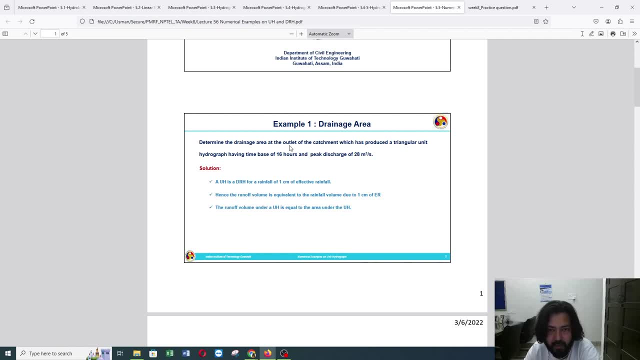 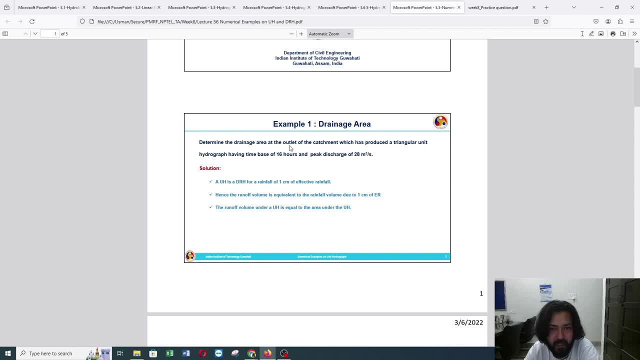 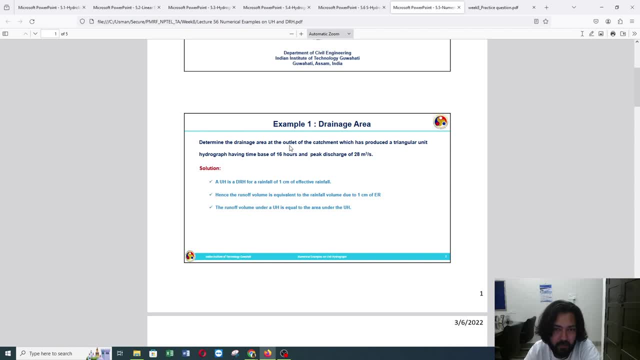 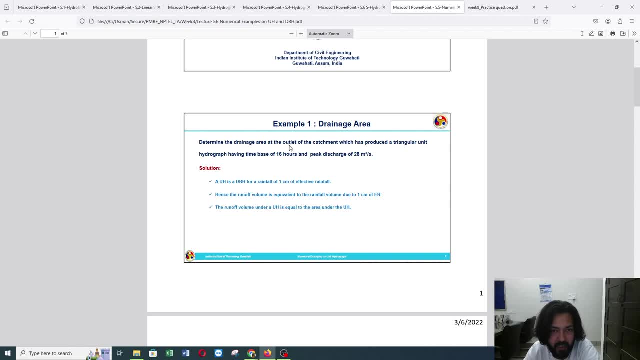 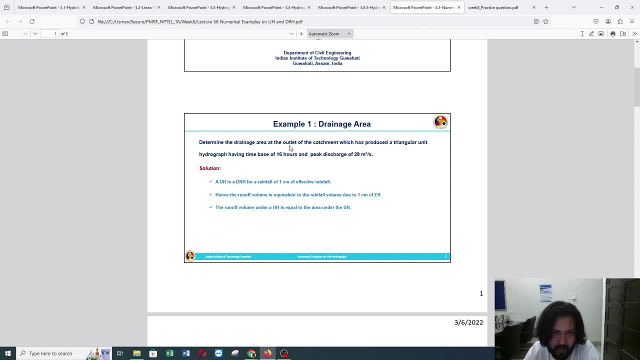 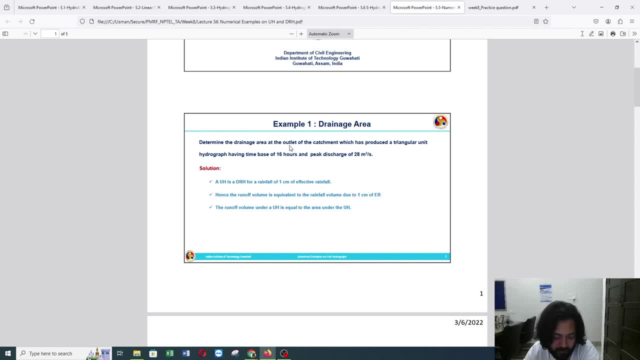 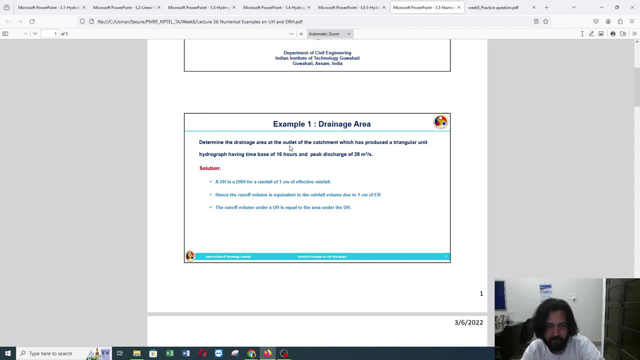 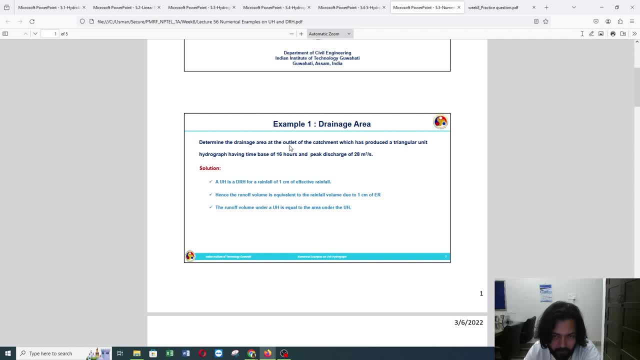 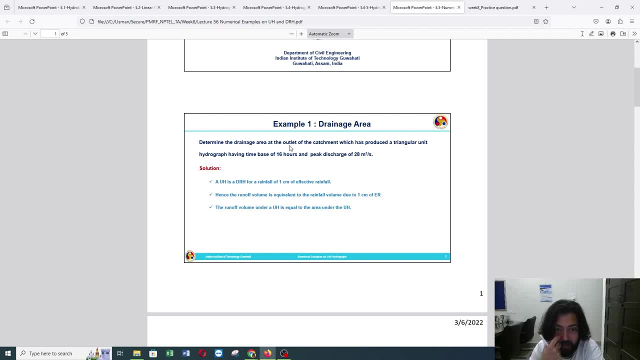 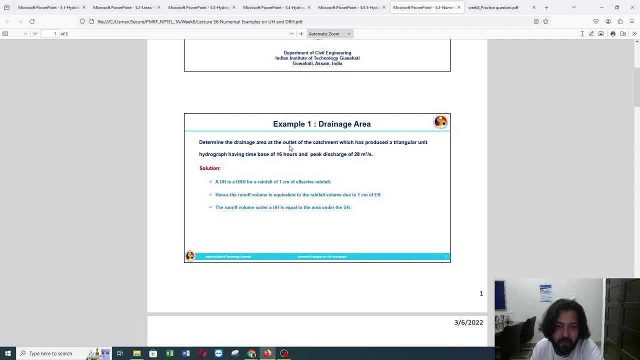 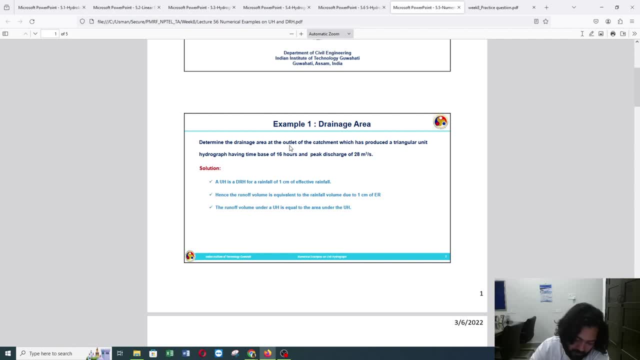 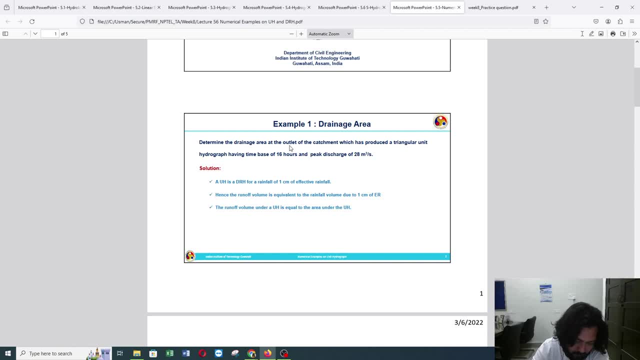 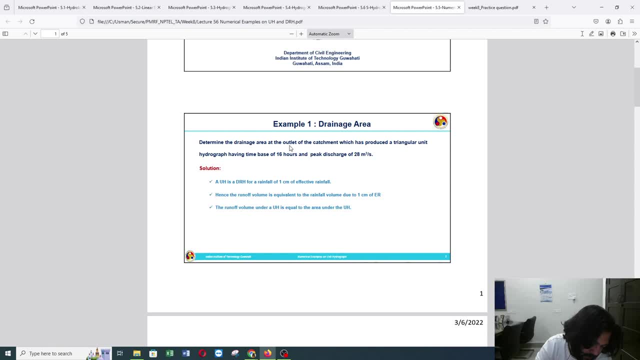 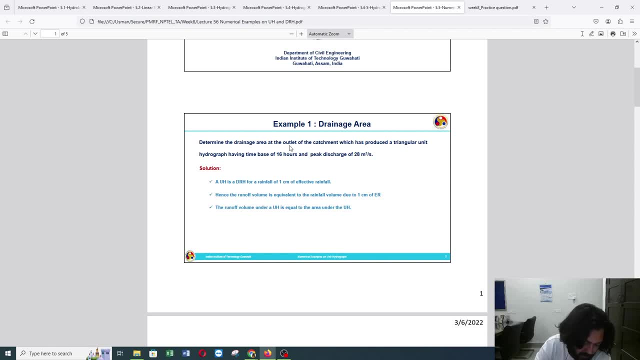 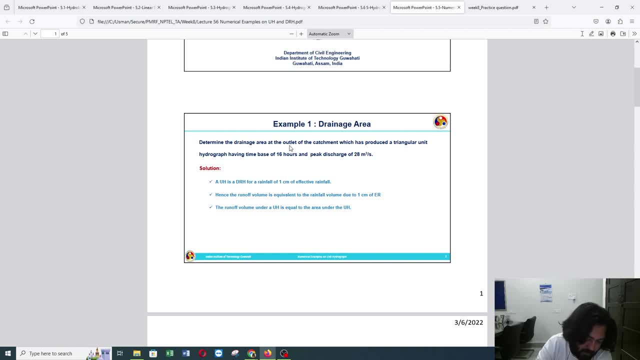 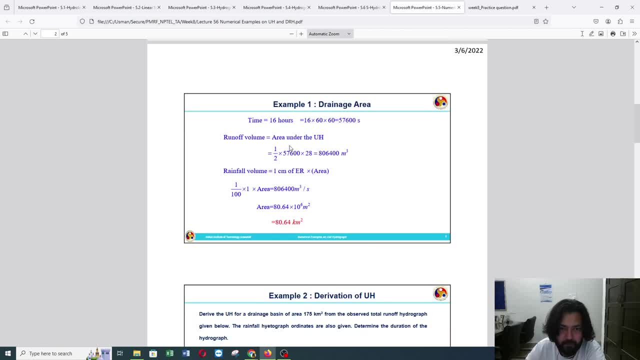 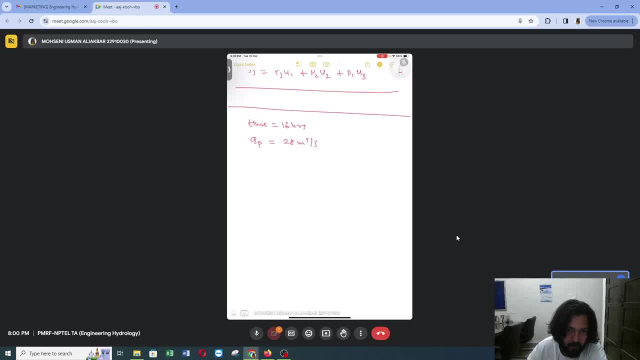 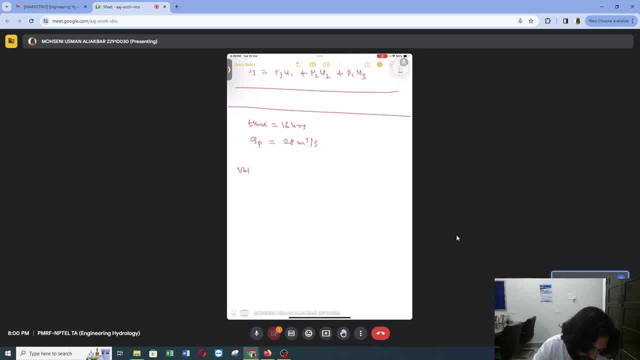 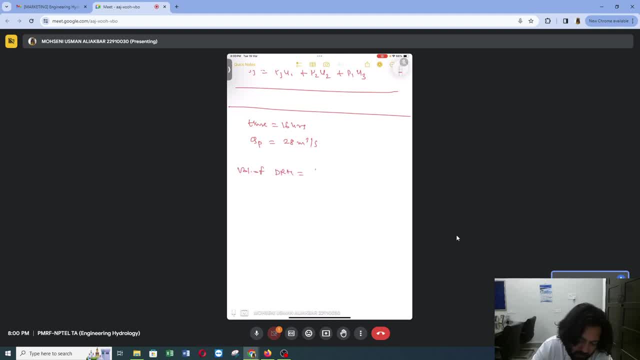 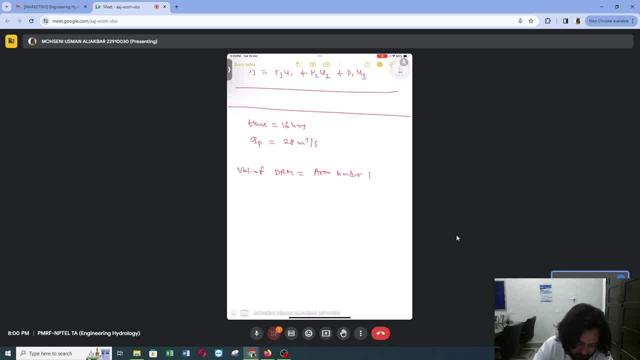 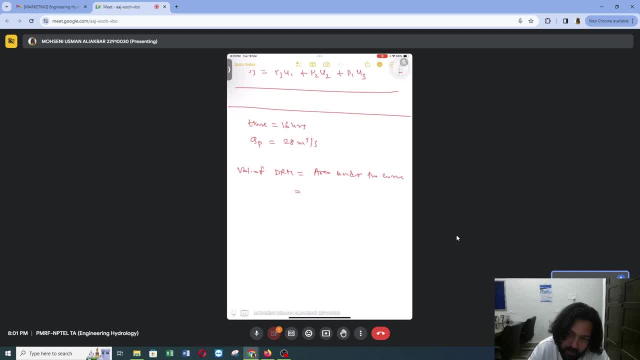 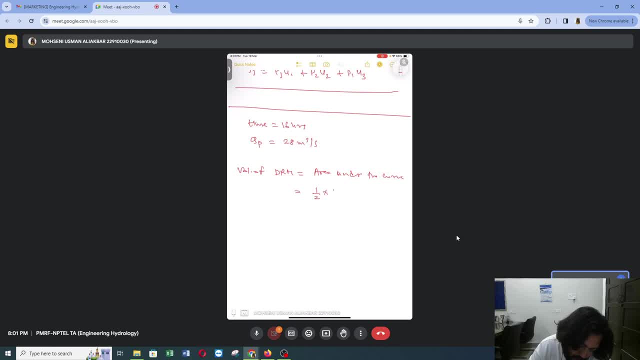 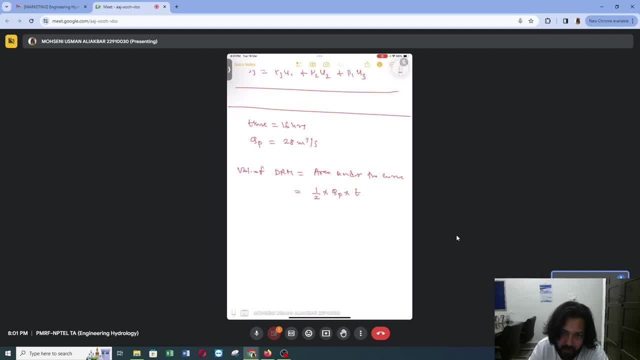 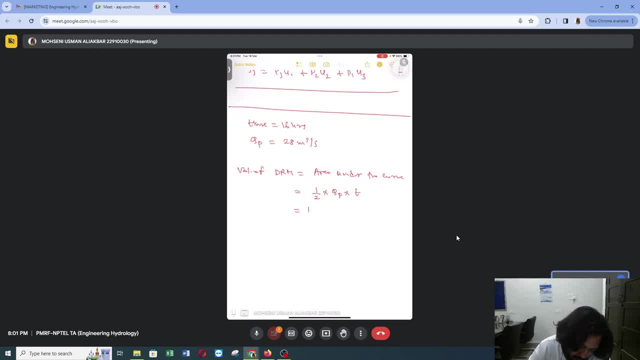 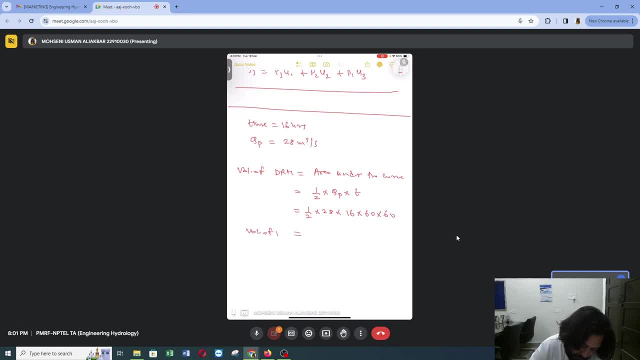 multiply this term, we will get the volume of DRH right, which will be in meter cube. now the next thing is to calculate. they have asked us to calculate the area, actual area of the catchment. so how we can do that, since we know the volume, we can calculate the depth. 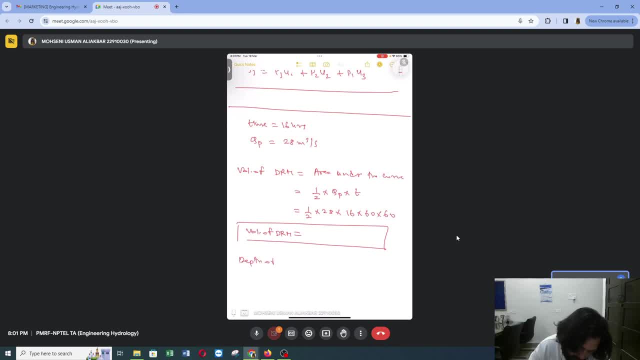 of ER. so there is another formula of depth of ER which is equals to volume of DRH divided by catchment area. right, but in this problem they have asked us to calculate catchment area and depth of ER, for unit hydrograph is 1 centimeter, that is, 1 into 10 to the 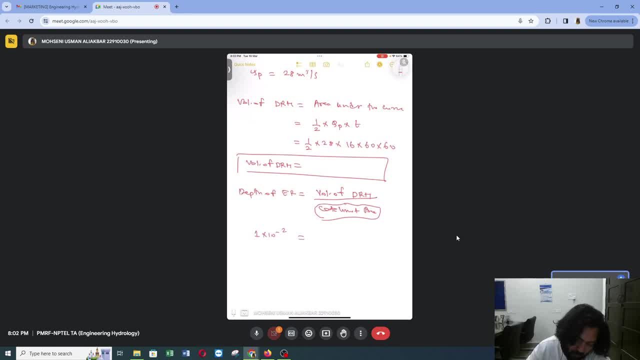 power of minus 2, and volume of DRH is known to us. so the only term that is unknown to us is the volume of DRH, so that is known to us. so the only term that is unknown to us is catchment area, so we can calculate: catchment area equals to. so this is a very 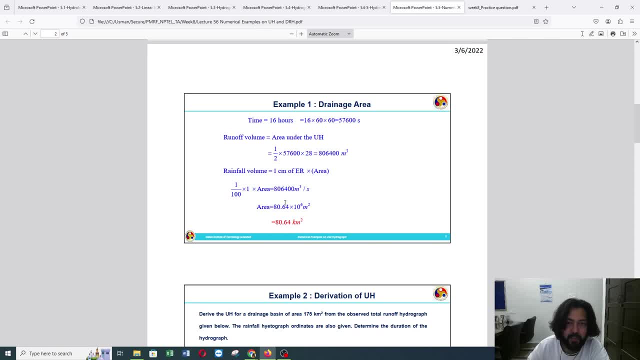 simple problem. we can see the solution also. so see: first, they have calculated the runoff volume or volume of DRH, which is 806400 meter cube. now, since we know this volume, we can simply divide it by excess rainfall and we can get the value of area. so they have divided. 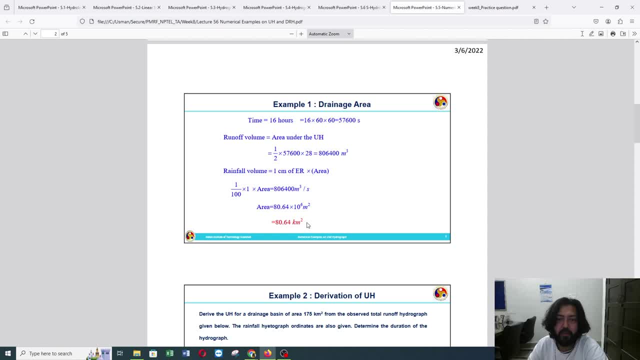 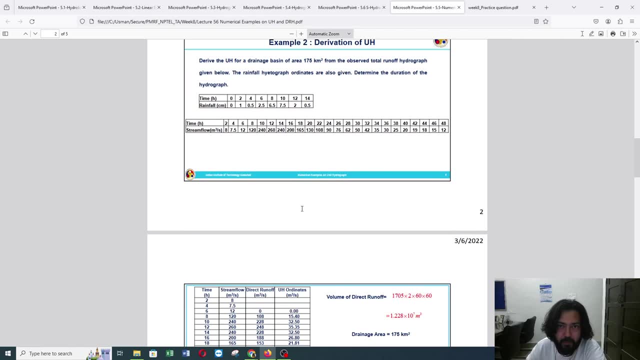 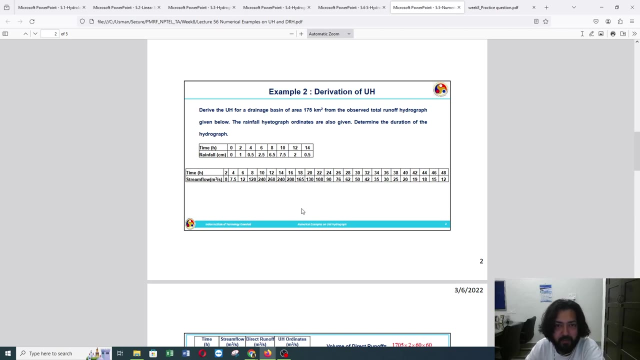 here. so they have calculated the area also. so the area comes up to be 8.6410 to the power 6 of meter square. so this is very simple problem. just we know. we need to be very clear, like how, what are the steps to calculate the DRH of unit hydrograph? now, next question. 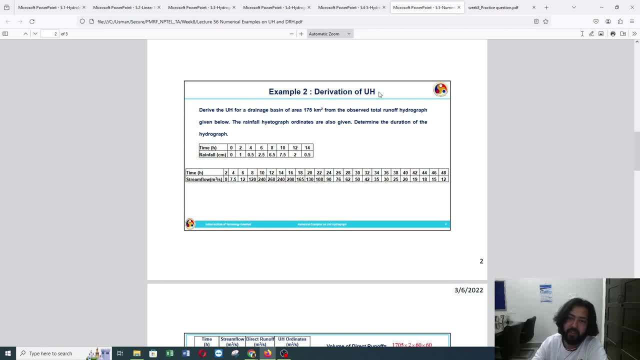 they are asking is derivation of unit hydrograph. so they are asking us to derive a unit hydrograph. so they are saying that derive the unit hydrograph for a drainage basin of 175 kilometer square from the observed total runoff hydrograph given below. so here they have given the 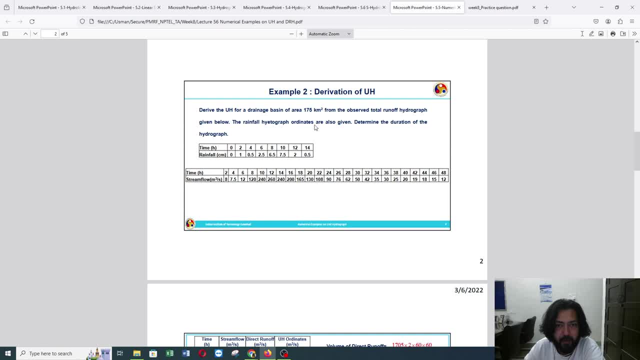 runoff hydrograph value. here also they have given the rainfall hydrograph coordinates determine the duration of hydrograph. so here they have asked us to determine the duration of hydrograph. it means whether the duration is 2 hours, whether the duration is 4 hours. 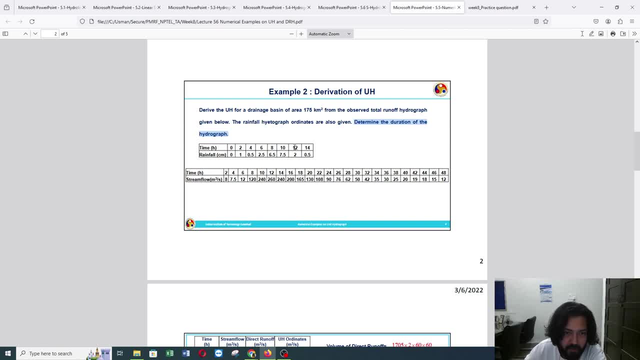 or 6 hours that we need to derive. so how we can do that here is, since they have given us the discharge value and they have given us the input right, so we need to calculate. first thing is to calculate DRH. so how we can calculate DRH from unit hydrograph is: 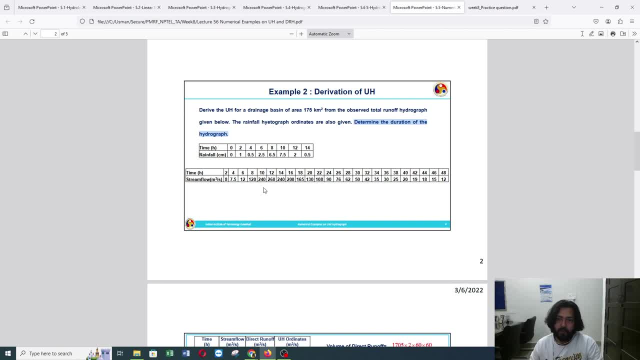 by. first we need to do is we need to separate the base flow. so first thing we should do is we should first look at the given data and we should calculate the base flow. so if you look at this data set, we can say that the value of 12 meter cube per second is repeating. 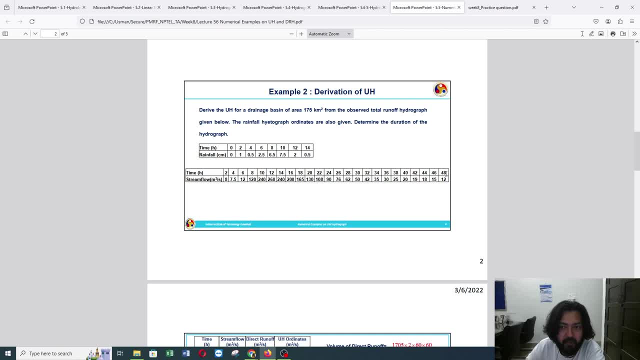 here. like it is 12 for time of 6 hour and again after 48 hour it is 12, so we can say that this 12 is nothing but 12., 12., 12., 12. 12.. 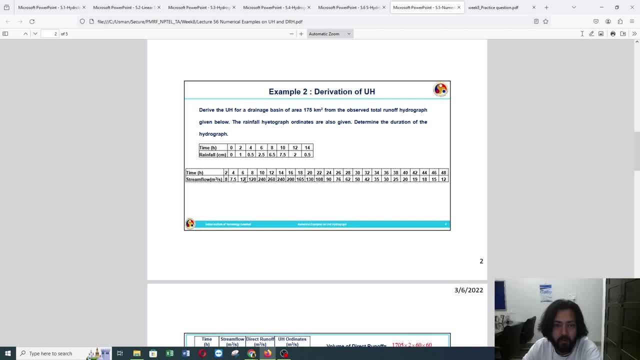 but it could be a base flow, it could be because of the base flow, right? so what we can do is we can first step- is to calculate the drh from the given data set. so in order to know the drh, we need to know the base flow. so here, what we are going to do is we are going to 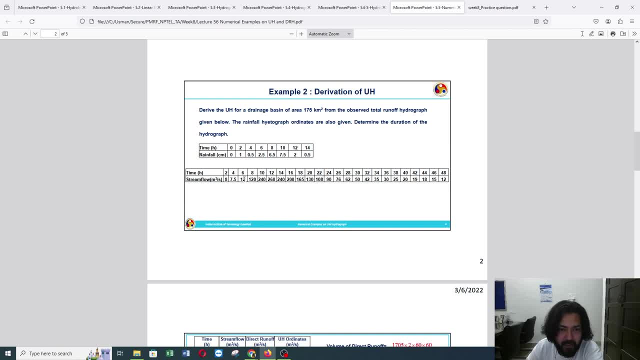 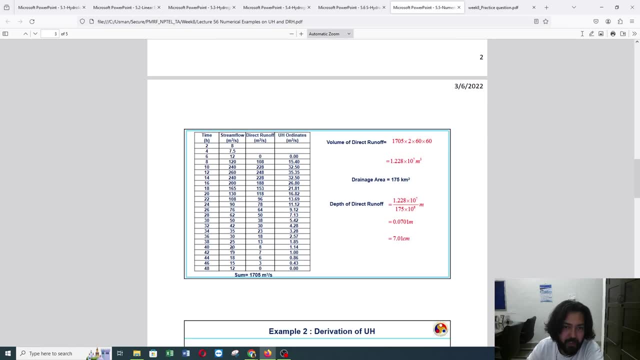 take base flow as 12 and then we are going to subtract this base flow from the given data, then we will get the value of drh. so here we can see this is stream flow data and then they have calculated direct runoff. so how they have calculated direct runoff, they 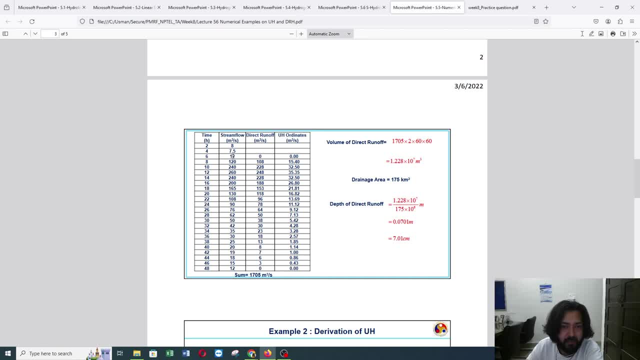 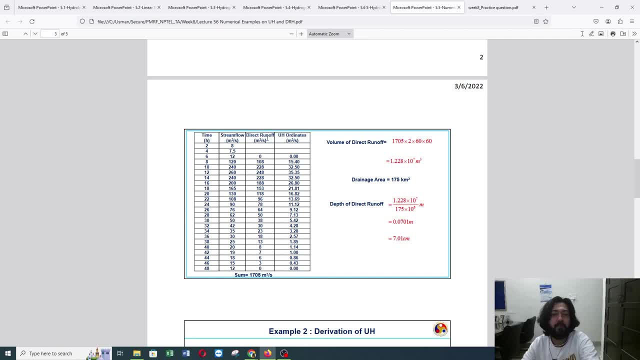 of drh. now the next step is to calculate the effective depth. since we know the volume, now we can calculate the volume. how we can calculate the volume, we know the peak value, like we know the total value. so the total value is 1705 meter cube per second. so this value we are going to 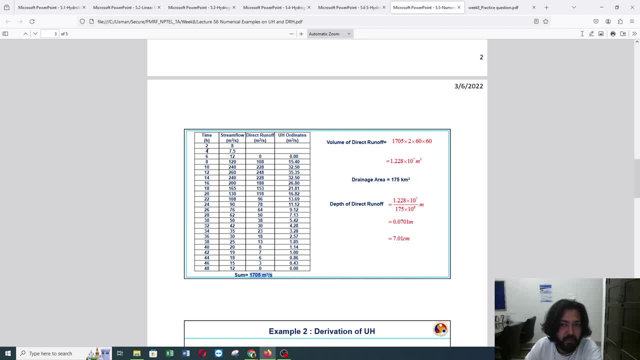 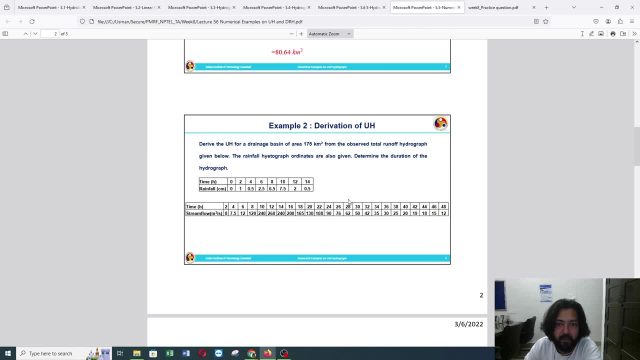 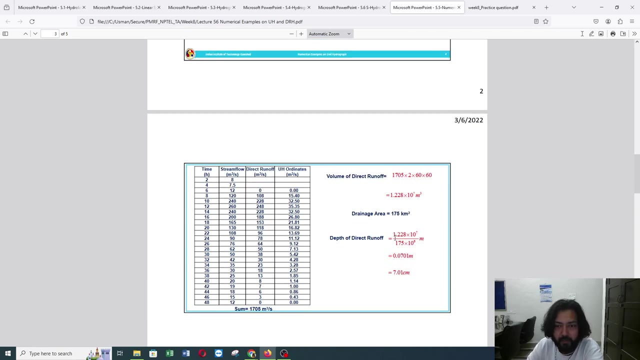 multiply with the duration, so the duration is 2 hours. so 2 hours means 2 into 60, into 60, so we got the volume of direct runoff and also we know the value of drainage area, so we know the volume. we know the area, so we can get the value of excess depth, of excess runoff. so we got the. 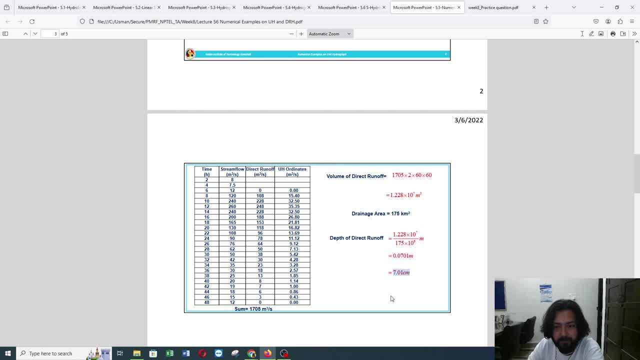 value of depth of excess runoff, which is 7, right? so we got the value of excess runoff, which is 7 centimeter. so now what is the next step? the next step is to calculate the ordinates. how can we get the ordinates of unit hydrograph? by dividing this value of 7 with the direct runoff. so once. 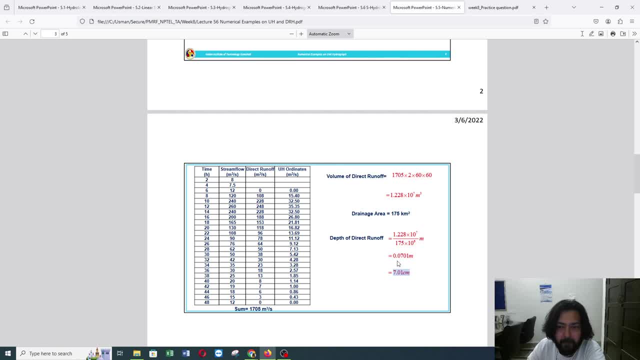 708, which is in meter cube per second, divided by 0.07, sorry, divided by 7.01, so we got the value of 15. similarly, 228 divided by 7, we got the value of 32. so, similarly, we are getting the ordinates of unit hydrograph. right now. the next step is to 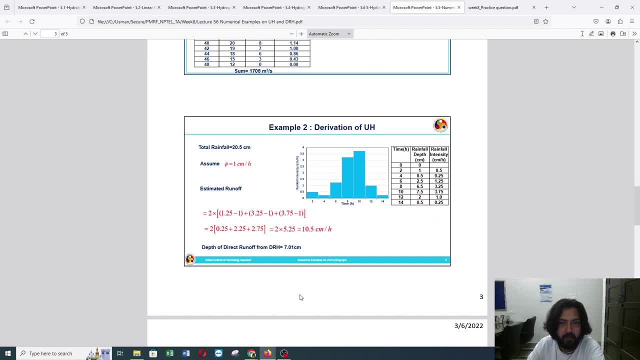 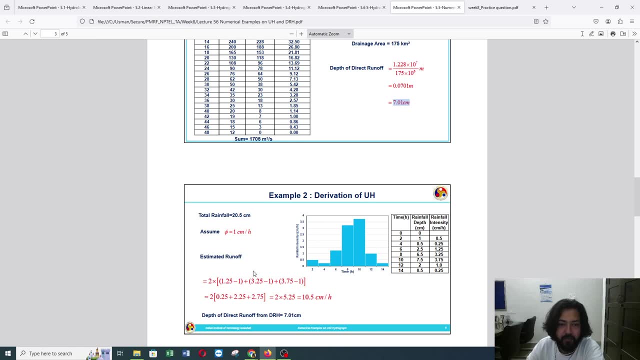 now the next step is to calculate the is to plot rainfall hydrograph. so, in order to plot rainfall hydrograph, what we need is we need rainfall intensity. so what we have done here is we have divided the depth of rainfall with the time duration, so 1 divided by 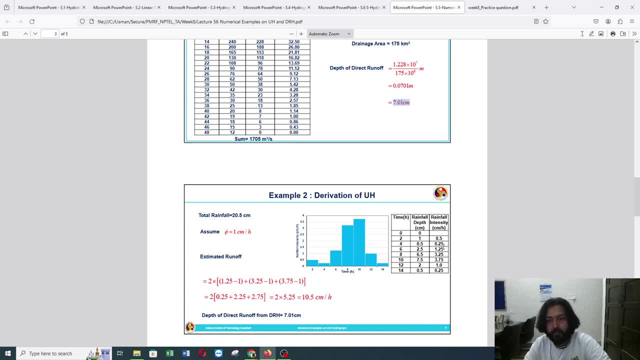 2.5.5 divided by 2, 0.5 because the time duration is 2. so we'll divide each value, each rainfall depth, with 2. we'll get the rainfall intensity. so we have plotted this rainfall hydrograph. now what we need to do is we need to calculate, we need to assume the value of phi such that 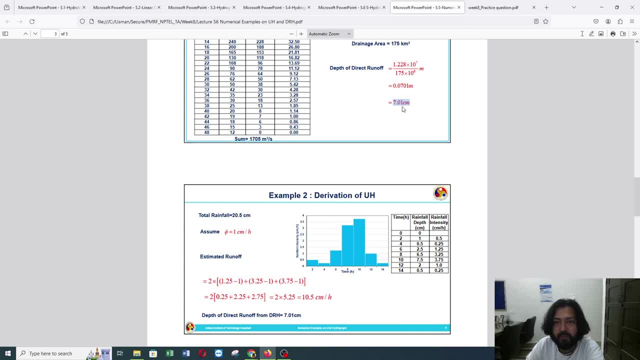 the estimated runoff is equals to the depth of runoff. right, it means the excessive rainfall value, that is, the input, should be equal to the output, which is the depth of runoff. so the input and output is matching. we can say that the phi value is whatever phi value we are assuming is. 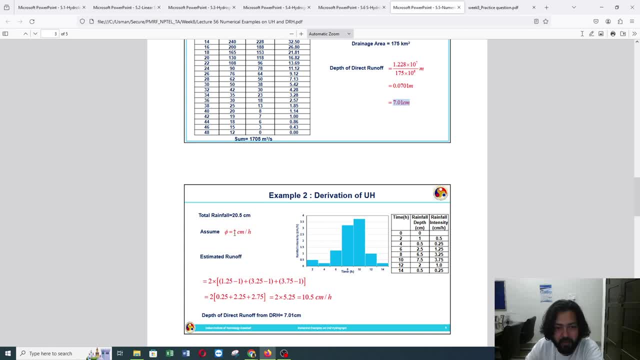 constant. why we are doing this is because, based on the value of phi, we can separate the drh value. we know that we have studied this in previous week also. so, firstly, we have assumed phi value is equal to 1 and we got the estimated runoff is equals to 10.5, which is not true because 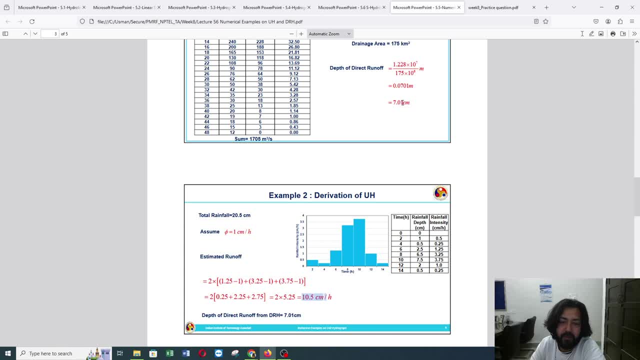 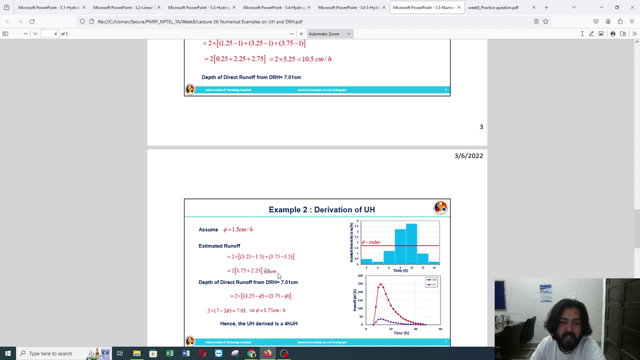 the depth of direct runoff which we got was 7.01. so again, we are going to assume new value. so that new value, which we assumed, was 1.5 and the estimated runoff that we got was 8. so again, it is not true. so what we can do is we can simply take the result, output, result. 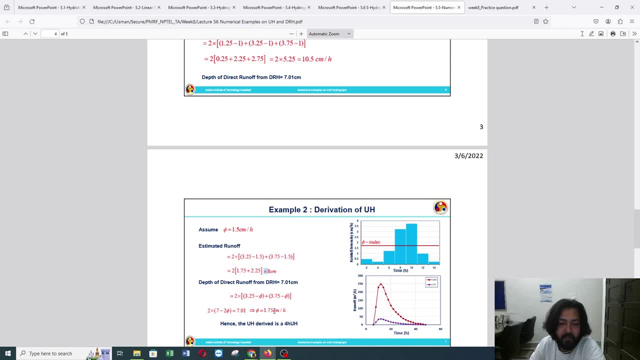 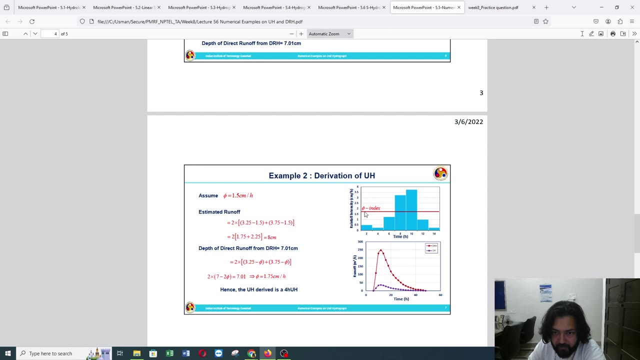 as 7.01 and we can get the value of phi. so that value which we got of phi is 1.75 centimeter. now based on this value we can calculate, like what is the time duration, how we can do that. here in the figure we can say that the rainfall hydrograph, the value of phi index, is 1.75. so 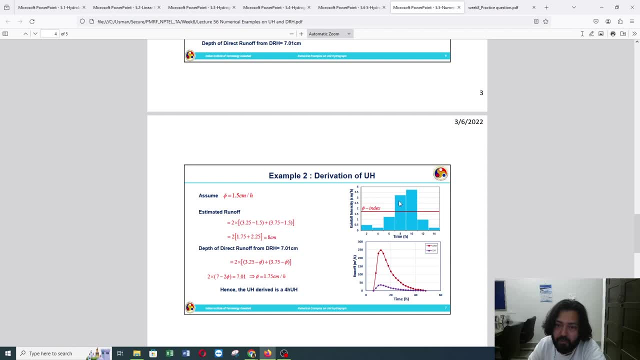 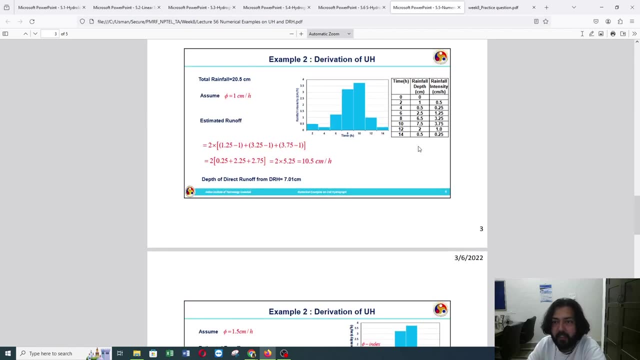 if the value of phi index is 1.75, only those rainfall intensity will be taken whose value is greater than 1.75. so there are how many rainfall intensity values which are greater than 1.75? it is 2. there are only 2 values, that is, 3.25 and 3.25, which is greater than. 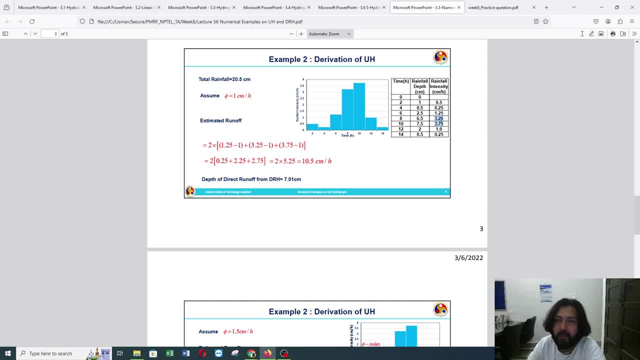 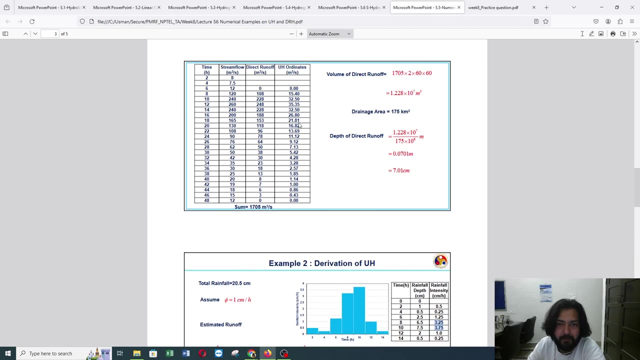 1.75. so only these 2 impulse will be active, that is of time duration of 8 hours and 10 hours. it means 2 hours of this and 2 hours of this. it means total of 4 hours- will be active. so from this we can say that the unit hydrograph which we have derived here- this 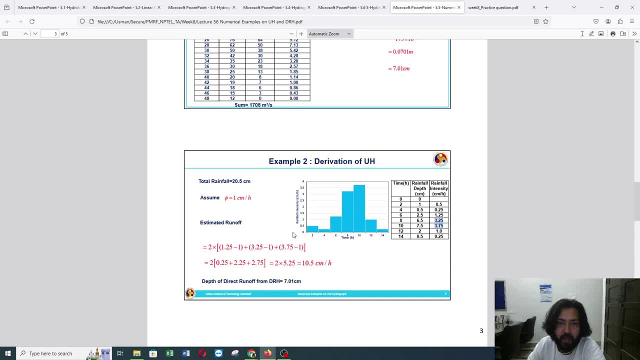 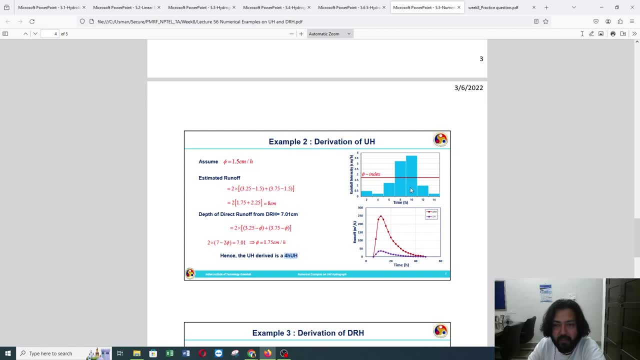 value. the unit hydrograph which we have derived here, is for how many hours. it is for 4 hours and why it is for 4 hours? because when the value of phi is 1.75, only 2 pulse are active, that is, of 3.75.. 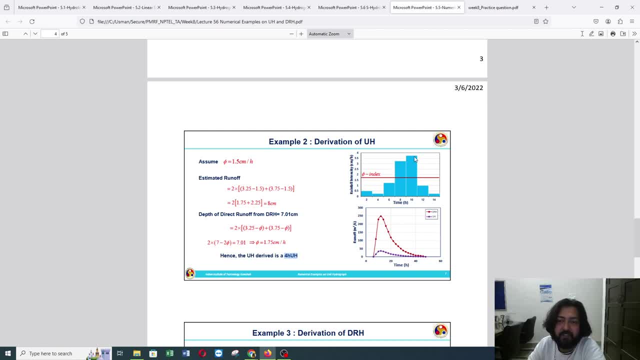 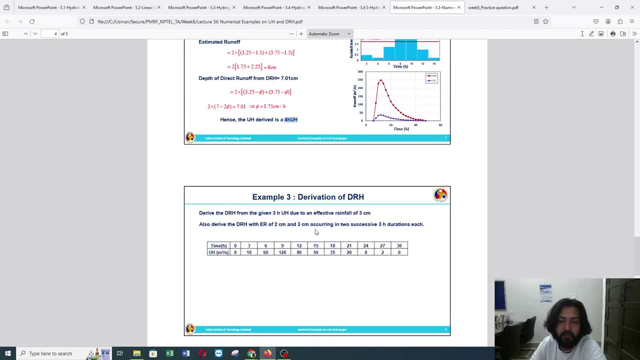 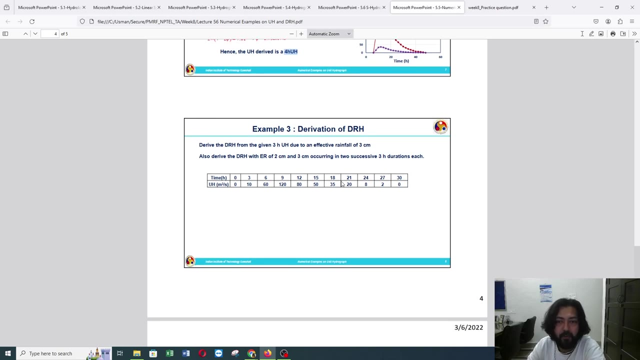 3.25 and 3.75, so 2 hours of this and 2 hours of this, which is 4 hours. so that why we can say that the unit hydrograph that we have derived here is of 4 hour unit hydrograph, right? so this was a problem which was based on how to derived unit hydrograph. now the 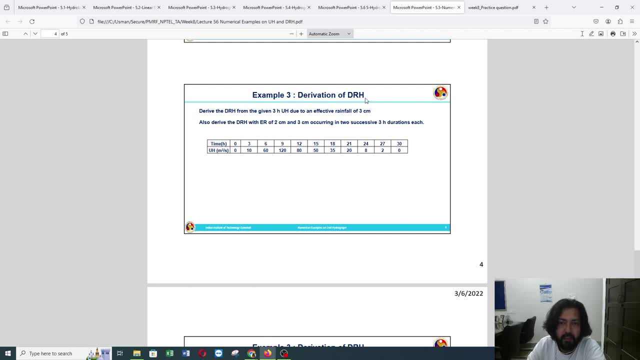 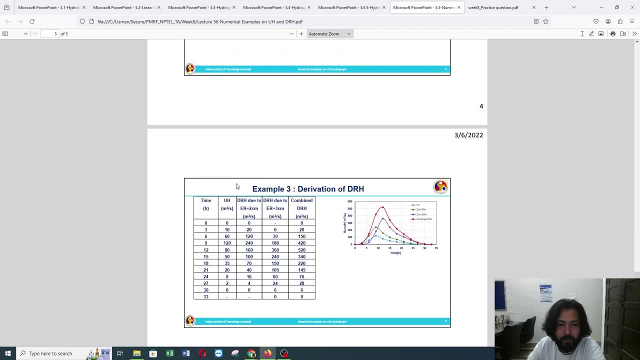 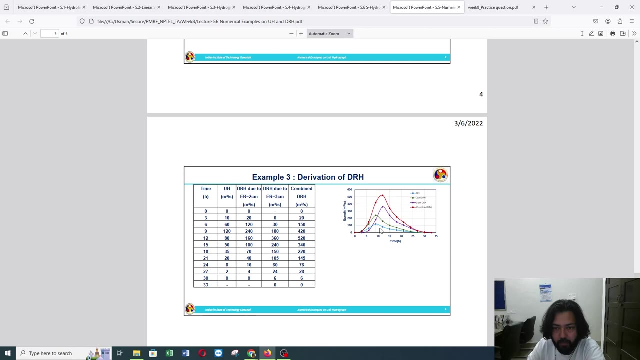 next problem is for derivation of drh. it means they have given us unit hydrograph and from unit hydrograph we have to derived drh. so what we are going to do here is: first, we have plotted the unit hydrograph based on the given value. so this blue plot, light blue. 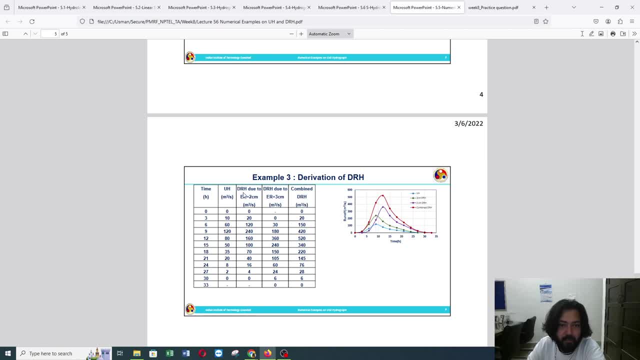 color plot. it shows the unit hydrograph. now we want to derived drh due to excess rainfall of 2 centimeter, right? so what? we can do that in when we want to find the unit hydrograph ordinate we divided by excess rainfall, right? we know this equation: drh is equals to we. 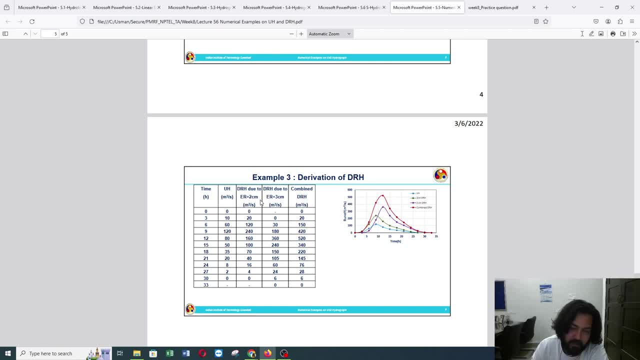 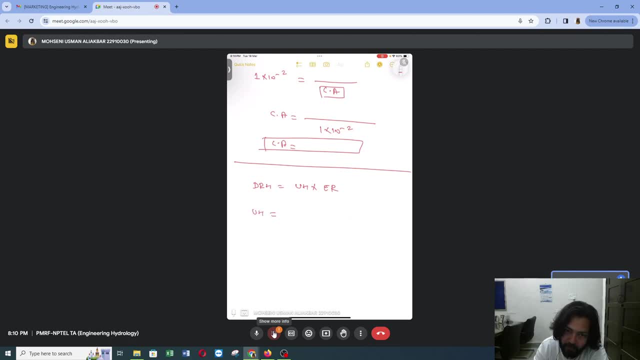 have given unit hydrograph into excess rainfall. right, the relationship here is: if we want to find the ordinate of unit hydrograph, we need to divide drh ordinate with respect to excess rainfall. so we know this. so now what we are going to do: we have given ordinate. 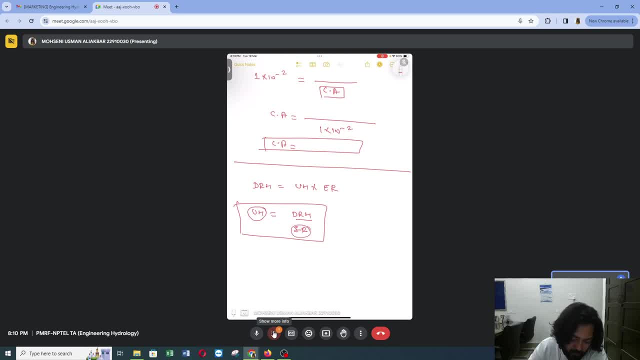 of unit hydrograph and we have been given excess rainfall and they have asked us to calculate drh. so we are going to use this equation. so we are going to use this equation here. so we are going to simply multiply excess rainfall value with unit hydrograph ordinate. 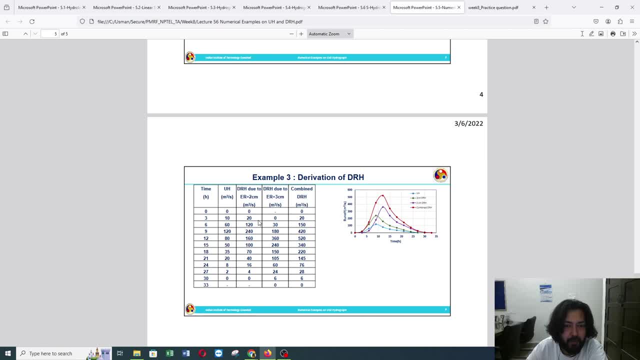 so the first value was 2: 0: 0 x 2 is 0, 10 x 2 is 20, 16 x 2 is 120, 120 x 240. now then they are saying is there is a time lag of 3 hours and we want to calculate drh due to excess. 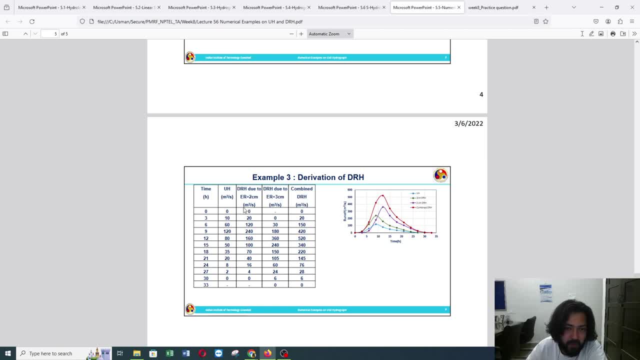 rainfall of 3 centimeter. so what we are going to do first, similarly, we are going to obtain another table of drh due to excess rainfall of 3 centimeter. it means we will get another column here which will give us the value of 0. then 10 x 3 is 30, 60 x 3 is 180, 120 x 360, 80 x 3 is. 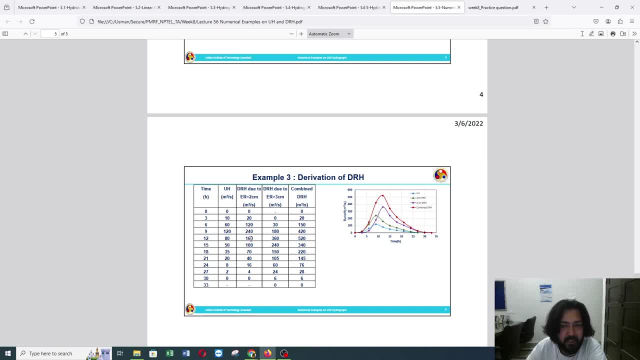 240, but since there is a time lag of 3 hours, we are going to shift it into 3 hour value. so that is the reason we have shifted here, because there is a time lag of 3 hours. so we have multiplied this column with 3, column second with 3 and then we have taken a time. 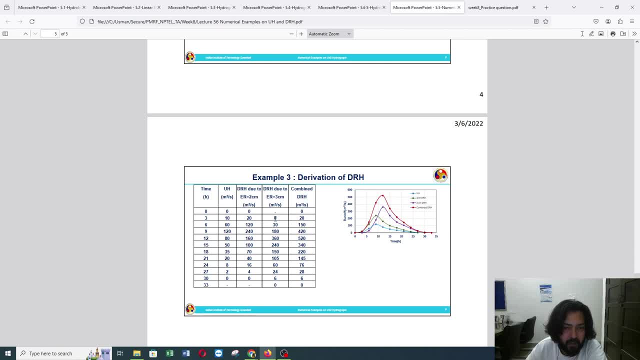 lag of 3 hours. so we have shifted it into 3 hours. so what we have done is that we have by 3 hour time lag. Now they have asked us to find a combined DRH. So combined DRH means we have to take apply principle of superposition. then it means we just need to add this value: 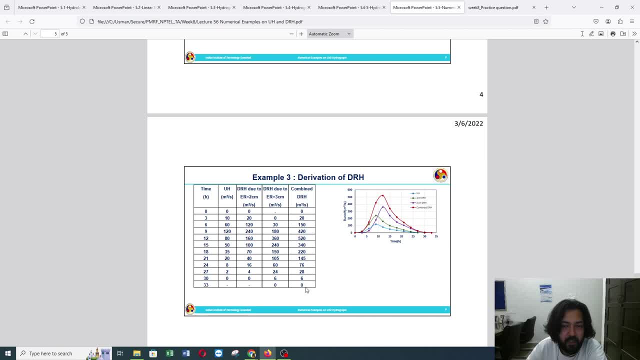 So 20 into plus 0,, 21,, 20 plus 30,, 150, and that is combined DRH. So here we have plotted first unit hydrograph for that same thing. we have plotted 2 hours, 2 centimeter DRH. then this: 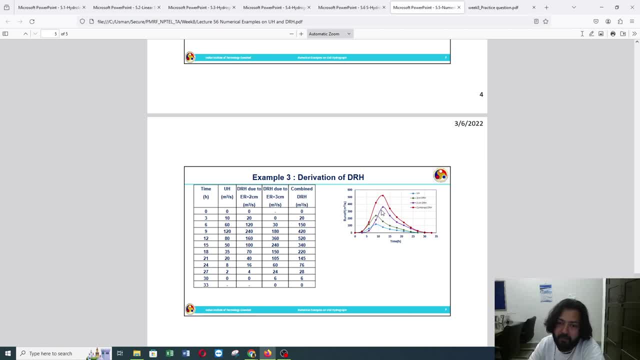 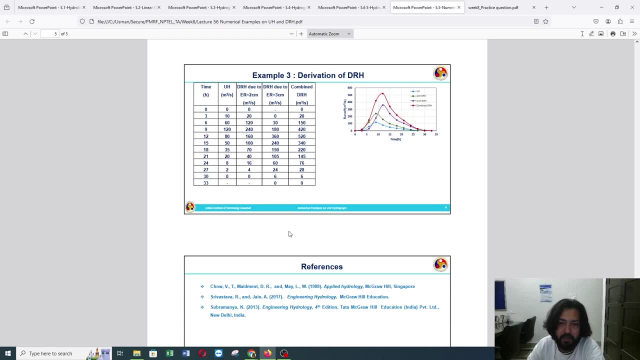 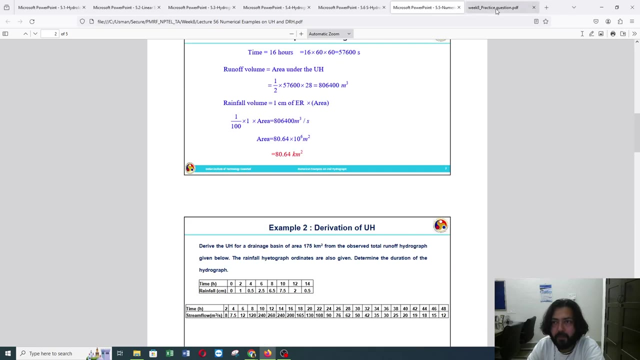 purple line shows 3 centimeter DRH which is having a time lag of 3 hours. So it has been shifted by 3 hours and the red curve indicates combined DRH. So this is also very simple problem. Now I have also given few problems which would help us to practice this kind of numericals. 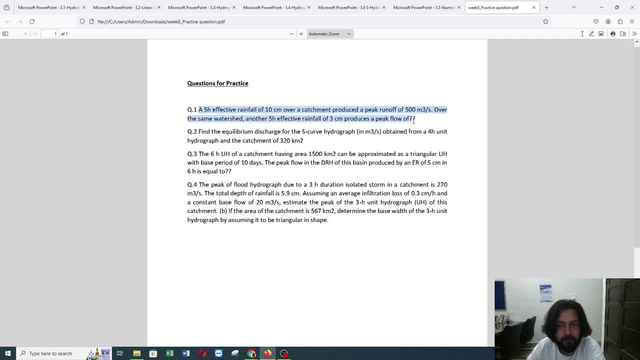 So first we will look into first problem. So here they are, saying an effective rainfall of 10 centimeter is occurring over a catchment. An effective rainfall of 10 centimeter over a catchment produces a peak runoff of 50 meter. 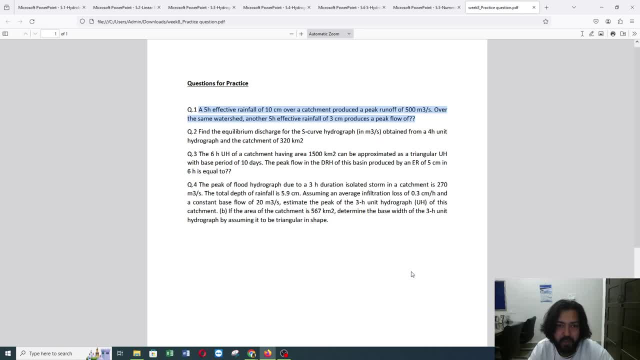 cube per second, 500 meter cube per second. Over the same watershed, another 5 hour. effective rainfall of 3 centimeter produces a peak flow of what? So they are saying that when the rainfall of 10 centimeter is occurring, the runoff is 500 meter cube. Now they are saying: 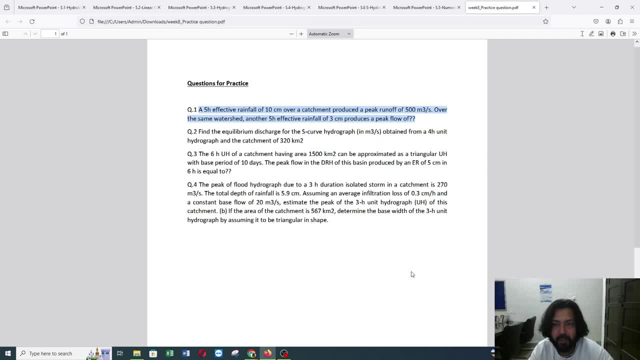 when the effective rainfall is reduced to 3 centimeter, what would be the peak flow? So we know that if the effective rainfall is reducing, it means the peak will also be reduced. So by logically we say that when 10 centimeter of rainfall was occurring, the peak flow was 500. So in 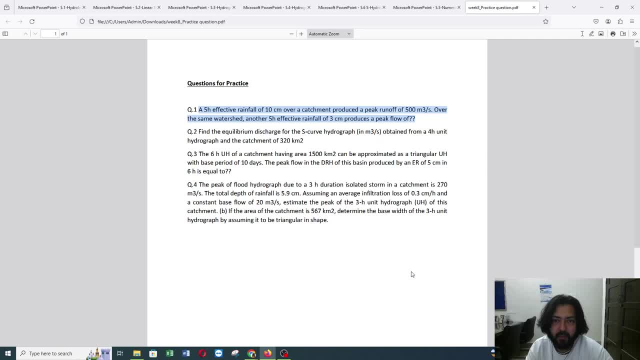 the same catchment for same effective rainfall duration, if 3 centimeter of rainfall is occurring, the peak flow would be less than 500 meter cube per second. So now let us calculate Now how we can calculate. that is So. they have given us effective rainfall here. that is effective rainfall is 10 centimeter. 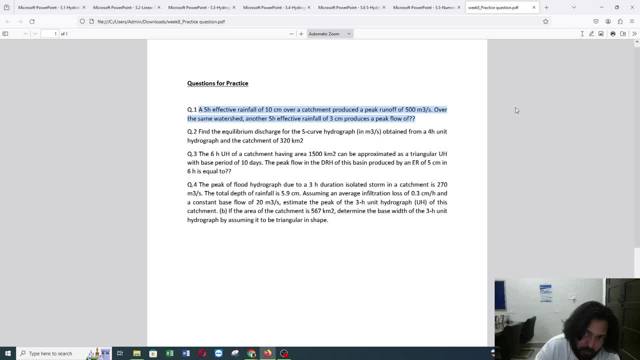 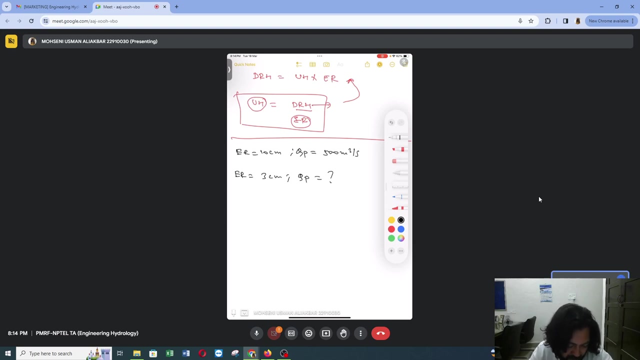 and also they have given us the value of peak flow as 500 meter cube per second. Then they are saying: when the effective rainfall reduces to 3 centimeter, what would be the peak flow Ready? Yes, Yes, Yes, Yes. So this is the condition that we have. they are saying that the effective rainfall is 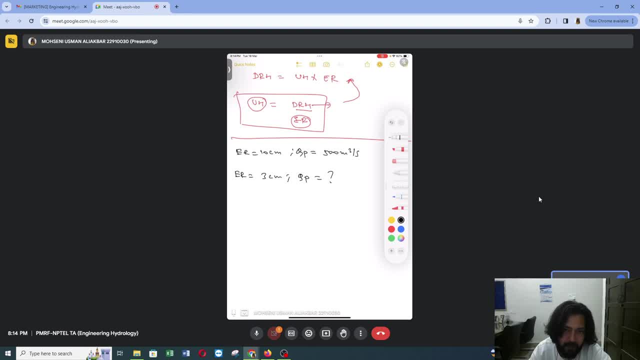 10 centimeter, which is occurring for 5 hour, and the peak discharge that was absorbed was 500 meter cube per second. Now, if the duration is same but the effective rainfall is reduced to 3 centimeter, what is the peak discharge? So, first, what we can do is we can calculate. 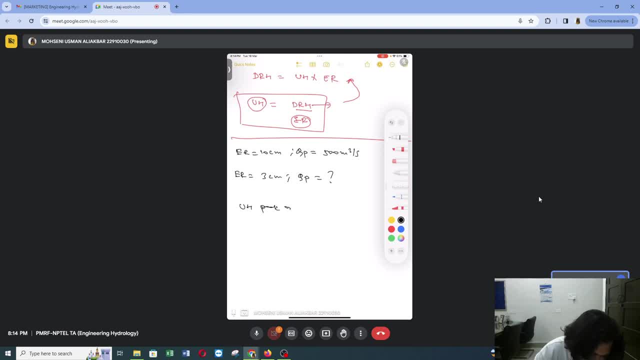 the unit R peak ordinate. So if we know the unit R peak ordinate, then we can just simply multiplied with the excess rainfall of 3 cm and we can get the peak discharge right, because the unit hydrograph peak coordinate will be same. so how we can do that, this is drh peak. 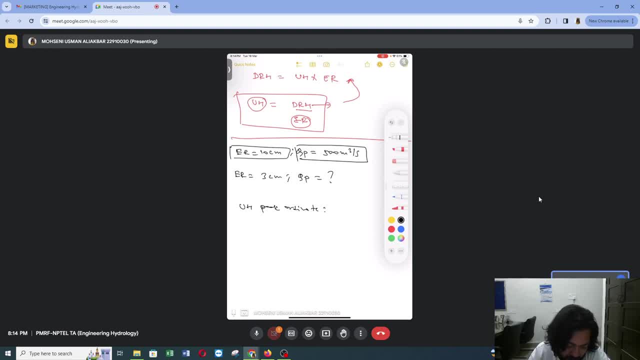 coordinate right, and this is excess rainfall. so we know the relation that uh is uh coordinate is nothing but drh coordinate divided by er. so we can simply divide this, 500 divided by 10, and we can get the value of 50. so the unit hydrograph peak coordinate is 50 mq per. 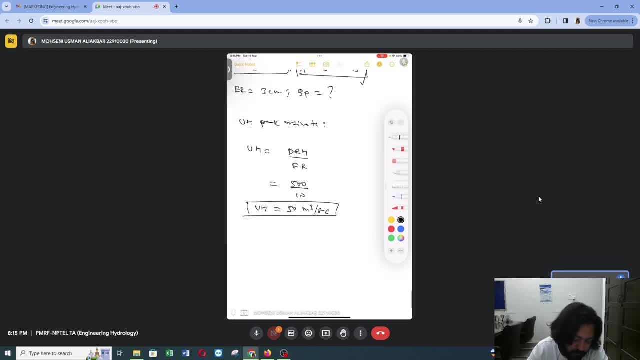 second now what we can do. we can use the same equation and we can calculate drh by changing er 3 and unit hydrograph as 50. right, so we can write: drh is equals to u another into er, so we know uh is 50 and effective rainfall that they have asked is 3, so we can. 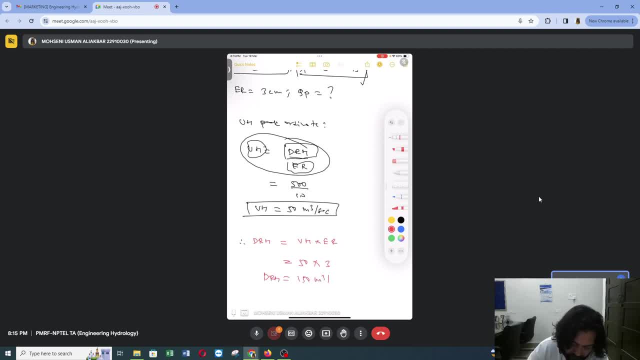 say that the drh is 150, right. so the important thing here to remember is that whenever the excess rainfall is reducing we can, we know that the drh will also reduce. so initially, when excess rainfall was 10 centimeter, drh was 200. but when excess rainfall get reduced, 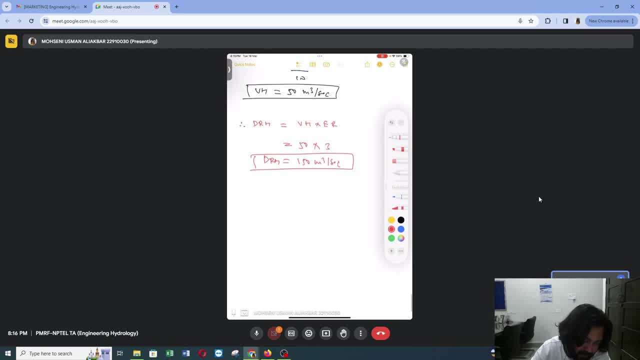 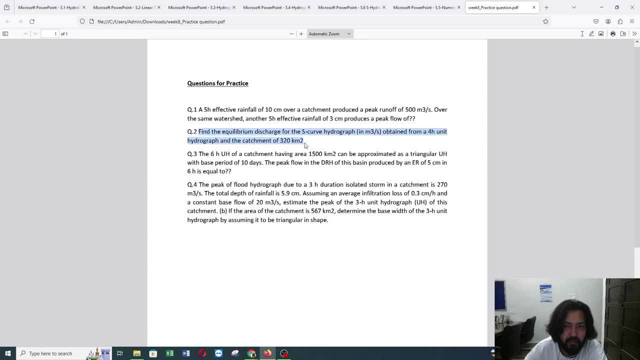 to 3. the drh also got reduced to 150. now let us see next equation. the next equation is based on s curve hydrograph. so they are asking us to find this equilibrium discharge for s curve hydrograph in meter cube per second, obtained from a 4 r unit hydrograph and the 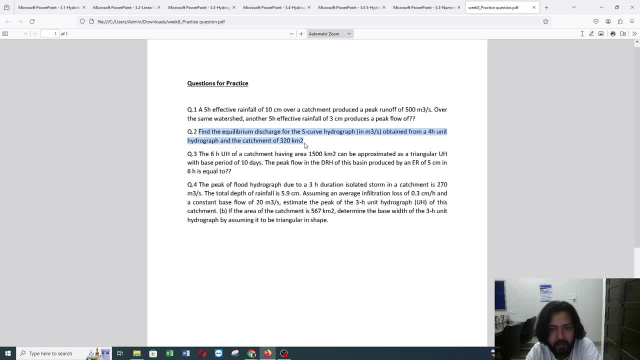 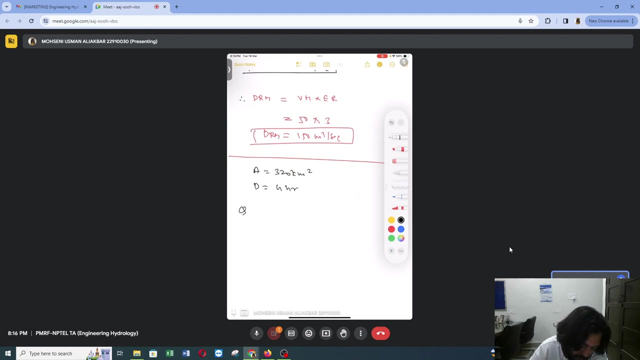 catchment of 320 kilometer per 320 kilometer square. so so, so, so. so, the area is 320 kilometer square and the time duration is 4 r, right? and they are asking us to calculate this equilibrium discharge. that is q equilibrium, right? so we know q equilibrium. 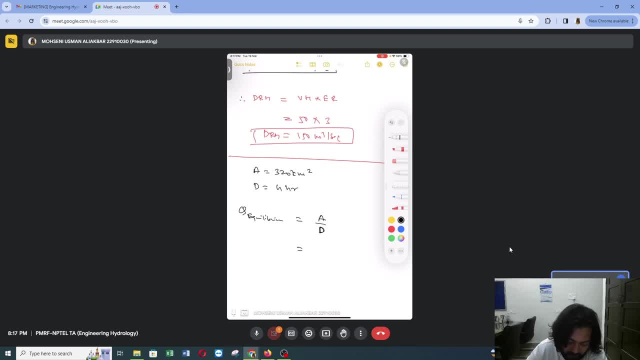 is nothing but a by d, right. but we need to convert area into meter square and r into second second. so area is 320, so we are going to convert it into meter square, right. so duration is 3 r. so we are going to convert 3 r into seconds. so it would be 4 r. so 4 into 60, into 60, right. 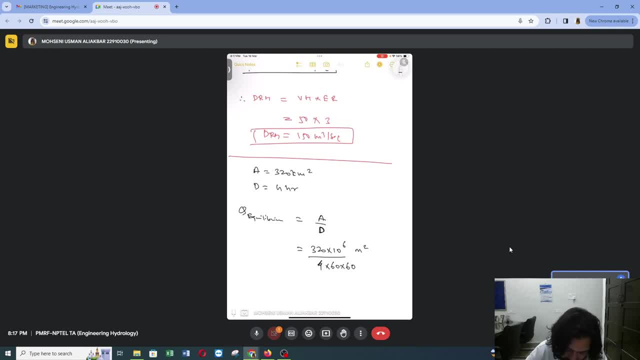 so right. so now we can solve this equation and we can get the value of q equilibrium. so this is also very simple problem. we just need to do the unit conversion and you can. you have to remember the q equilibrium. the next equation, the next equation we are going to do, is we: 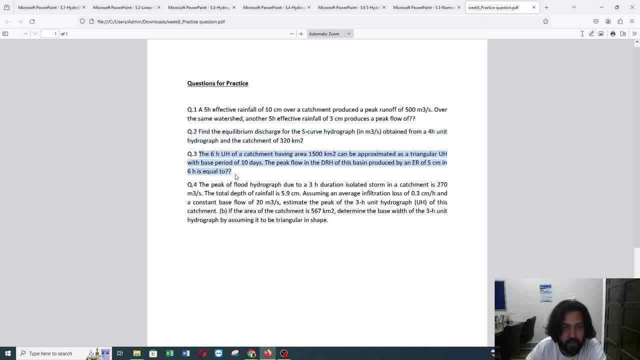 are going to do the unit conversion and you can. you have to remember the q equilibrium. the next equation, the next numerical is: they have given us 6 r unit hydrograph of a catchment having area 1500 kilometer square and it is approximately z as a triangular unit hydrograph. 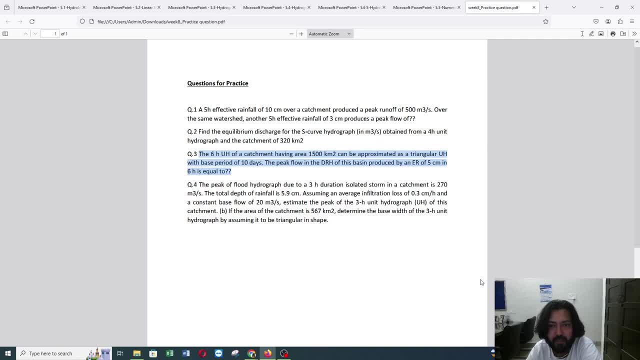 at the base period of 10 days, the peak flow in the drh of this basin is produced by er of 5 centimeter is equal to how much? so they are asking us to calculate the peak flow right, so how we can do that. so again, we need to remember that the air flow is equal to how. 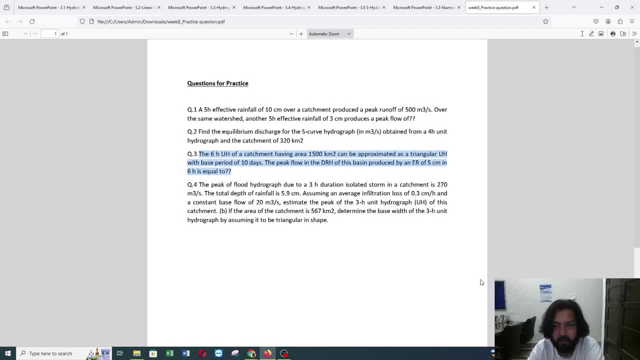 much. so here we are checking the peak flow right. so we can do it with the help of d r. remember the procedure: how to derive the drh right. so, firstly, what we are going to do is we are going to calculate the volume right. so volume is nothing but area under the curve. 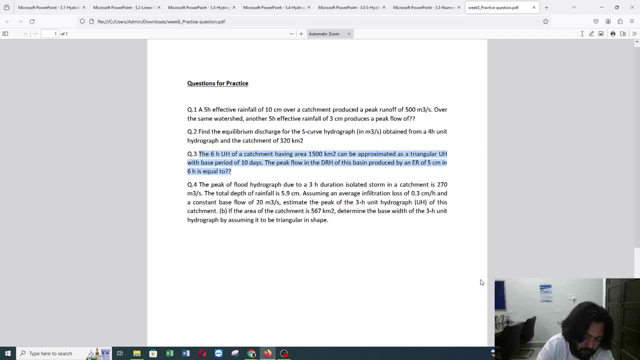 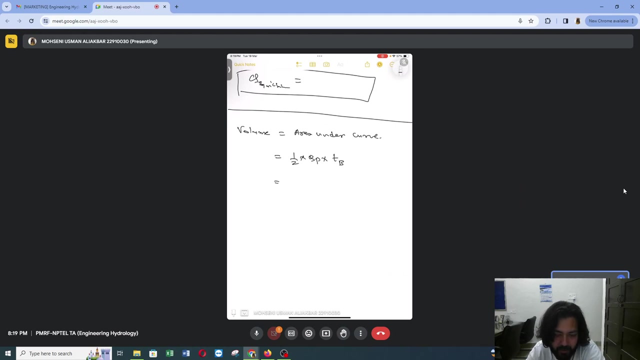 so area is nothing but half into qp into time of base, right? so volume is nothing but area under the curve and that area, they are said, is to be triangular. so for that triangular the base is tb and peak discharge is qp, right? So half into Qp is equal to time base. So the base time they have said is of 10 days. 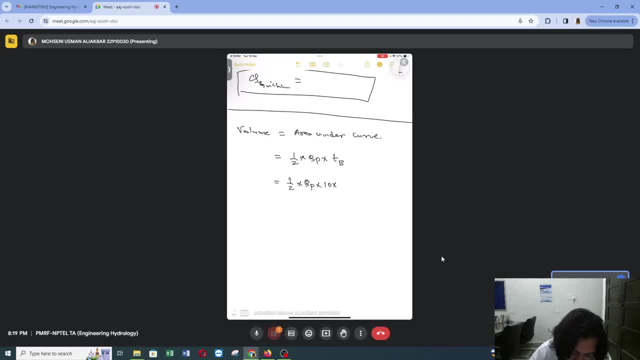 So 10 days means 10 into 24, into 60, into 60. So we are converting days into seconds. So this is the value of volume and we don't know the value of Qp. Now, this volume, if 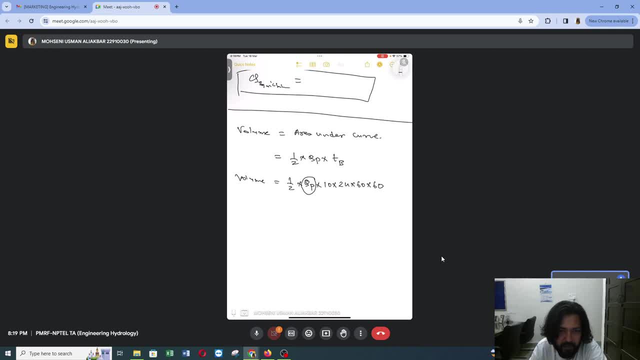 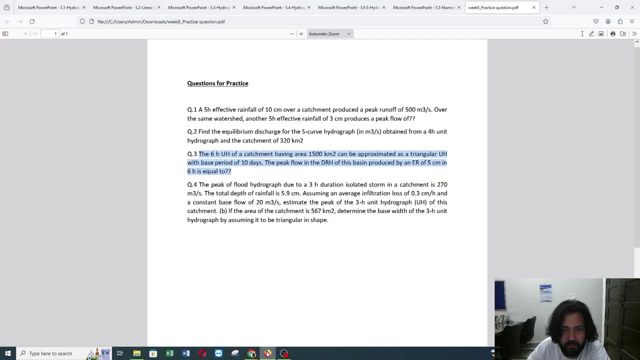 we derive this volume with the area of catchment, we will get the value of excess rainfall right. So we know excess rainfall. the depth of excess rainfall is equal to volume divided by catchment area. So excess rainfall that they have given us is 5 centimeter, right. 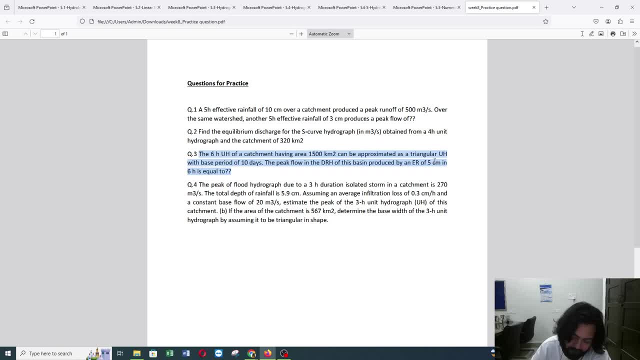 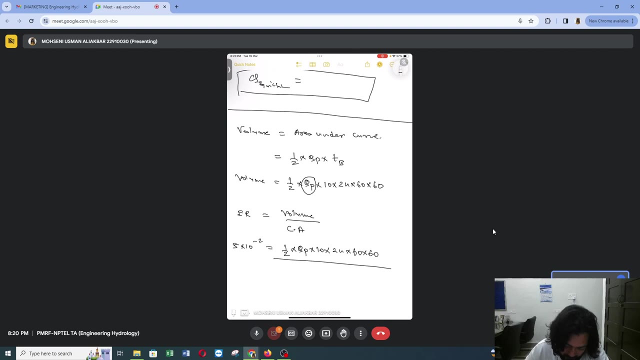 So 5 centimeter excess rainfall they have given, and volume is that we have calculated. Now the value of catchment is also known to us, catchment area, which is 1500 kilometer square. So we have converted into meter square. So if we solve this equation we will get: 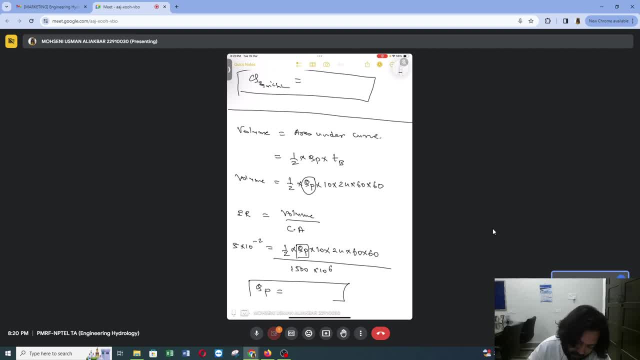 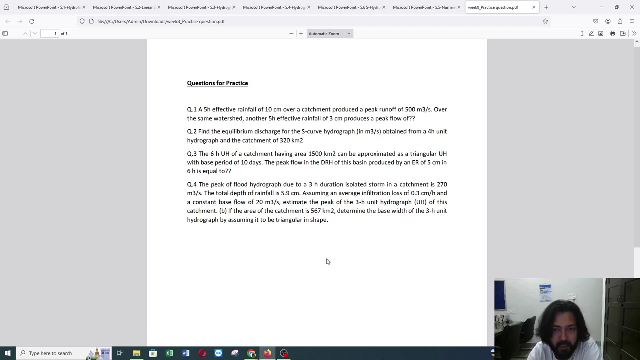 the value of Qp, which they have asked us to calculate, which will be meter cube per second. right Now let us see another problem, or the last problem. So here in this problem, they are saying that the peak of flood hydrograph, due to a 3 hour duration, is isolated storm in. 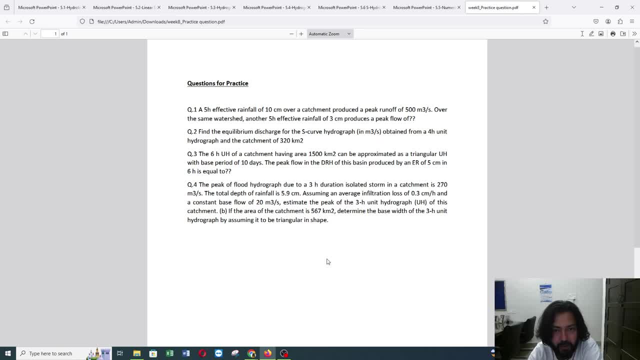 a catchment is 270 meter cube per second. So they have given the duration of storm and also they have mentioned the catchment area. They have also mentioned the peak of that storm, that is 270.. The total depth of rainfall is 5 centimeter, assuming an average. 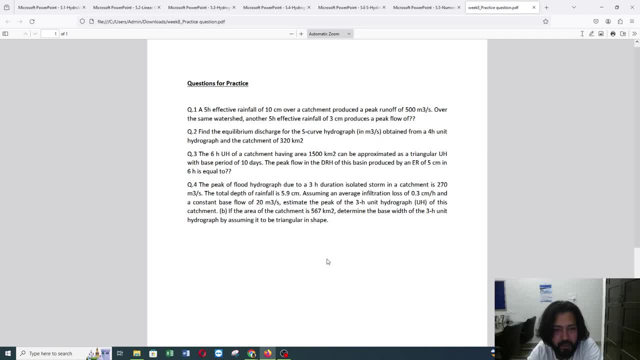 infiltration loss of 0.3 centimeter per second. So this is the peak of flood hydrograph, due to a 3 hour duration of 3 meter cube per second. So the first thing that they have asked is the first thing that is given to us is duration of rainfall. So the duration is known to. 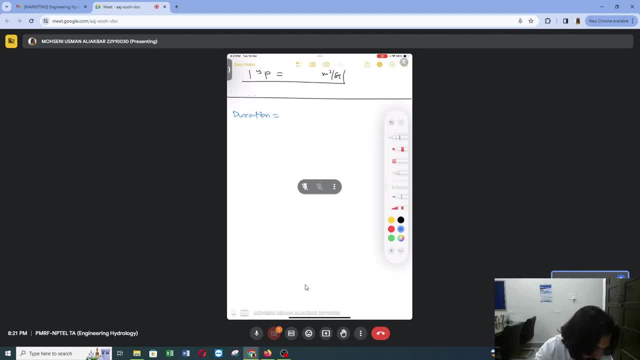 us, So that duration is 3 hour. right Then they have mentioned losses. So 3 hour is nothing but 0.3 centimeter per hour. So 0.3 centimeter per hour means we have hour of. 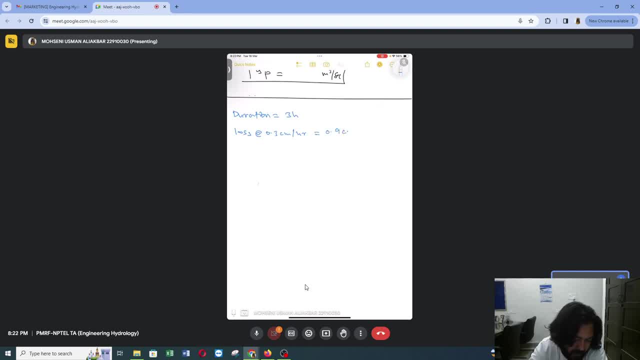 3 duration. So the losses would be a count of 0.9 centimeter. For 1 hour the losses is of 0.3 centimeter. So for 3 hour it would be 0.3 into 3, which is 0.9 centimeter. Then 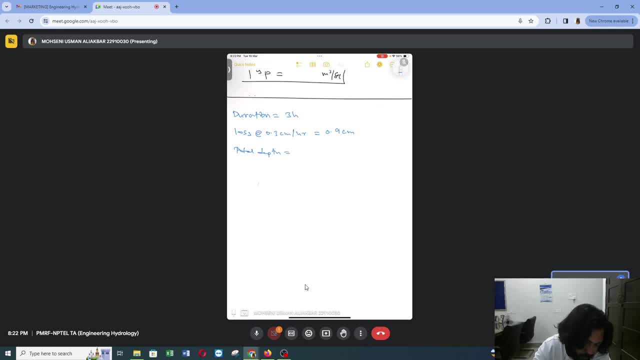 they have mentioned us is total depth, So the total depth is 5.9.. But what we need is we need excess rainfall, right? So what is excess rainfall? Excess rainfall is nothing but the total depth of rainfall minus the losses. So total depth of rainfall is 5.9, minus losses is 5 centimeter. So the 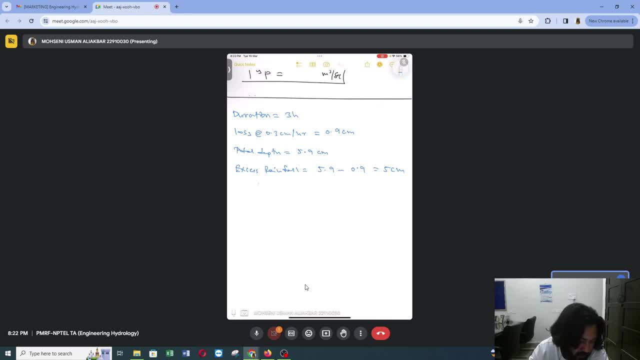 value of excess rainfall for that storm duration of 3 hour is 5 centimeter. Also they have given us is the peak flow of hydrograph. that is 270 meter cube per second right. So this is the peak flow of hydrograph. So this is the peak flow of hydrograph. So this is the. 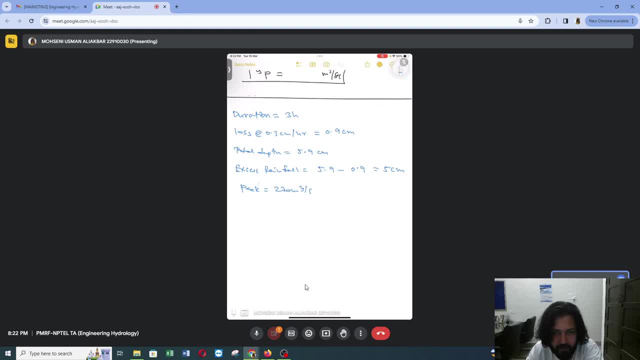 peak flow of hydrograph. But we need the peak of DRH. So how we can calculate the peak of DRH, They have given us the base flow value. So base flow is 20 meter cube per second. So if we separate the base flow from the value of storm hydrograph we can get the value. 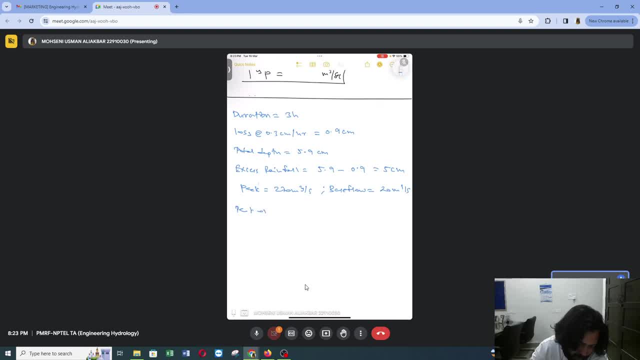 of direct turn of hydrograph. So the value of peak of DRH would be 270 minus 20, which will be 250 meter cube per second. Now in the equation they are asking us is to find the peak of 3R unit hydrograph right. 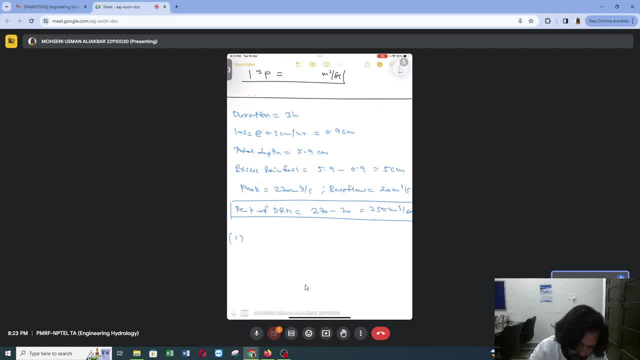 So the first thing that they have asked is to calculate. the first thing they have asked is to calculate peak of unit hydrograph, right, And the second thing that they have asked is to find base of 3R unit hydrograph. So these are the two unknowns that they have asked us to calculate. 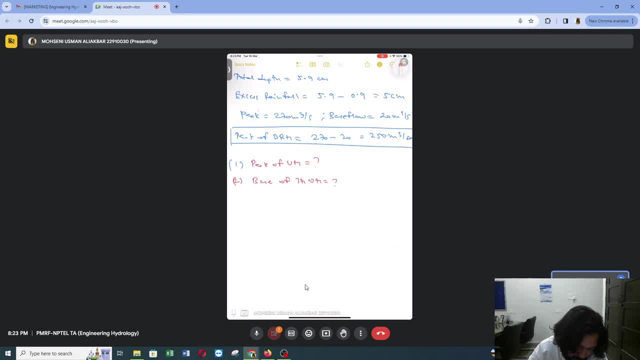 So how we can do that? We know this relation. In order to calculate ordinate of UH, that is, unit hydrograph, we need to divide the ordinate of DRH with respect to excess rainfall, right? So here we are required to calculate peak of unit hydrograph. 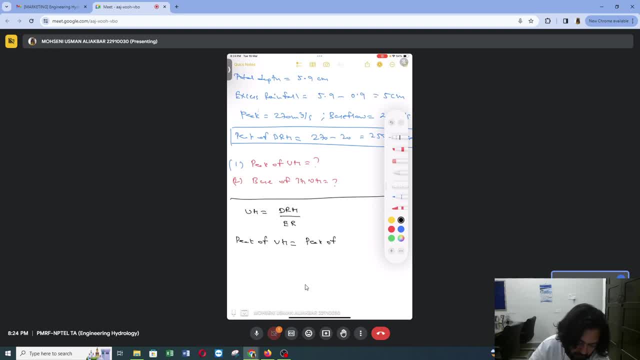 And we know the value of peak of DRH And also we know the value of excess rainfall. So what we are going to do is we are just going to divide peak of DRH with excess rainfall. So peak of DRH is 250, excess rainfall is 5.. 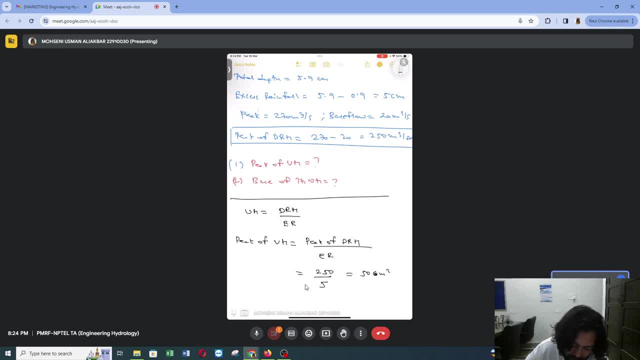 It means peak of unit hydrograph would be 50 meter cube per second. So this is the first unknown that they have asked. Now the second unknown that they have asked is to calculate the width. So in order to calculate the width, we need to calculate the. 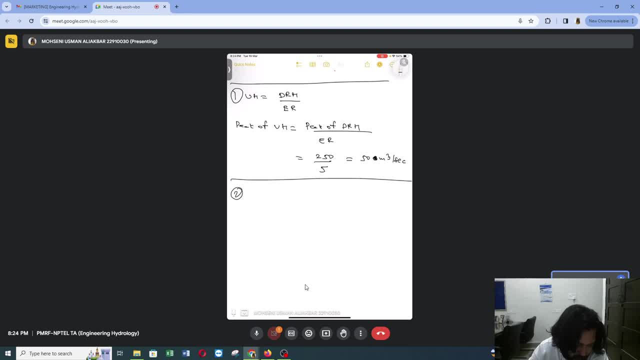 volume, right? So first we will calculate the volume. So we know this: that excess rainfall of unit hydrograph is equals to volume of unit hydrograph divided by catchment area, right? So excess rainfall of unit hydrograph is nothing but 1 centimeter. 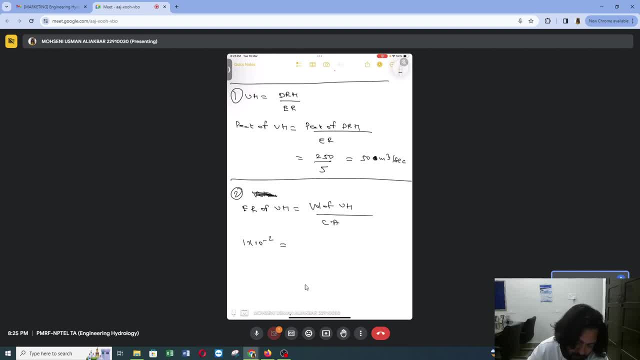 That is, 1 to the power of 10 to the power of 10.. So that times theytes to the power of minus 2.. We want to calculate the volume of unit hydrograph, So that volume of unit hydrograph is nothing but half into peak of unit hydrograph, which. 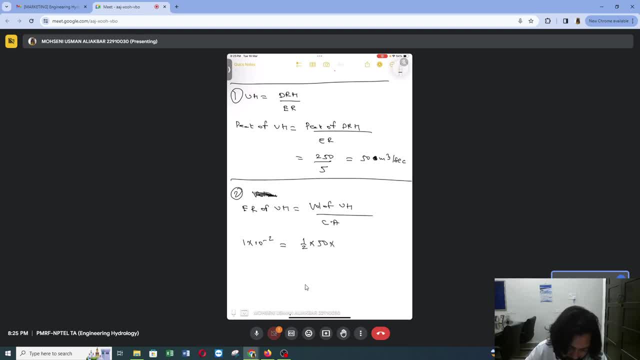 is 50 into base. So base is unknown to us, but it would be in hours, So we are going to convert that into seconds. So this is the unknown term and then also given as the catchment area. So the catchment area that they have given is 567 kilometers square. 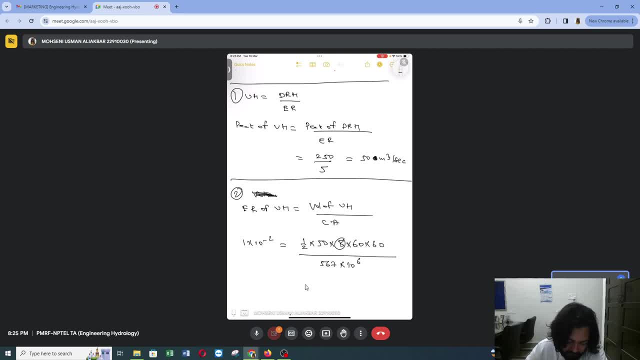 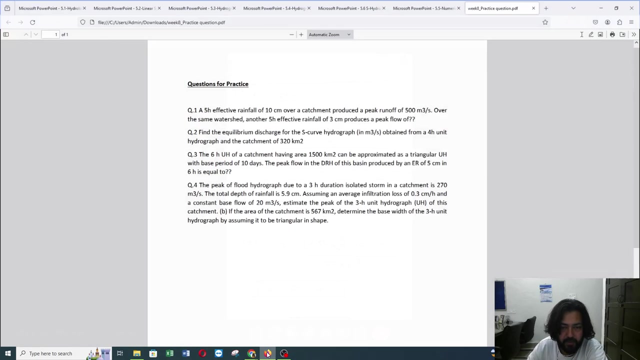 So we have convert that into meters, square right. So if we solve this equation now, we will get the value of time base, that is, it would be 63 hours. So these are like the few examples that can help us to solve numerical based. 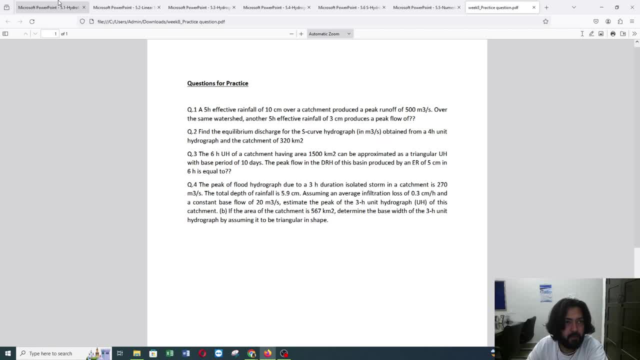 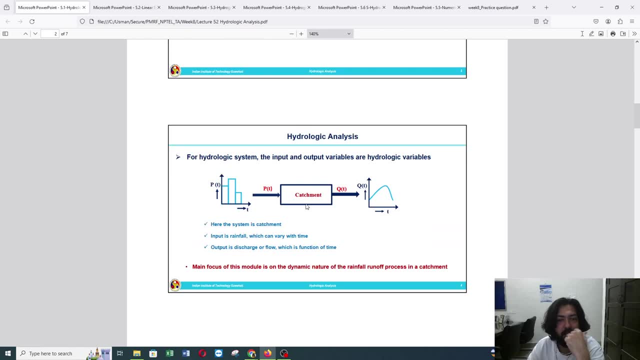 on this concept, right? So in today's class we started talking about hydrological hydrologic analysis. So we talk about, like, what is the hydrological system? So any system that consists of input and output variables as hydrological variables are called as hydrological. 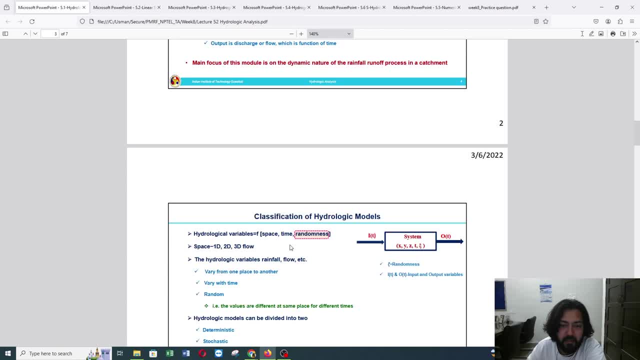 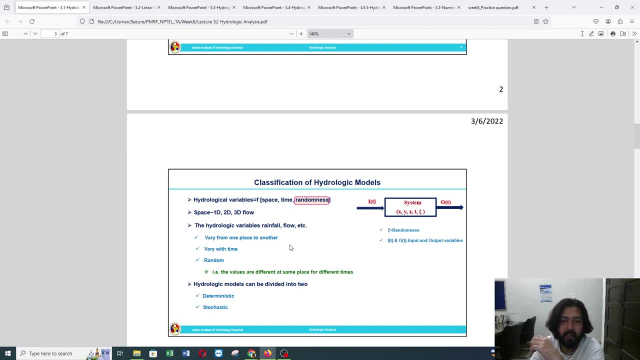 system right and we know that this hydrological system is a linear system. Then we also talk about different classification of hydrological model. So hydrological models are based, or classified, based on the functions, three functions. The first is function of space, function of time and randomness. So when we account for randomness, so based on the 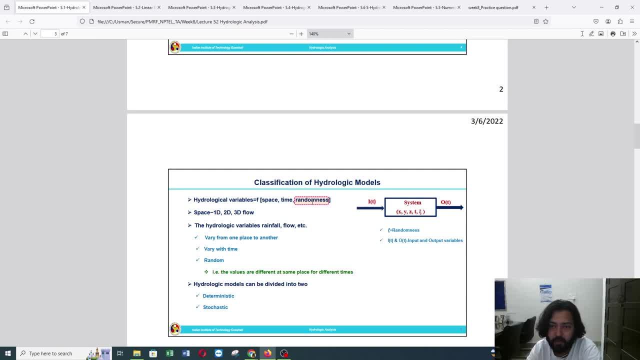 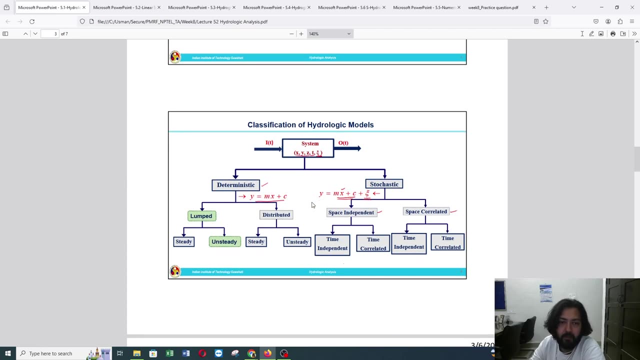 function of randomness. a model could be domestic or non domestic. So we talk about those models which are considered, and so that ignores uncertainty and the stochastic models are those that consider uncertainty. right, Then we have divided the model based on function of space. So, based on the function of space, model could be lumped model or distributed. 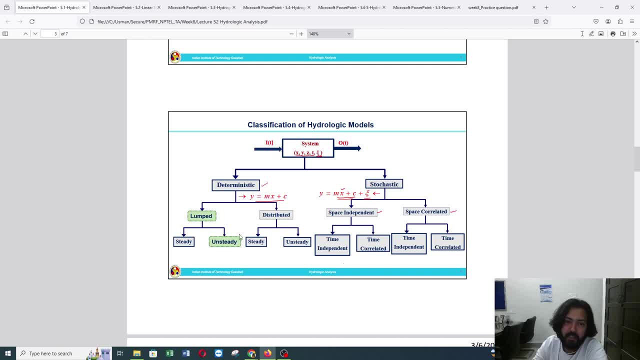 model, right. So lumped model are those model which ignores special variation. distributed model are those that accounts special variation. Then, based on the function of space model, time, a model could be steady or unsteady. steady knows variation with time, unsteady varies with time, right. so we have studied the different classification of hydrological model also. 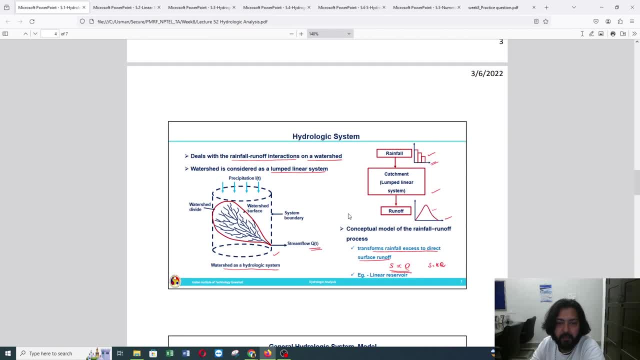 then we talked about hydrological system, right? so if you look at this figure, the red color pointed the shows the watershed divide, that is the watershed boundary. then this surface are nothing but watershed surface, then this boundary is the system boundary that we have considered. then the input is the precipitation and the output is the stream flow. so from this function, 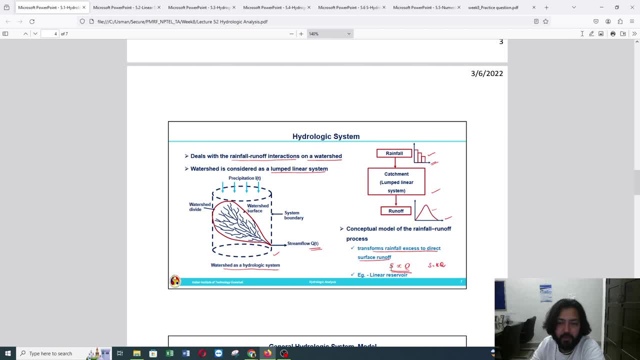 we can say that the output is a function of storage. right, so we know that storage is directly proportional to the output. so storage is equals to k times of q. so this type of approach is nothing, but it is example of linear reservoir. so then we started talking about more of linear reservoir. 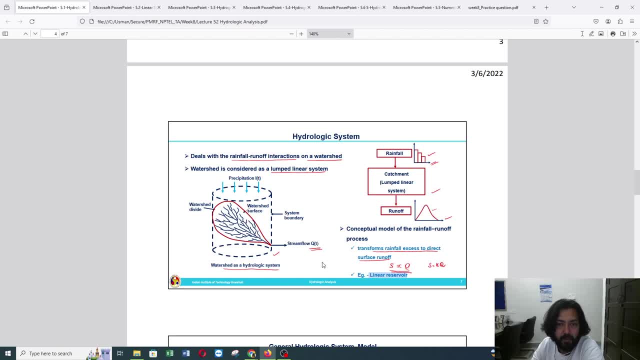 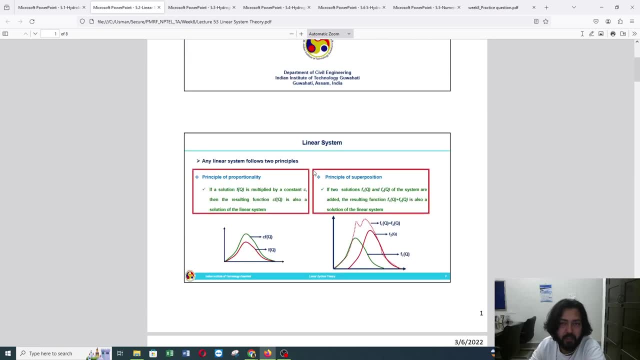 then we talked about the transfer function. so the transfer function could be a constant transfer function or it could be a differential transfer function. then we talked about more on linear system. so linear system are based on two, two principle, that is, principle of proportionality, where what we do is we just multiply the solution with a constant value, and that 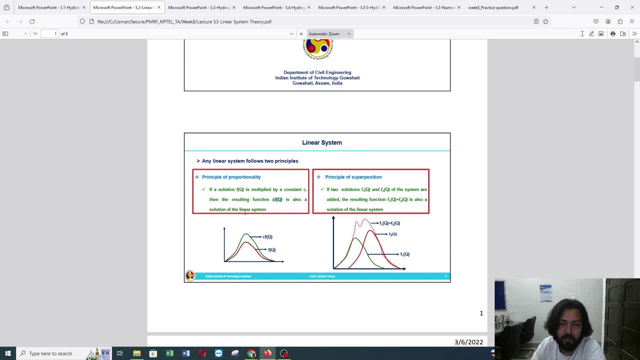 that value is also a solution to a solution of the linear system. it means a linear of principle of proportionality. we just multiply the result with a constant value in principle of superposition. let us say, if there are two output with us right, f1 of q and f2 of q. so if we 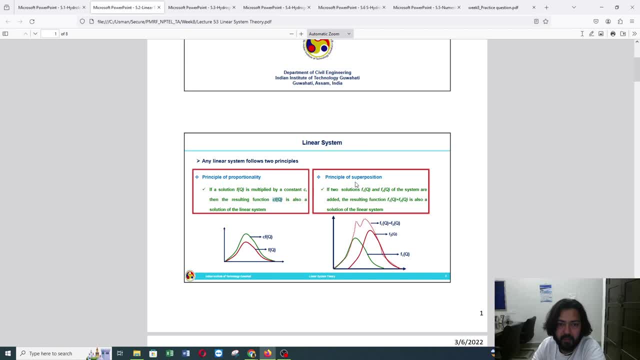 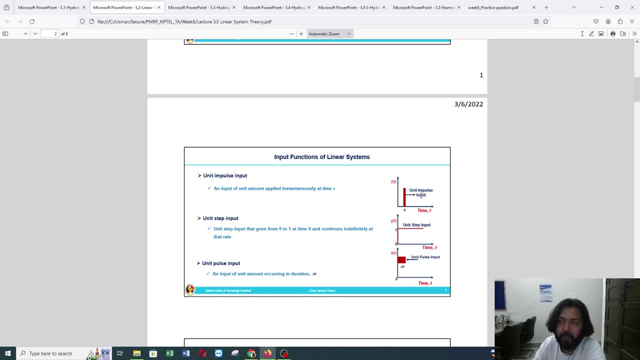 just multiply that method. there are only's two celestial Outputs: the food of producto, the output of theinges systems. there will be an output which is also the solution of the system. so these are the two principle of linear system. then we talked about the Matrix function of the linear system. so the input function could be of three types. it could 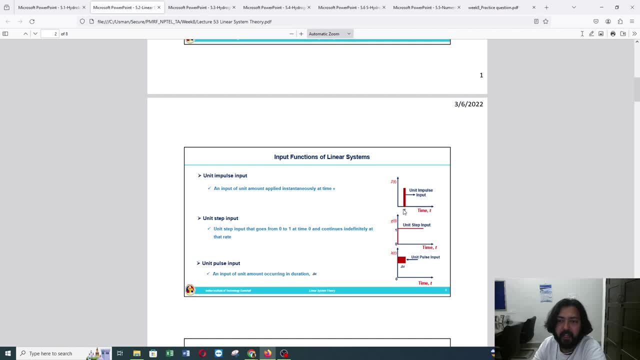 be a unit impulse which is applied instantly at any time. At 다음, there is unit step function which varies from zero to one. when at time equals to zero, then it remains constant over the period of time. this is called as unit step, and then there is unit pulse, so unit 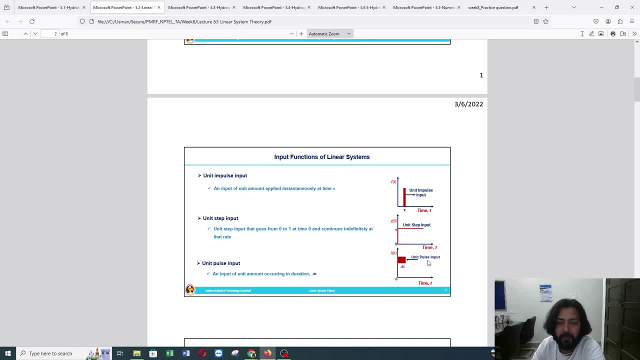 pulse is nothing but it is an input of unit amount which is occurring over and different times, yousn't see any difference or any other variation � tom 00001 lo for each unit and a constant time so that is function of linear system or the 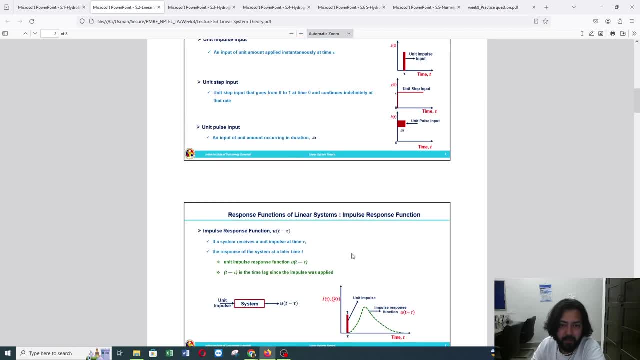 input function of linear system. then we connect this function with Nt. for a new function it could be defined period of time, that is, delta t. then we talked about the response function of linear system. so, considering the case of impulse input, we have derived a generalized equation which is: 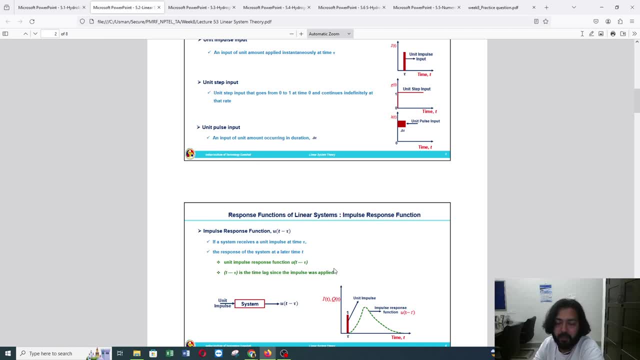 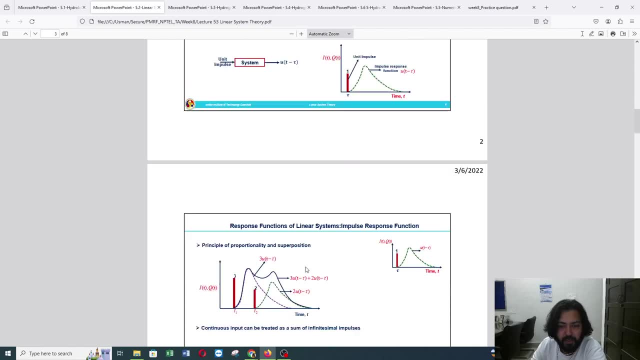 known as convolution integral, and based on them, though of the based on the convolution integral, we have derived the response function for unit step and unit pulse as well. right, so we have derived this equation of convolution integral, which is this equation: qt is equals to 0 to t. 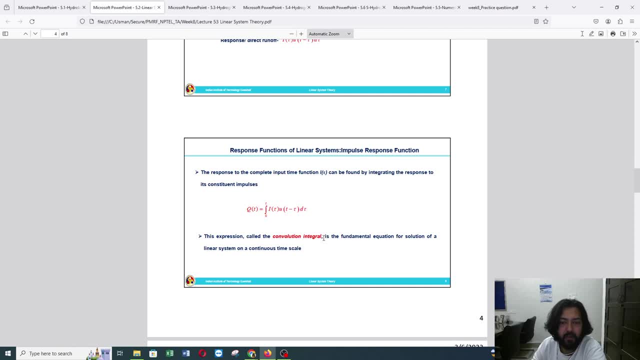 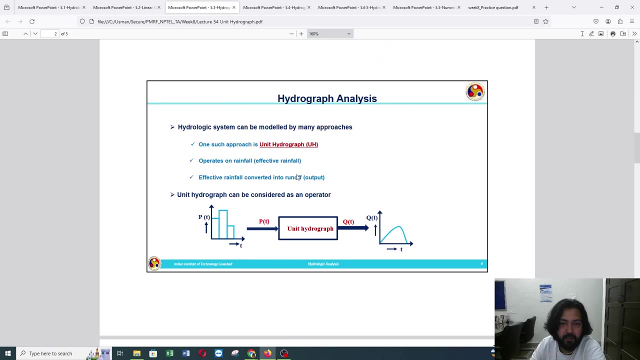 i times of tau ut minus tau dt. so this is convolution integral. so we can use this same equation for unit step response function as well as for pulse impulse response function. then we talked about unit hydrograph. right, so we talked about the unit hydrograph, which is nothing, but it is resulting from one centimeter. 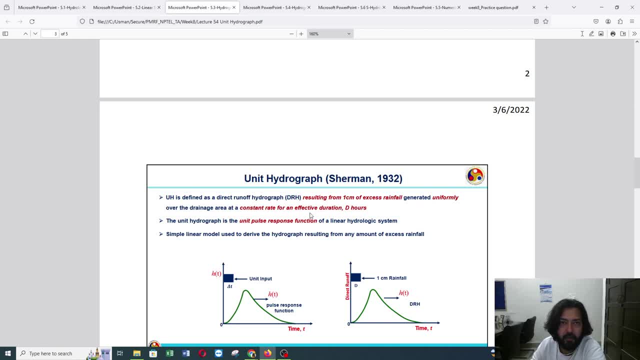 of excess rainfall which is generated uniformly over the interior at a constant rate for an effective duration of dr. so we know that the unit hydrograph is nothing, but it is a unit pulse response function of linear hydrologic system. so this is nothing but a representation of unit pulse response function where unit input is a unit. 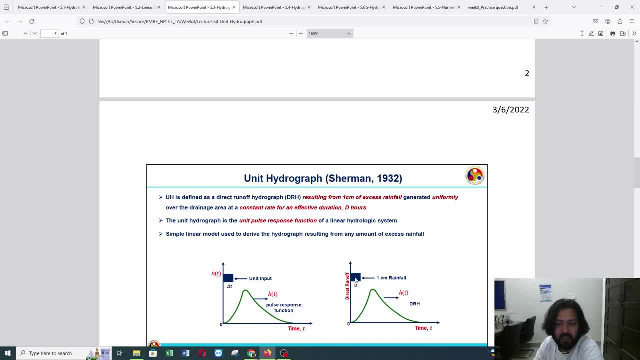 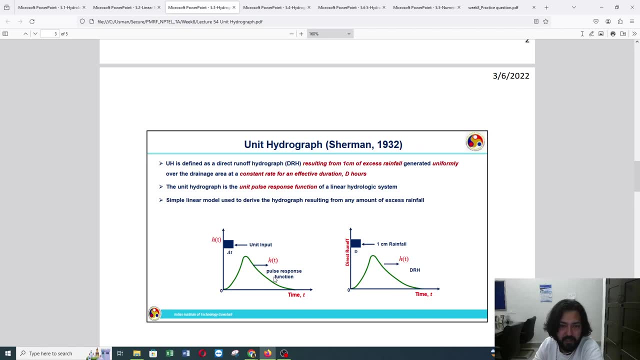 pulse and output is nothing but a pulse response function of ht. similarly, this is applied to unit hydrograph where input is er, that is, excess rainfall, and output is nothing but drh. right, then we have under. then we have talked about assumptions in hydrograph, that is, it is linear. 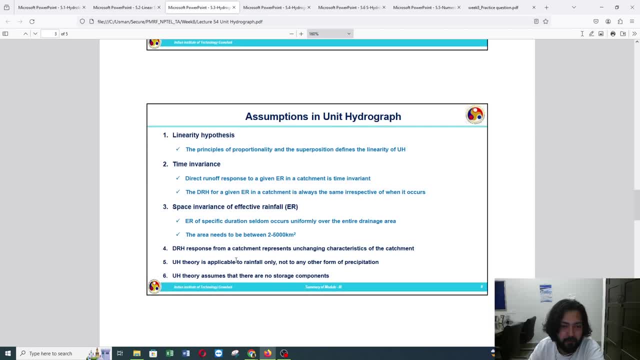 it is time invariance, then excessive rainfall remains constant over the period of time, then the area of catchment should be between two to five thousand kilometer per square. then we talked about that. the drh, response from catchment represent unchanging characteristics of the catchment. so we should 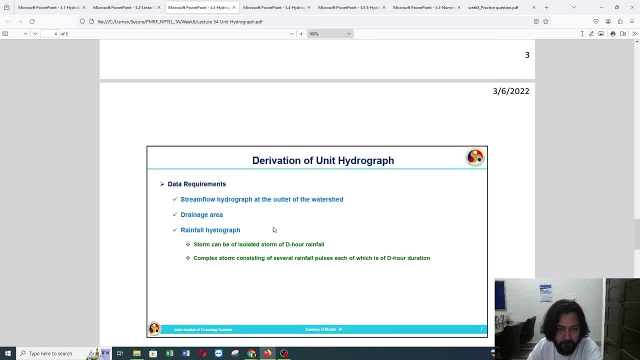 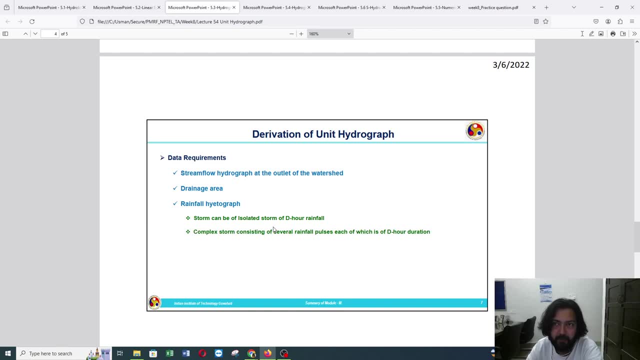 consider the changing characteristics. and then we have to derive the drh. then we looked into the procedure like how to derive unit hydrograph. so there are certain step. the first step is to separate the base flow. once we have separated the base flow, you get the value. 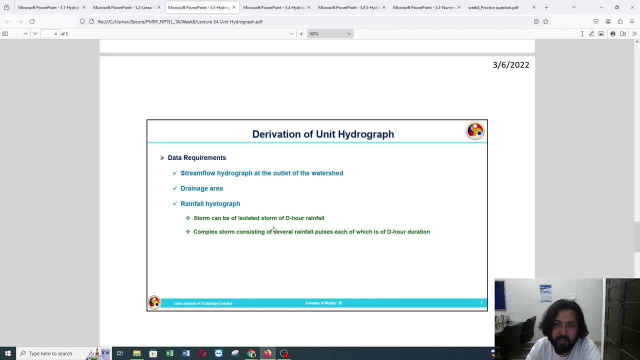 of drh, then you can calculate the volume of drh by taking the area under the curve, and then you can calculate the depth of excessive rainfall by dividing the volume of drh divided by the catchment of area. and then you can calculate the ordinate of unit hydrograph by dividing. 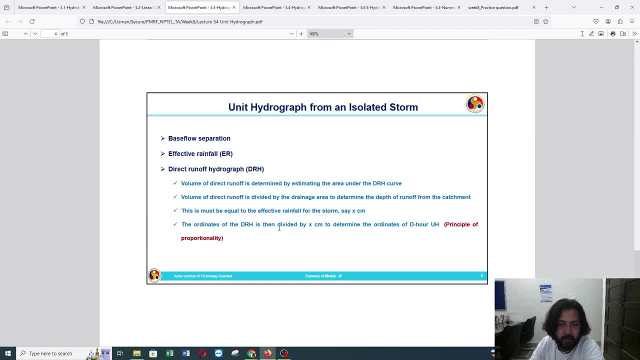 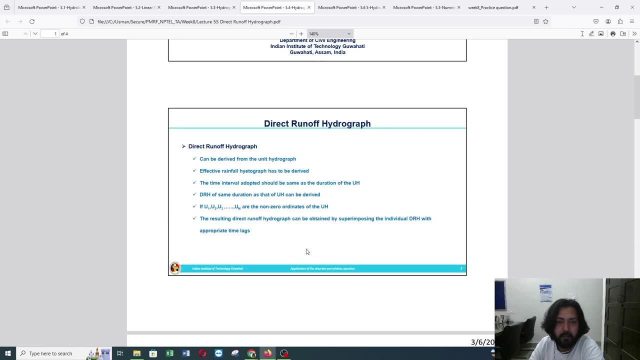 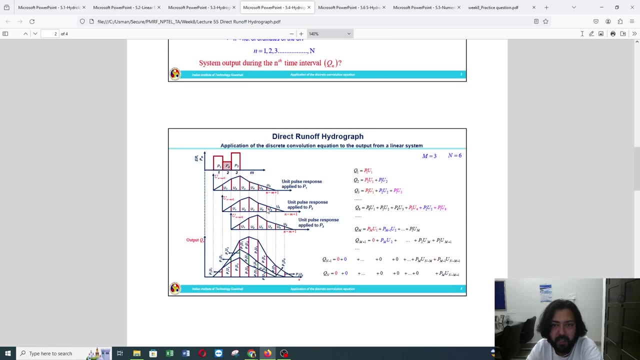 the ordinate of drh with respect to the, with respect to the excess rainfall depth. right now we have. we have also looked into this thing. like this is nothing but a representation, but it is how we can derive the drh from multiple storm events right, so we have also looked. 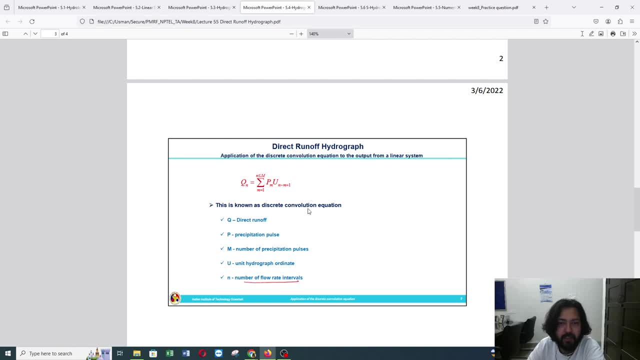 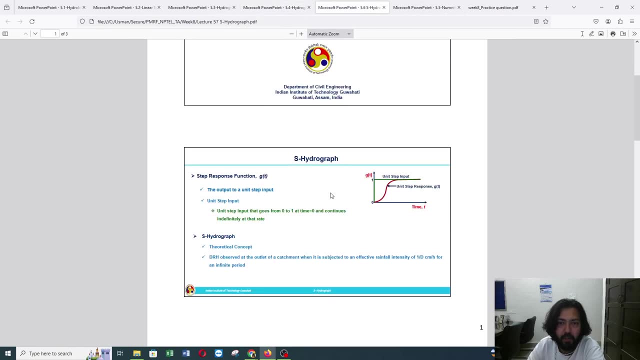 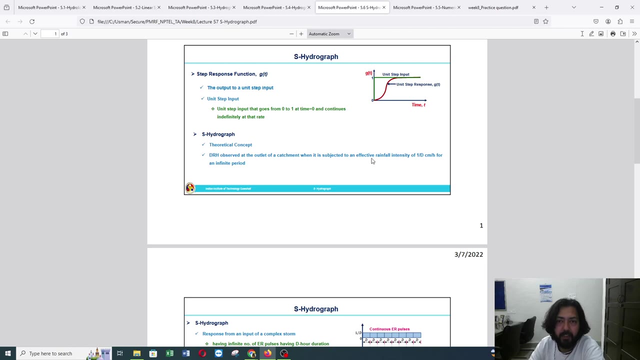 into a standard equation, this equation, which is known as discrete convolution equation. this equation can be used to derive the output when there are multiple storm events. right then, we talked about s hydrograph. s hydrograph is nothing but when, when drh is observed at the outlet of a catchment, when it is subjected to effective rainfall intensity of 1 by d. 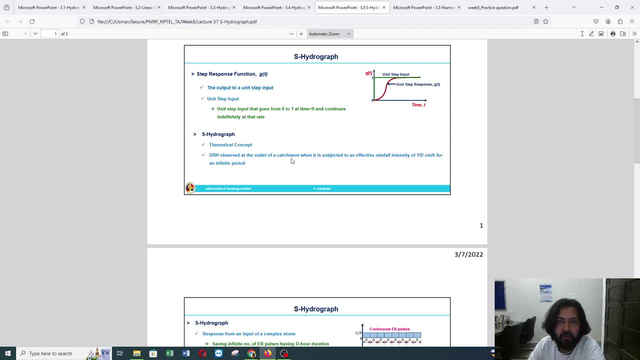 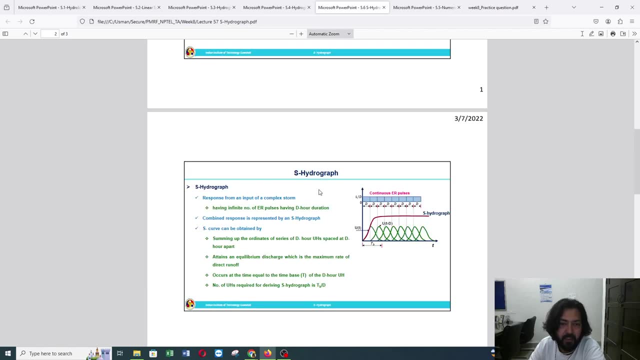 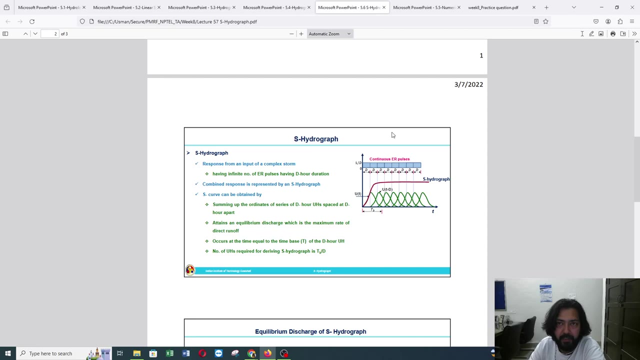 centimeter per hour for an effective period, right? so similarly as unit hydrograph is based on unit impulse, unit pulse response function, s hydrograph is based on unit step response function. right? so we have also talked about how s hydrograph is plotted and how it can be obtained. then we talked about various numerical 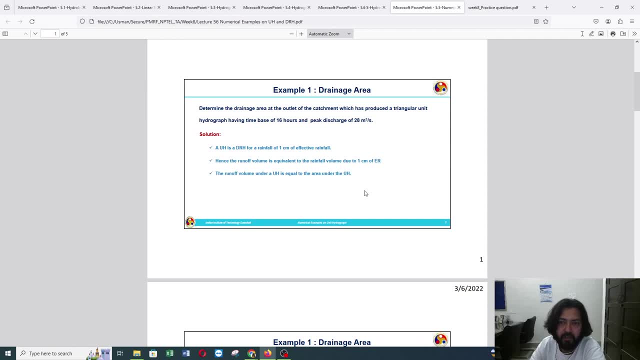 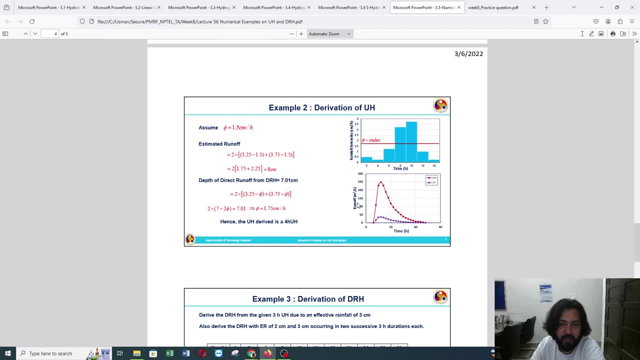 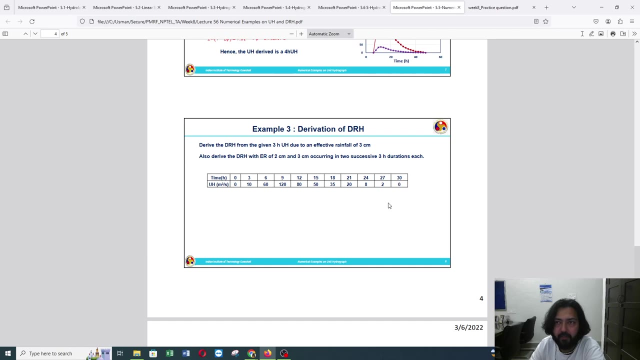 the first numerical was simply based on to calculate the drainage area of a catchment. then we saw, like how we can derive unit hydrograph. then we also saw numerical based on derivation of drh, like how to derive a drh when we have the value of unit hydrograph. and then we have 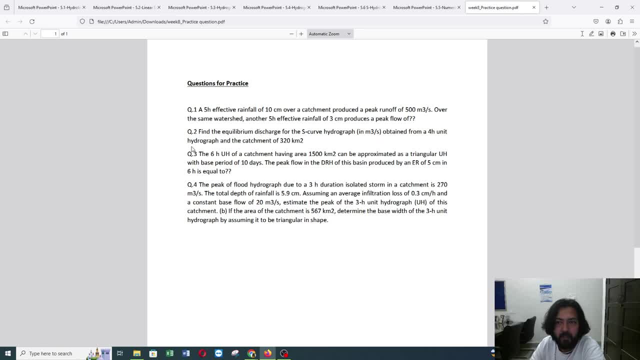 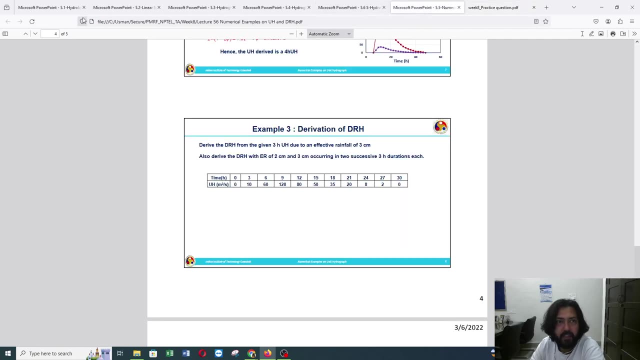 solved five, four different example where we, where we have also taken an example based on equilibrium discharge for s curve obtained from a 4 r unit hydrograph. so we know how can we can calculate the equilibrium discharge right. so we have taken like we have covered everything. so in the next class i think we will talk more about different hydrographs. 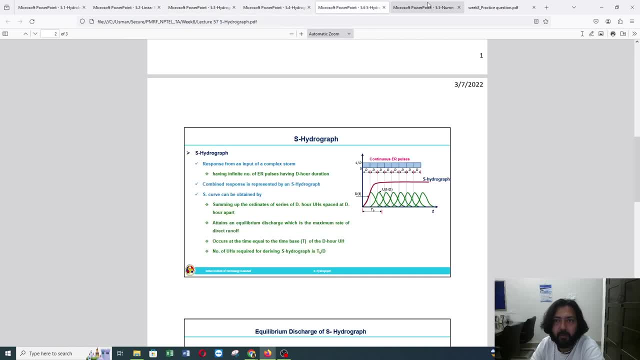 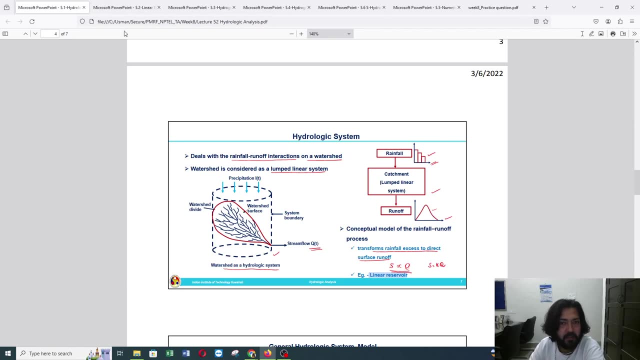 that are available. that will, that is, we will talk more about. Thank you. We will talk about synthetic unit hydrograph. we will talk about instantaneous hydrograph. so this is so far for today's class. so we have started with a new module which is called. 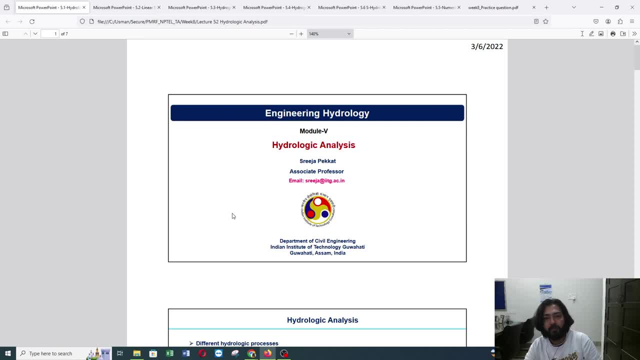 as hydrologic analysis, which is module five. so the same module will be again- will be covering in next week session, that is, week nine. again we will talk about more into hydrological analysis and then in the next, coming next to next, session we will start with another. 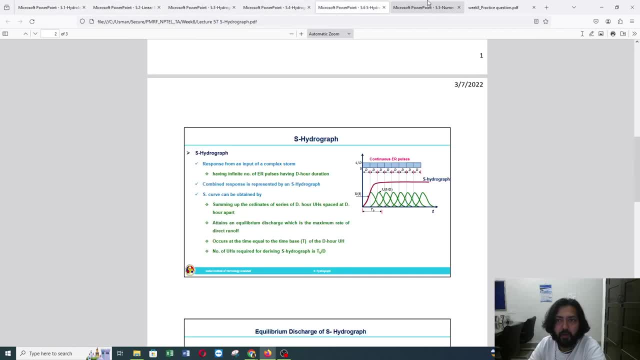 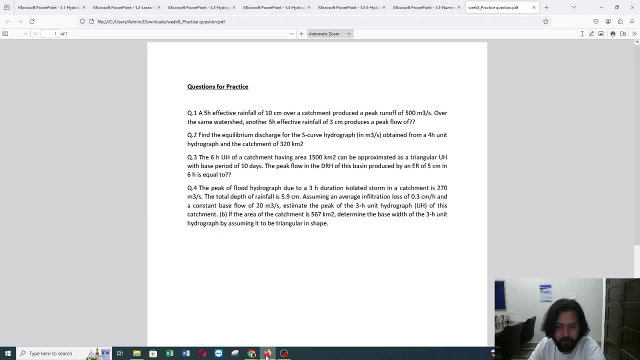 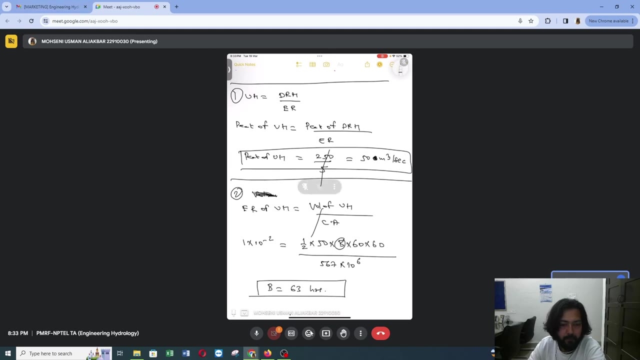 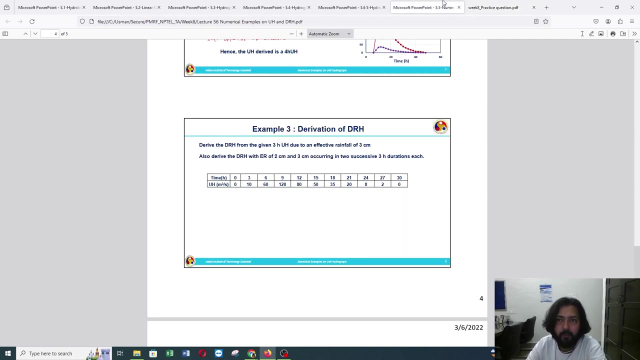 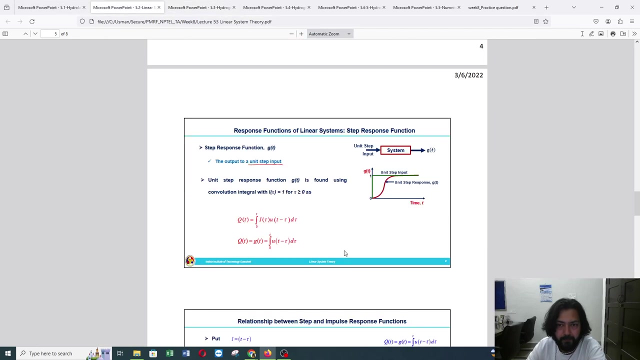 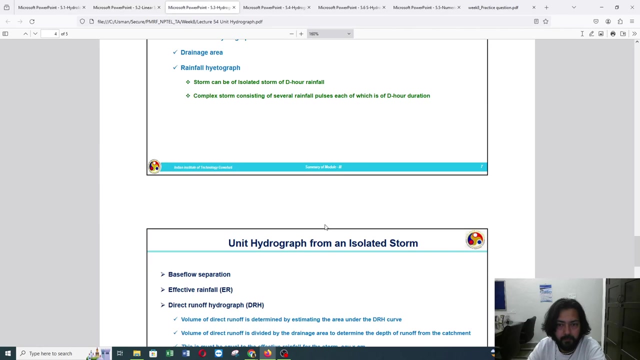 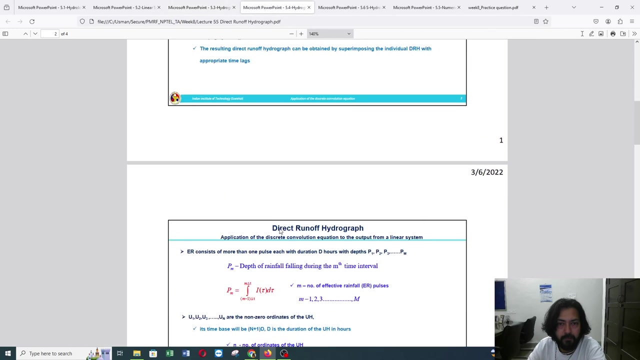 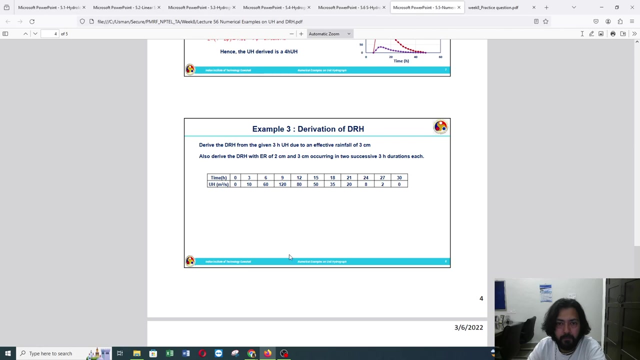 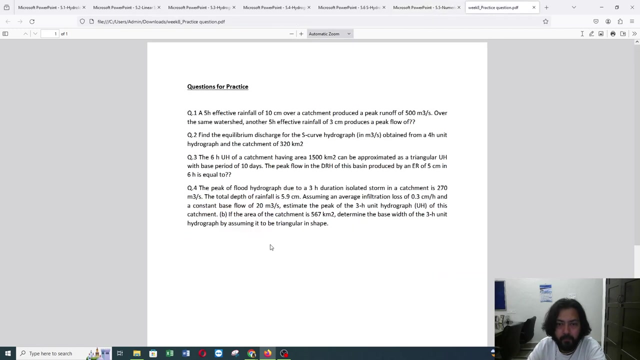